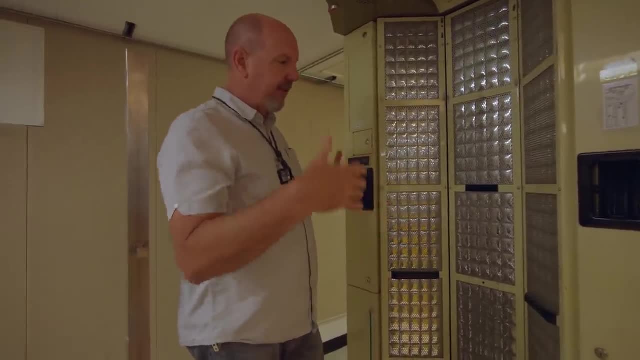 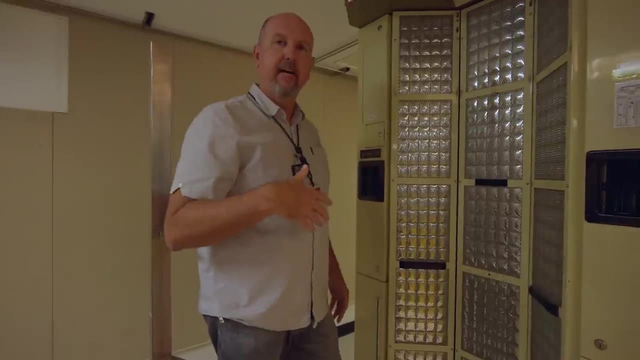 contamination. And so basically, I'll step in and show you it. It'll do a whole body scan on both sides. It'll do a 15 second scan, then i'll rotate and it'll do another 15 second scan on the back side and then, if i pass, it'll. 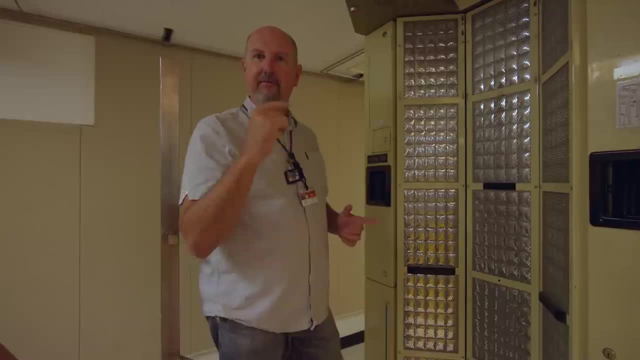 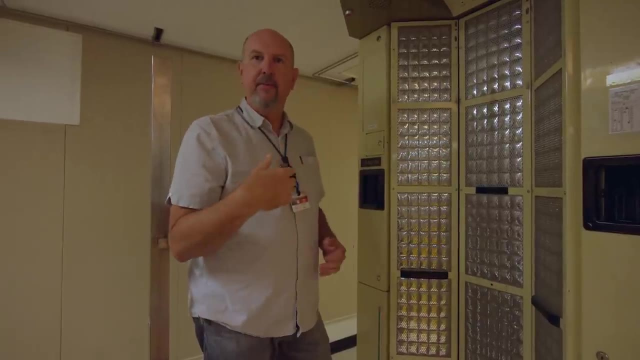 give me a doorbell, chime, ding, dong and then i'm free to go. if not, then all these guys at the control point, or radiation protection technicians, would come in and they would do a frisk of me with a, with a tiger mueller detector. doug, here is one of our rp technicians and they would be looking. 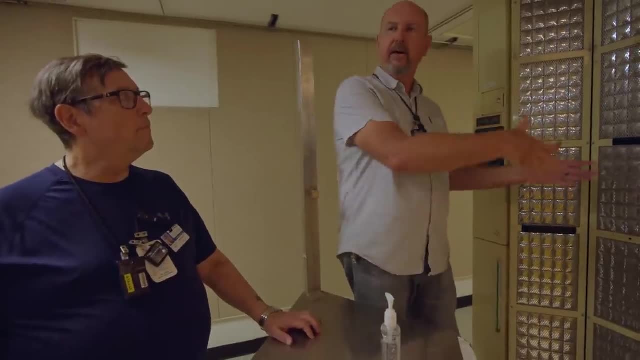 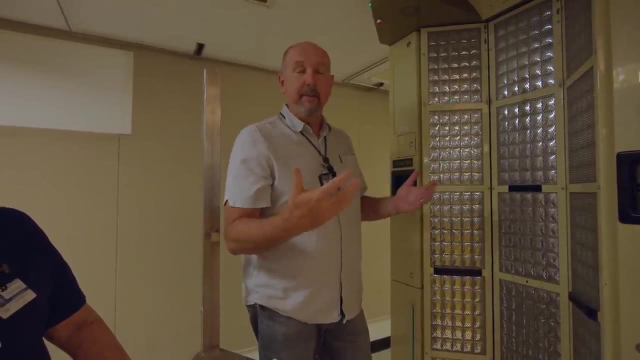 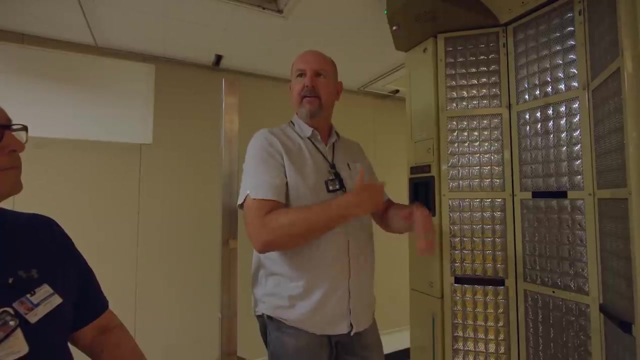 for contamination. okay, and then if if they didn't find anything, i would get checked again. i would have to pass twice success successively to be able to be released from the area. or maybe, if i was contaminated, they may have to. uh, maybe recover contamination from my clothing or from my skin via. 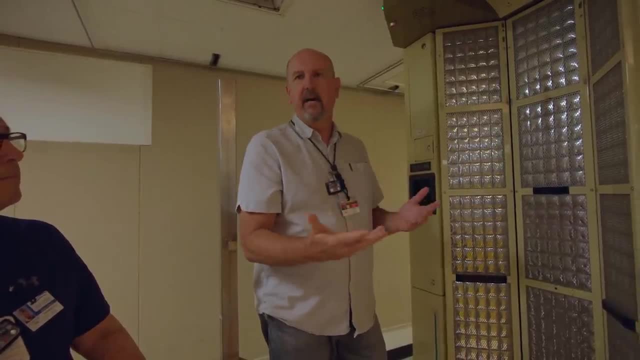 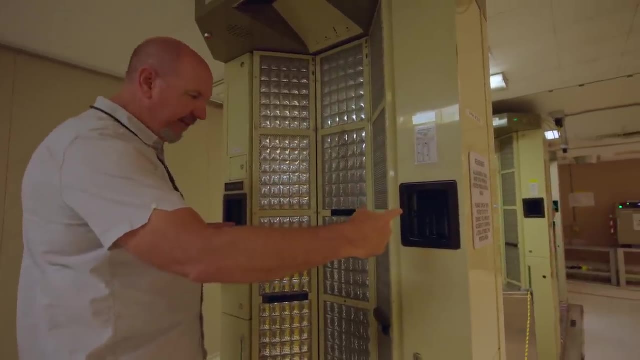 soap and warm water, um decon methods would be deployed. so i'll go ahead and try this, just to show you how. there's a couple of things here. there's a couple of paddles on the end in here that you have to depress. also, you need to break a couple of beams. here's one beam and there's one. 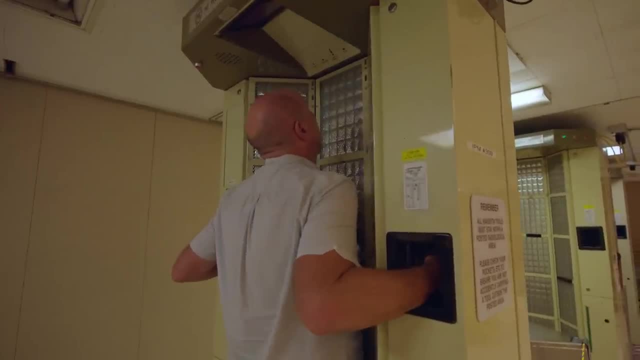 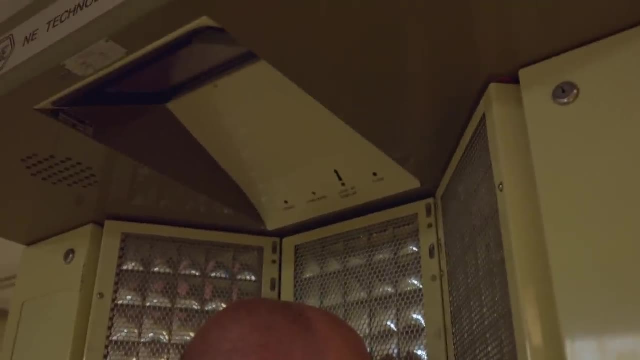 down by your foot and then you're going to take a couple of these paddles and you're going to feed, but you have to break that beam in order to activate the counter, so you can see up there that there's a yellow light on for telling me that it's checking me and so hopefully here in a few seconds. 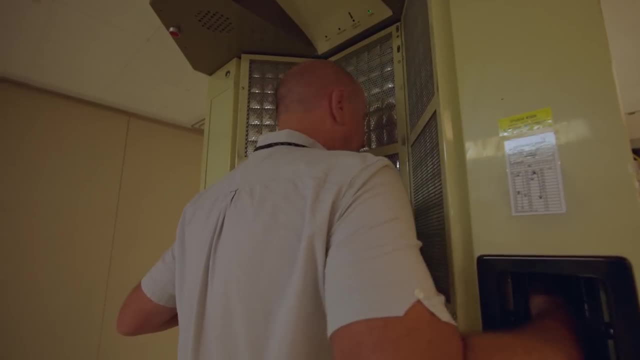 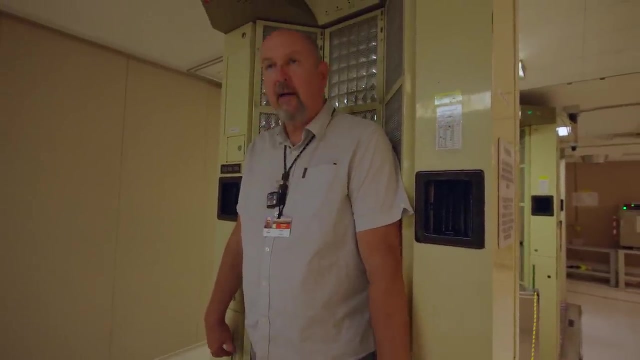 it'll give me a chime to tell me to turn around like that one. i'm going to do the same thing. i'm going to press in, not all the way, but but in, and then these green strips here. i'm going to apply some pressure with my fingers, okay, and you have to apply pretty good pressure, they would you think. 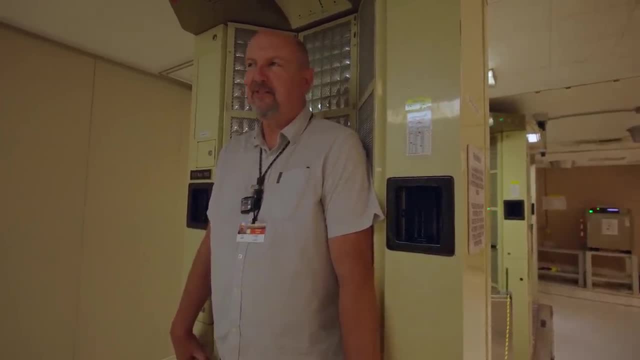 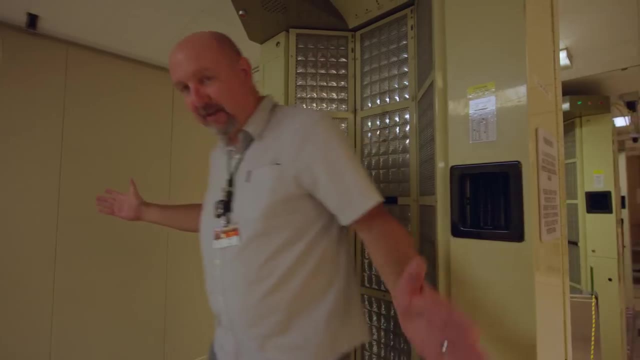 they would have gave you a simple button to push, but they didn't. they gave these strips, and so you're kind of straining and hoping that the 15 second count will hurry. yeah, yeah, and i'm playing ding dong, i'm playing all right, so now you're up. okay, can i go two? 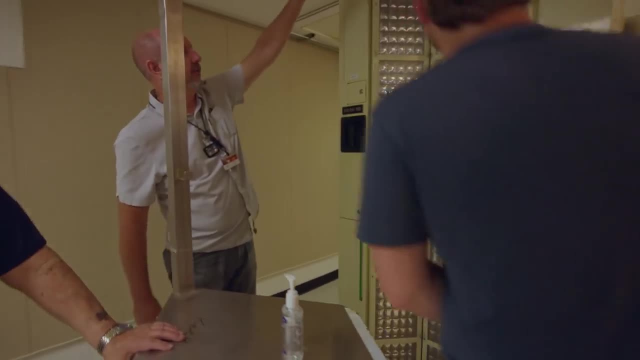 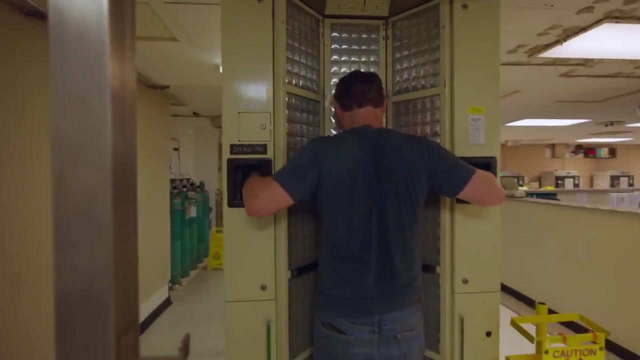 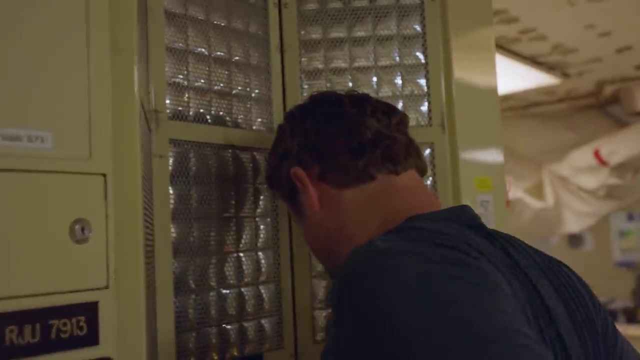 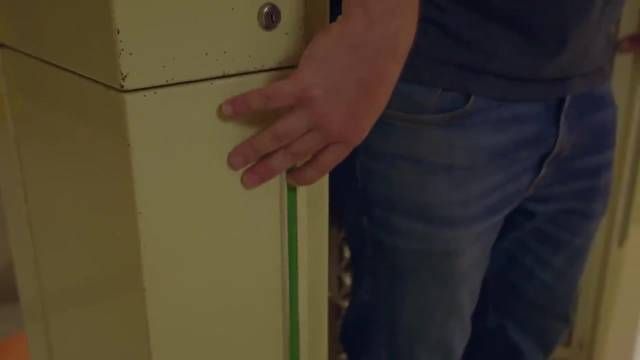 minutes. yeah, now, before you get get in, um, wait for the green light. so it's green now, so it's ready for you, so it does a reset. step in, push the bars and just right, exactly, so that should do a count. all right, and press firmly on those green strips. oh, that is awkward. yeah, what idea maybe? okay, push down. 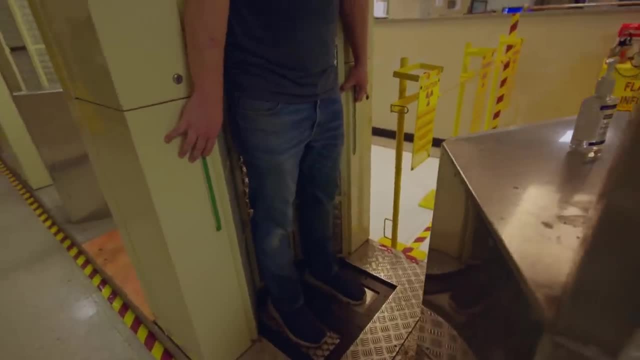 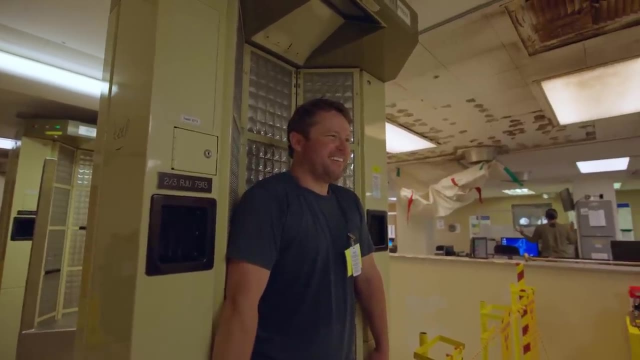 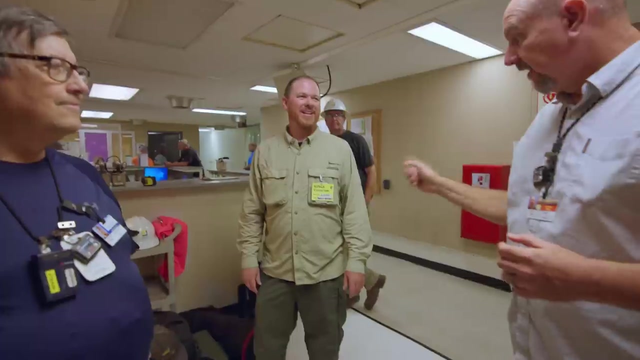 all the strips a little firmer, maybe further down on the strip. there you go hold your breath. most people they do one of these and then they break the beam and then all of a sudden it stops. hey, trying to get comfortable, right, yeah? hey, that's nice, you're good. this thing is susceptible. 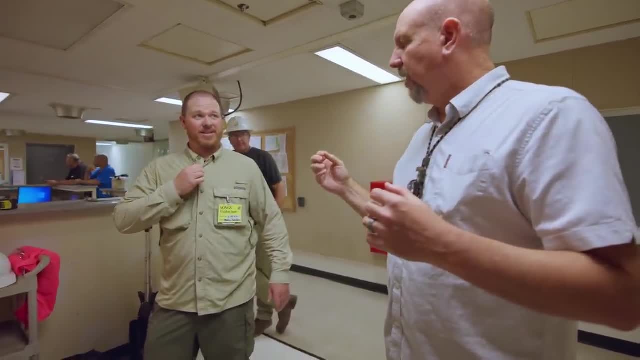 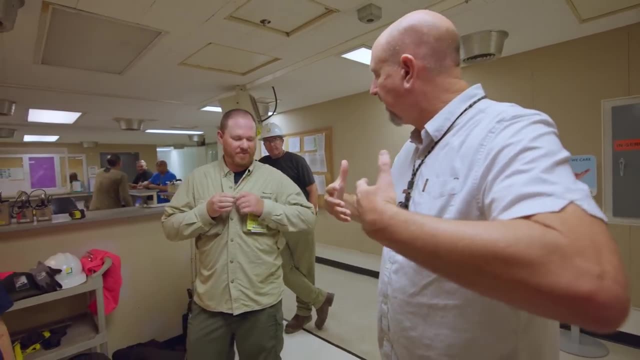 because you think i should touch it. um, i don't want you to go shirtless. i have a shirt, okay? um, i would recommend you do that because what will happen is is it'll create static and that's radon will attach itself to you for sure. 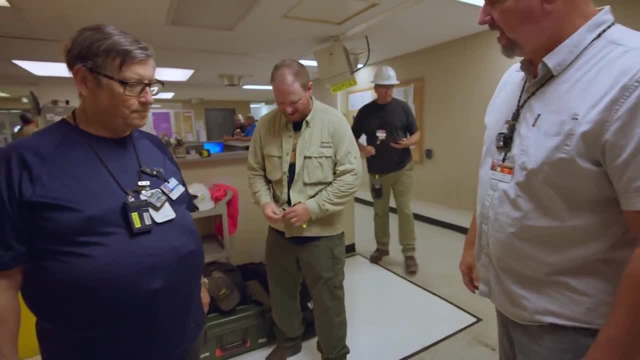 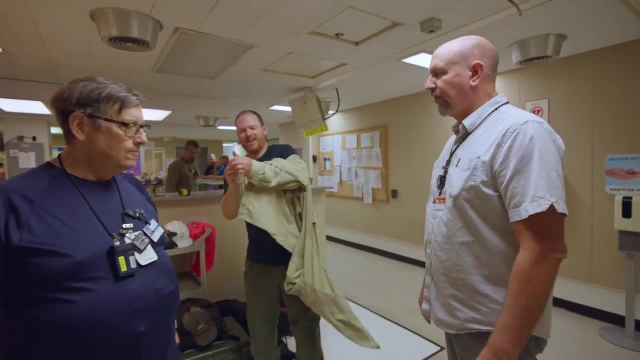 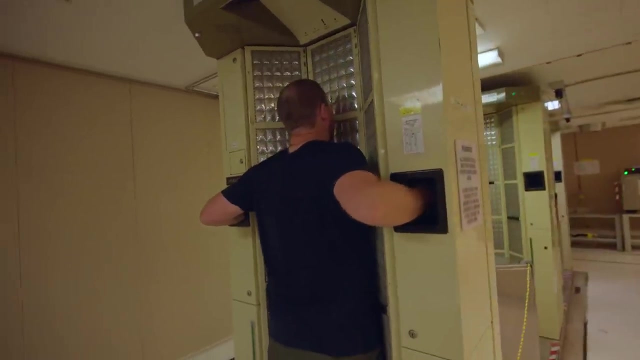 oh, yeah, okay, smoke with your vest and actually it's. it responds the same way as your vest. would any kind of polyester blend or polyester material, for sure? yeah, all right, so let's go ahead. tobacco products: there you go, turn around. go ahead and turn around and 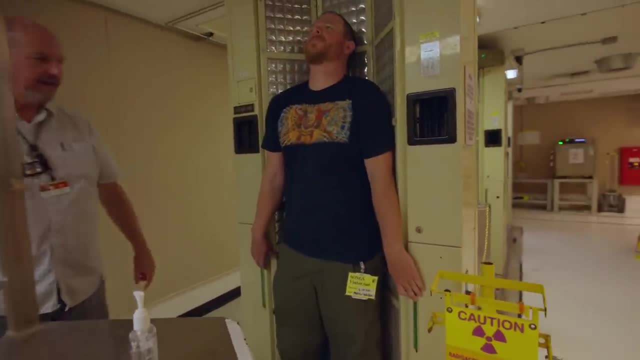 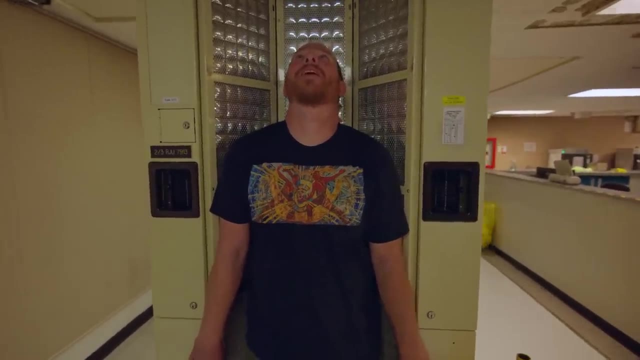 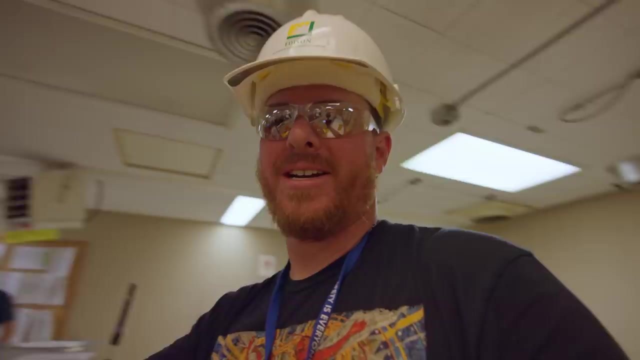 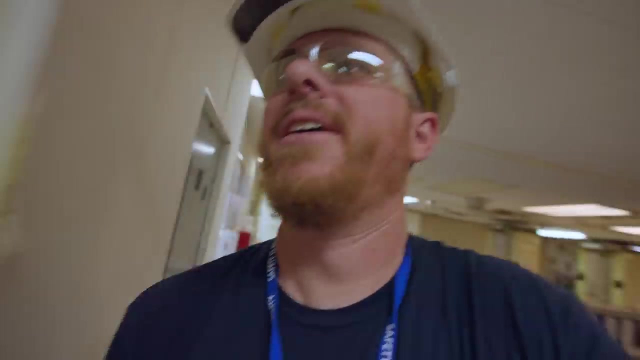 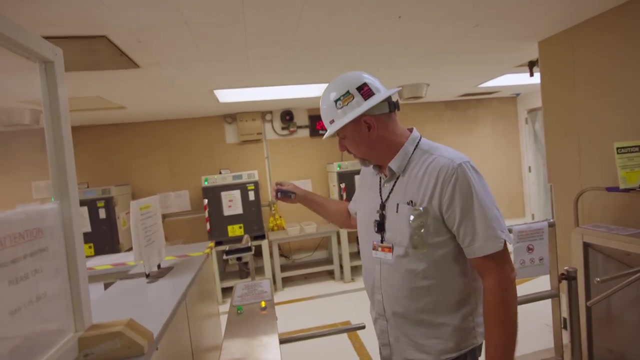 press all those green strips firmly, and further down on that strip the better. it's like the beginning of the running man, i know. them into the sled. yeah, i know, drop down into a tunnel, all right, thanks. all right, check and see if our equipment is hot. hey, proximity detector, and that's to make sure this thing is turned on and actually working this. 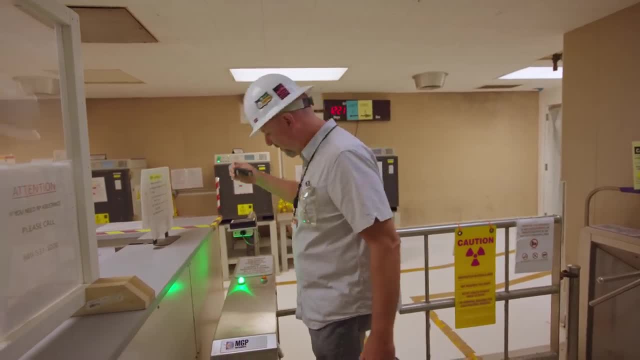 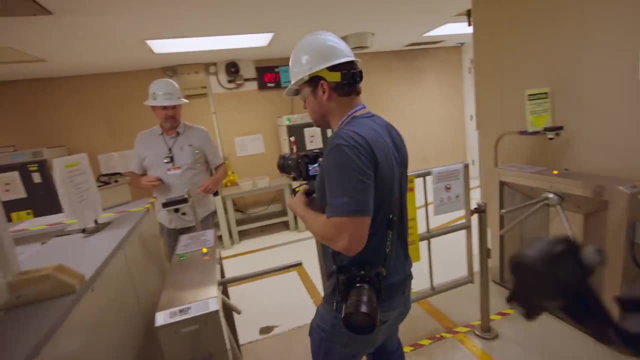 is just an access control feature that we use here just to make sure that people are going to be monitored while they're in the radio control area. so if you guys want to do the same thing, put your um electronic decimeter next to this. this should release the turnstile and allow you to come. 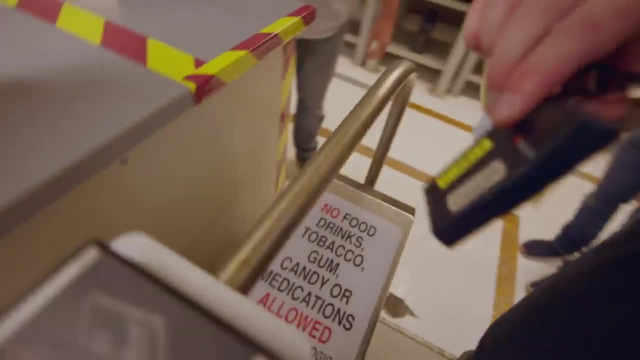 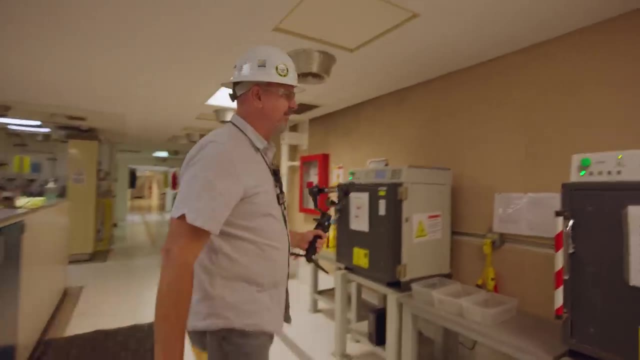 in all right. so the next thing we're going to do, i'm going to reach across. yeah, normally we don't allow people to do that, but i'm taking some executive privilege. we're going to use one of these monitors. this is, like i said, a small articles monitor. we're going to use this to. 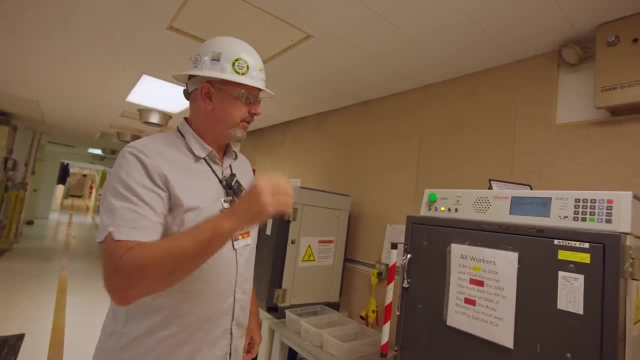 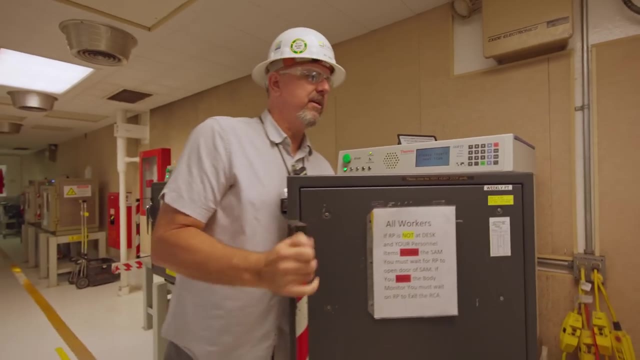 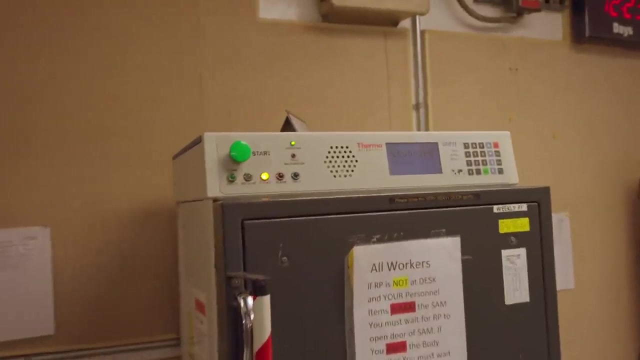 do a baseline check on all of your equipment. let's make sure this passes, and it did so. that was clean. that's a good sign. the next step will be to put your cameras in one at a time. all right, all right, we're in the final count. 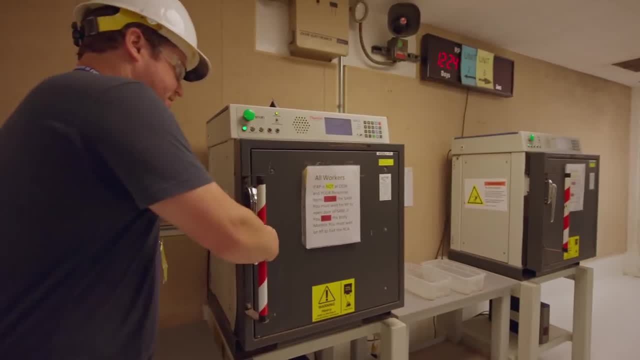 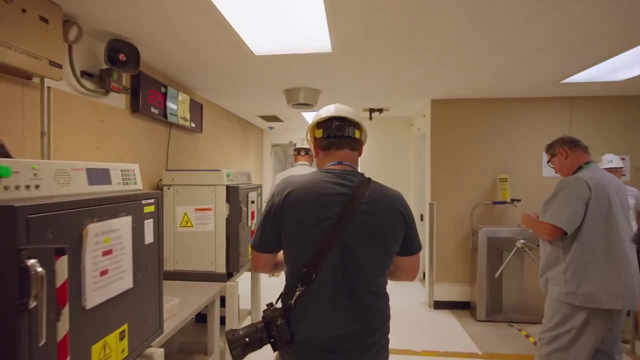 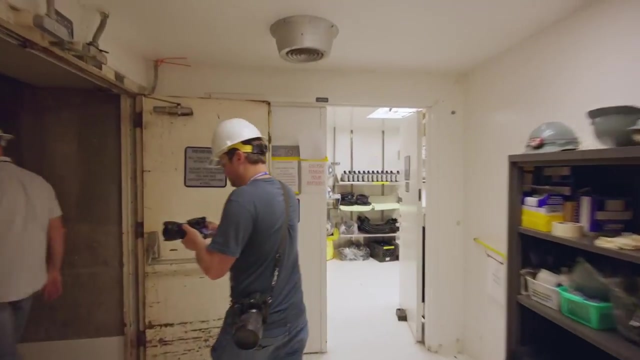 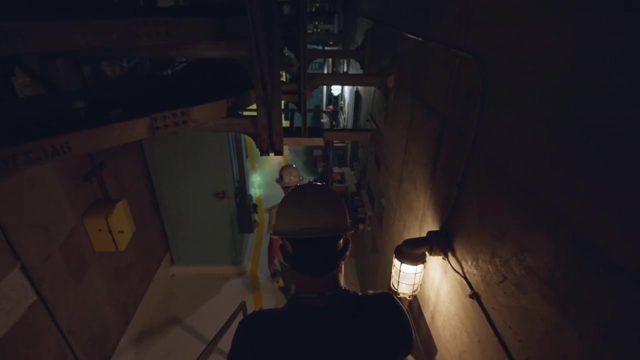 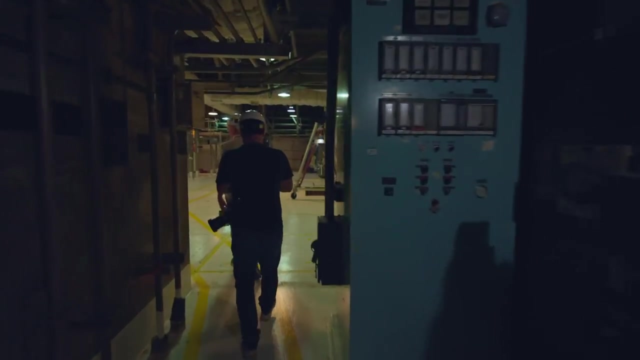 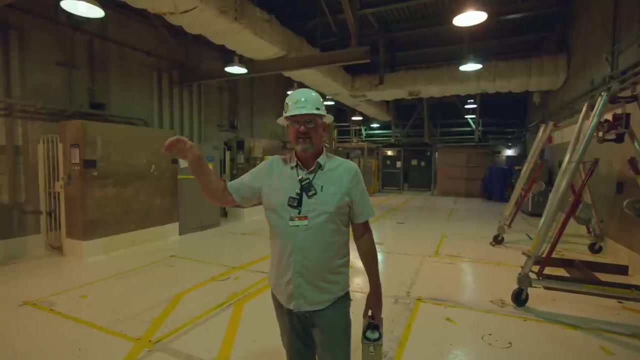 clean, all clean. okay, you guys ready? yeah, all right, you got your ppe ready to go? yeah, yes, so we just left the radways control point. that's our main, our rp, uh, radiation protection access control point. that, um, basically, is the boundary, the entry point for the whole radiologically. 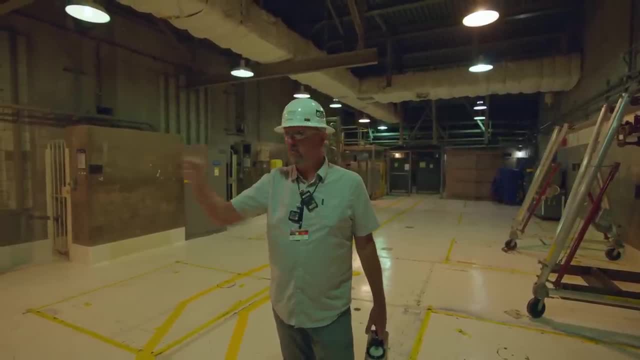 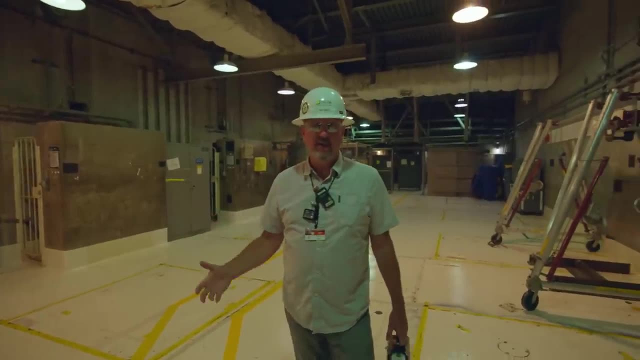 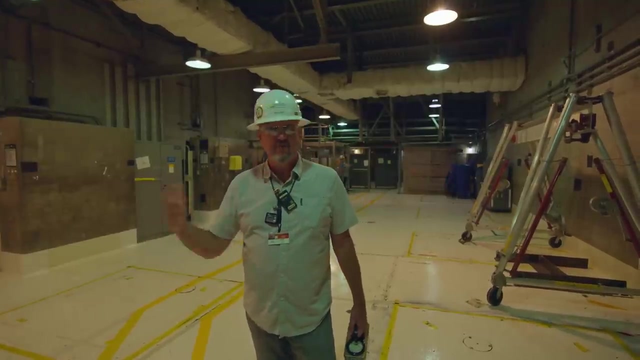 controlled area for the uh, for the power block here. right now we're in the radways building a lot of plants. call it an ox building, auxiliary building. this is where a lot of uh pumps and uh isolation systems and so forth- all kinds of uh uh volume systems and all kinds of uh uh. 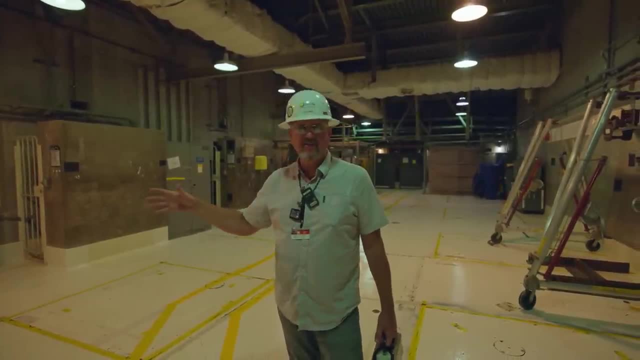 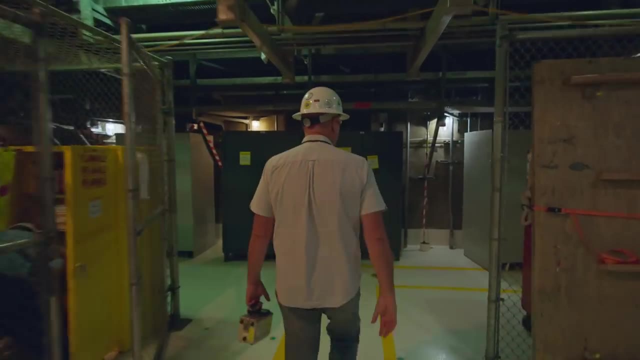 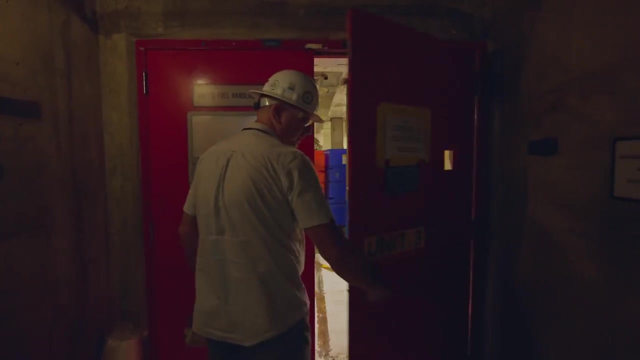 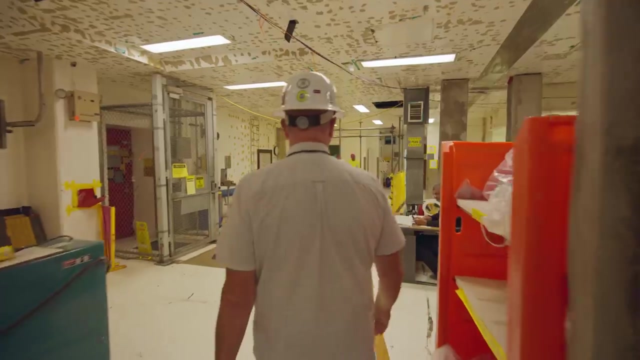 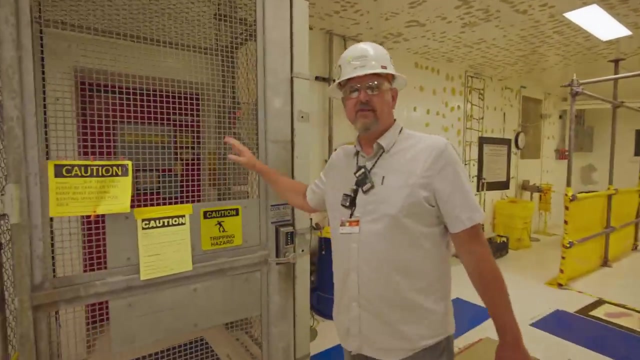 control systems for chemical injection, stuff filtration. all that stuff is housed in this, in this area here. um, we're going to head over to the fuel handling building. all right, don't have to be cold for here anymore. it's a safe being home, all right. so this is the outside of the spin fuel building. uh, this is a unit three side spent fuel building. 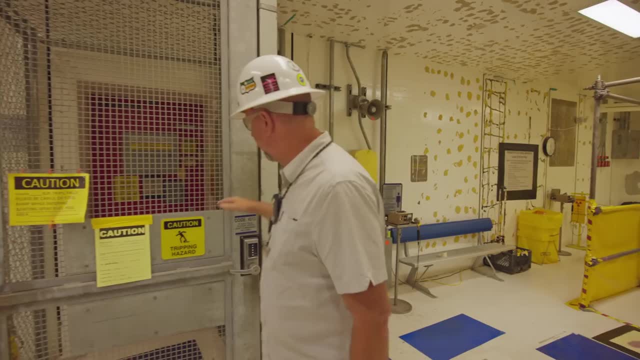 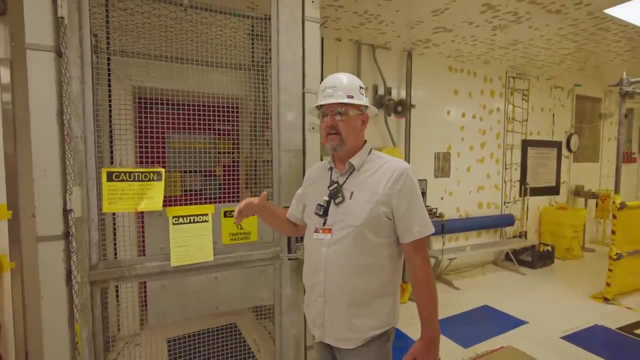 and we had some security controls that were in place here that um still left over. go through the door and go into the building. what you'll see when we go in on your right hand side is a large pool area- spin fuel pool- where we used to store all of our spent fuel, which is actually now. 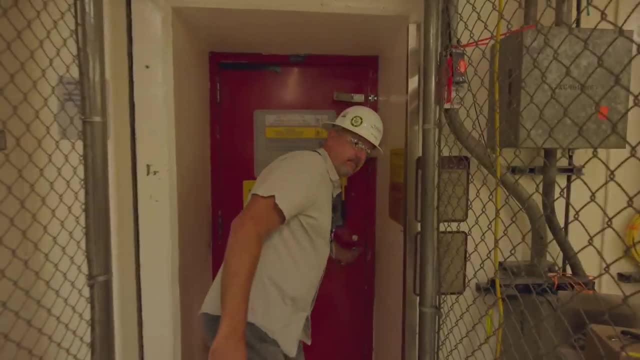 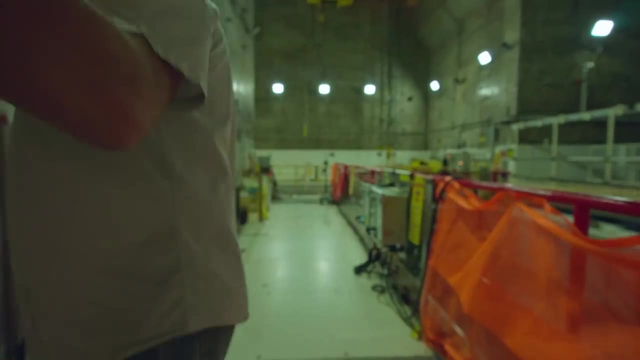 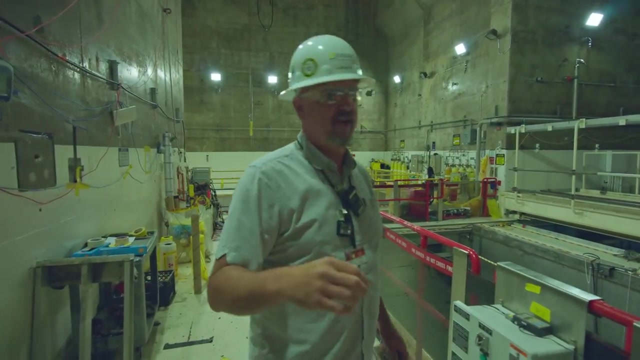 stored over on the ssc pad by the door. yeah, this is a sign we have. we post all areas, so this is the area when we're reefing at the control point. uh, the supervisor up there was talking about a yellow area or yellow pipe. that's the. 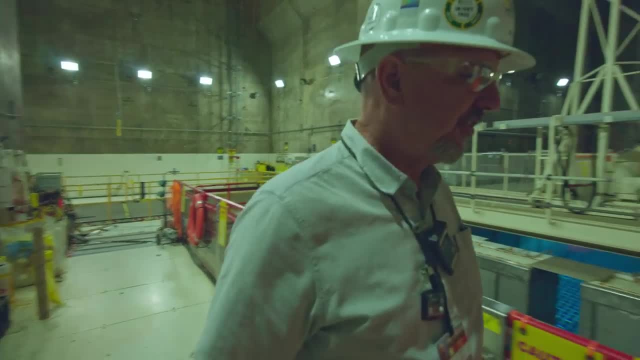 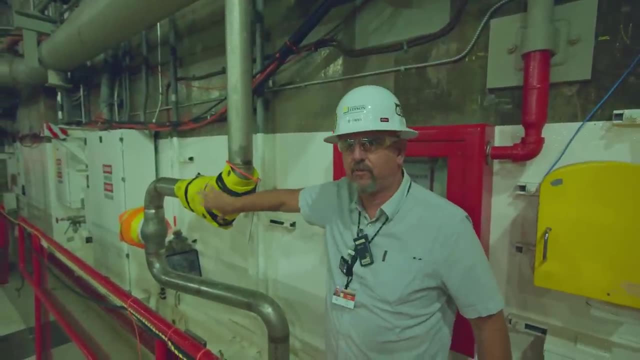 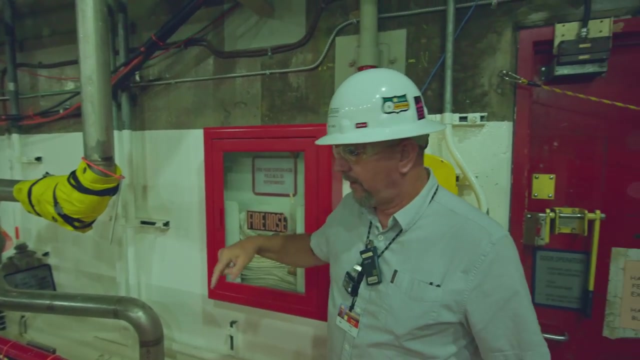 pipe right there. this is a just normal plant shielding that we have. it's a lead shield and it's just coated in heavy plastic. there's no contamination, it's just for radiation dose level control. this was actually a cooling pipe that would supply cooling to the plant or to the pool. 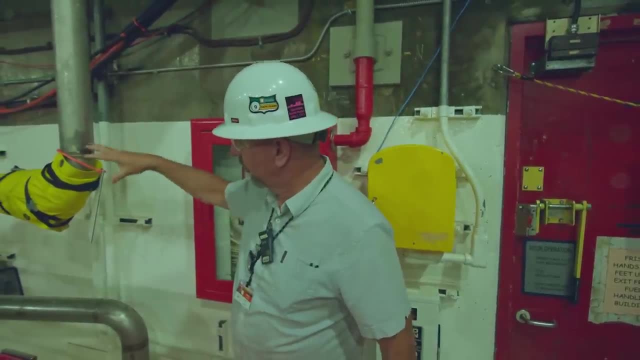 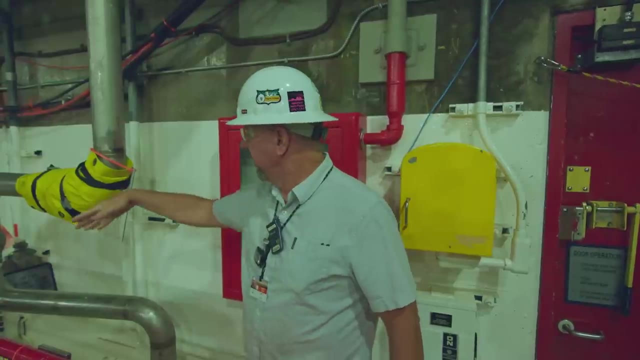 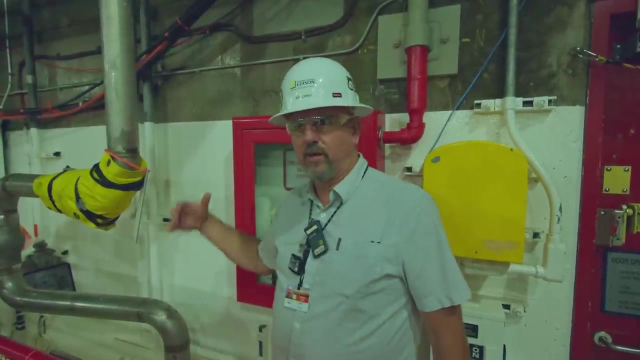 and so this was just an elbow, where you know when the valve was closed or whatever. we just create like a little crud traffic, so rad levels would increase, radiation levels would increase, and so we put this shielding in place, part of our normal plant processes for controlling worker exposure, just to knock down the dose rates, just so as people walked into the door. 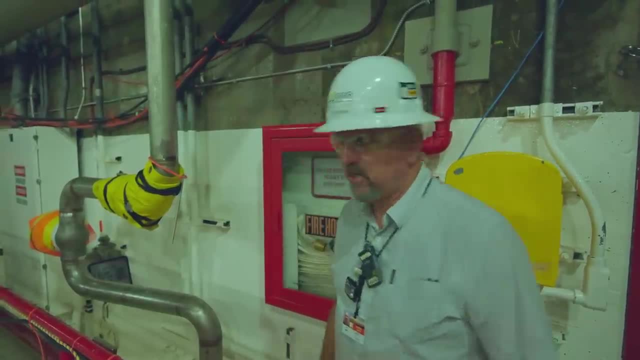 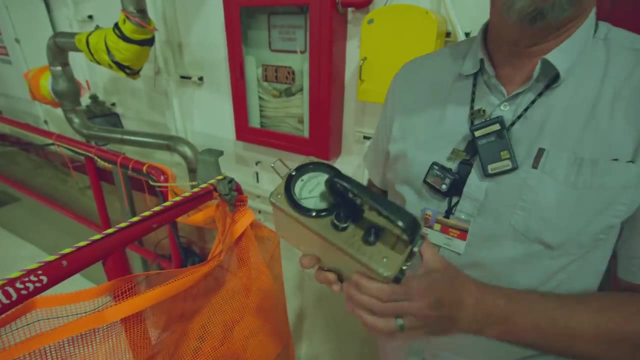 or worked in this general area. it would reduce their exposure overall. so this is what we use here at the power plant. this is common for all of the power plants. uh, in the in the nuclear industry. this is a heberline ro2. it's an ion chamber design. it's a little bit different than your. 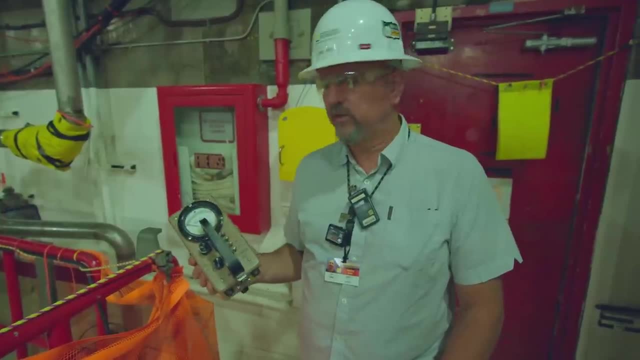 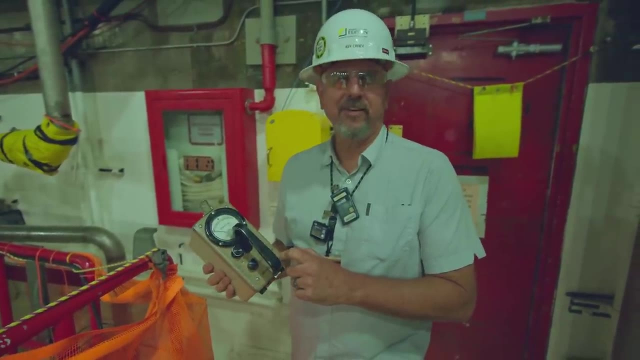 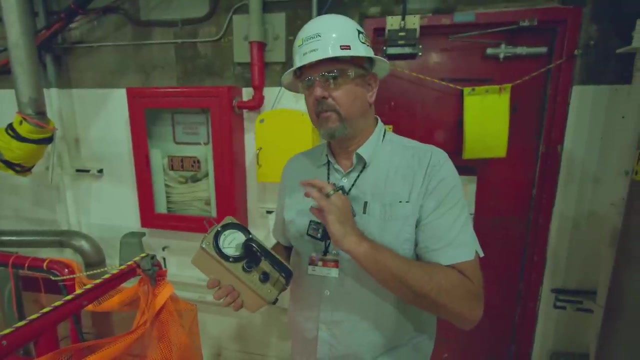 rat eye. your rat eye uses a different detector, uses a geiger mueller detector and this is an ion chamber detector. and so much is better. we use these. they're both good. we use these in the industry only because the detector design is the most akin to file absorb dose biologically all. 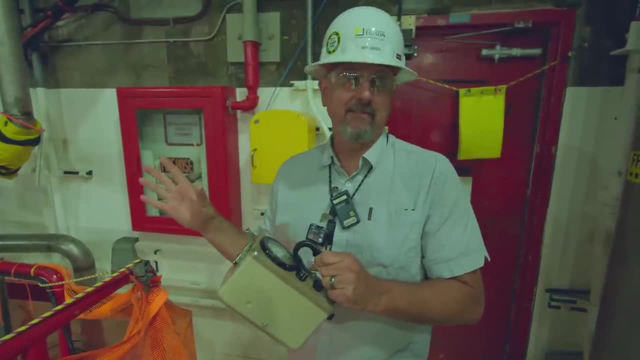 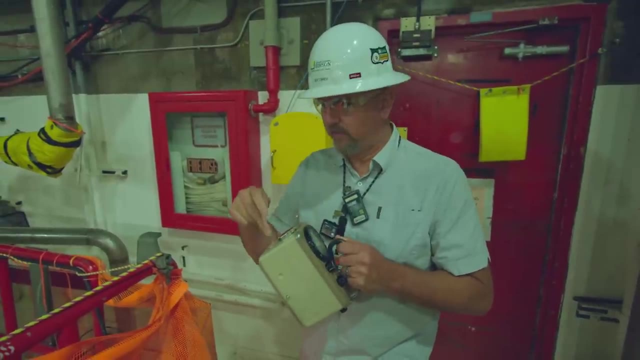 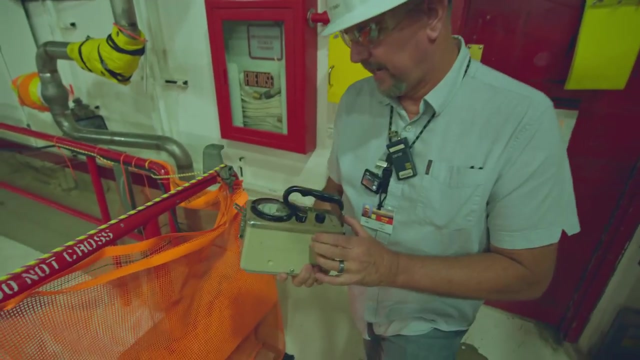 right, so, um, so this is what we always use for for dose rate, establishing dose rates, so that we can. you know, we monitor and we set up all of our dosimetry programs based on what we get really from this type of instrument. so for this one right inside the door here, and i've done all 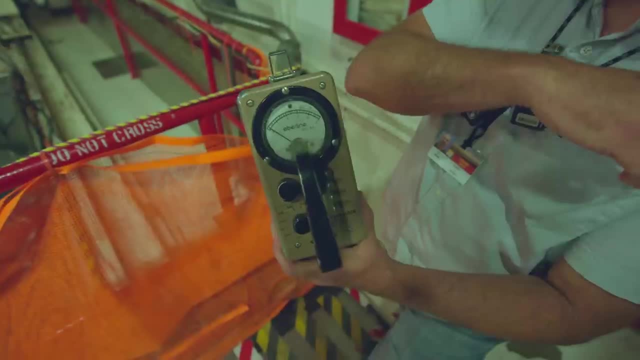 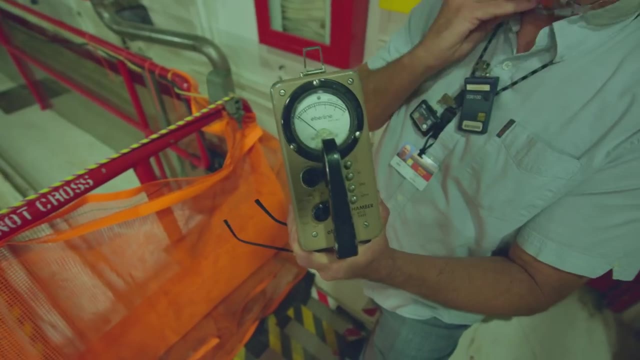 my preliminary operational checks. you can see, i can put my glasses on and i could tell you that i think what we'll see here is like 0.2 miller per hour. yeah, i don't know if you're familiar with the scale. the scale we have a, basically a times. 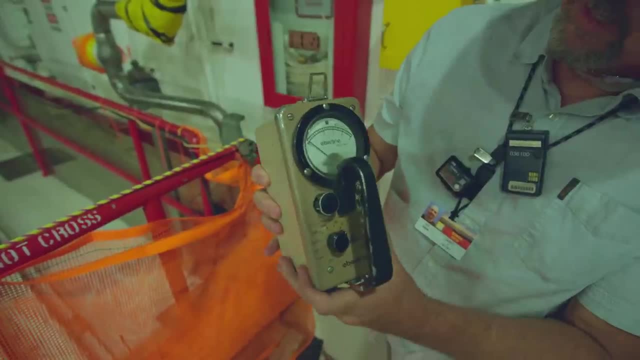 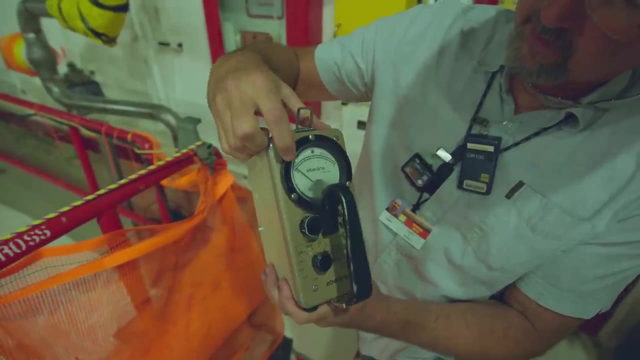 one. it says 550, 500. it's basically times one times ten, times 100, obviously. so we have times. one would be one miller per hour. we're down on the first line there, which would be 0.2 miller per hour, and if we went over 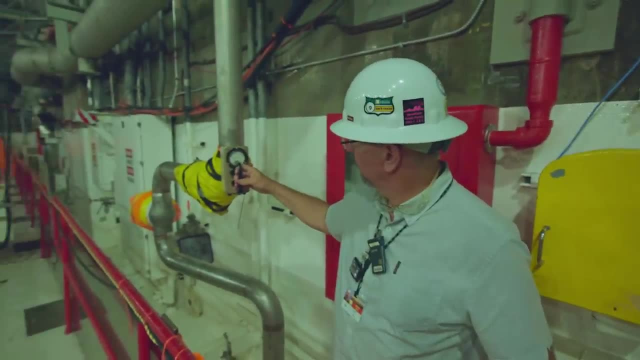 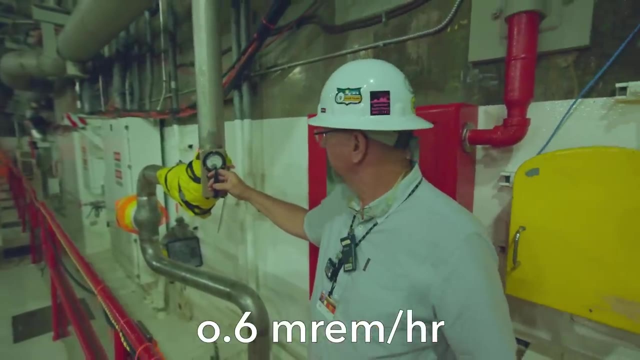 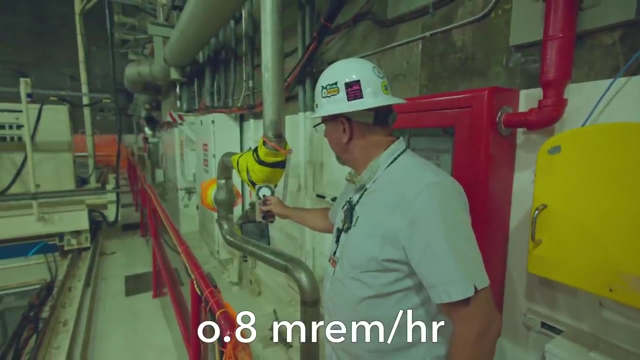 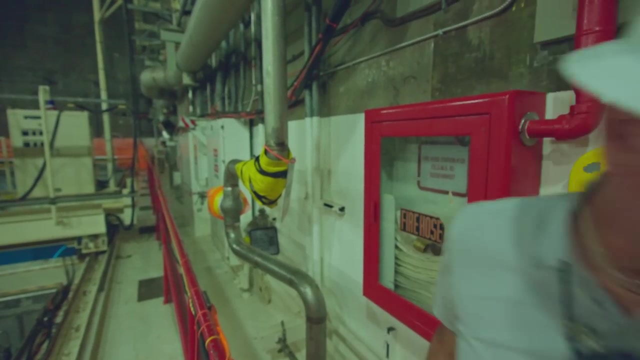 this area that we're shielding. minor increase in dose rates up to 0.6 miller per hour. 80.8 there. so if i take the shielding off, i'm not sure what it would be. i'm curious like what my- uh, my radar will pick up. check it out. 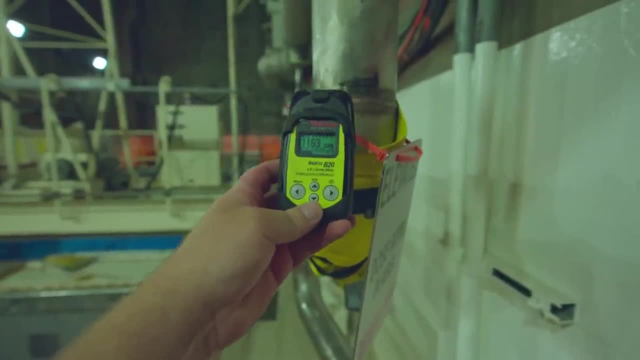 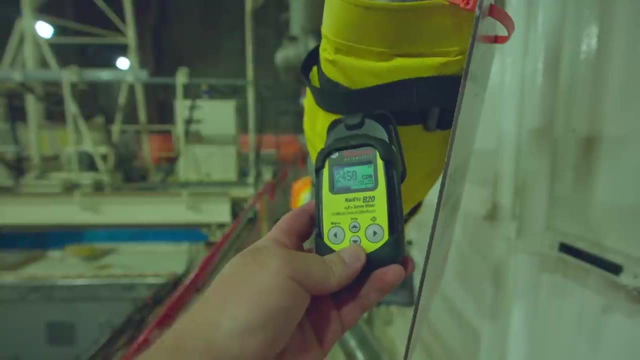 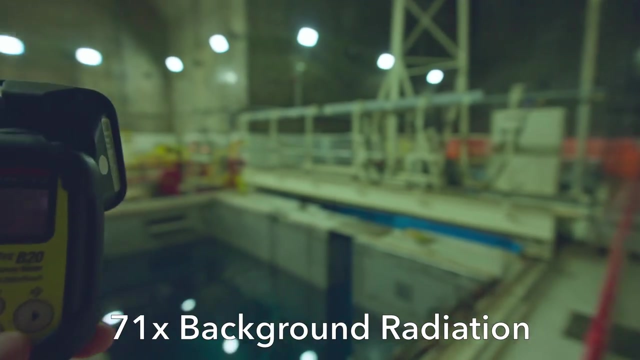 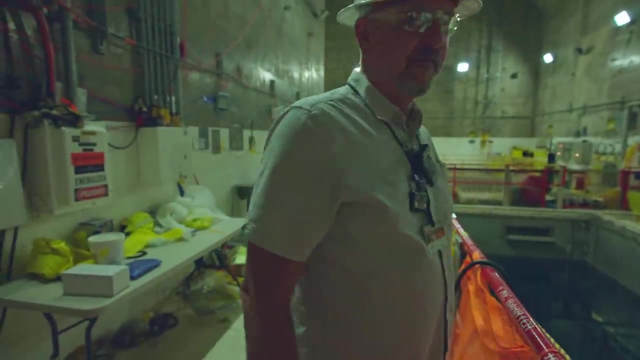 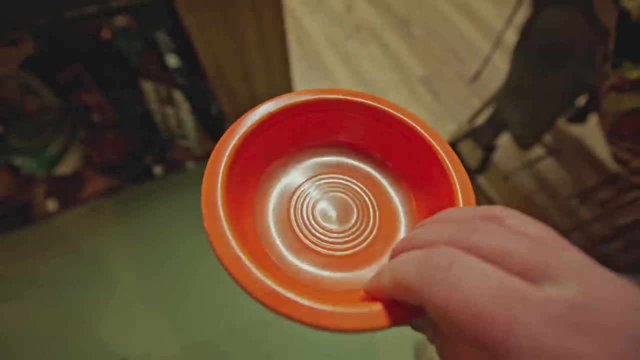 so everything i've seen here so far. i could find stronger stuff in an antique lot. yeah, yeah, especially all of those um, all that fiesta wear got a lot of, uh, densely concentrated uranium and so, yeah, it's, it's. we have tours out here frequently. i used to run the radius protection. 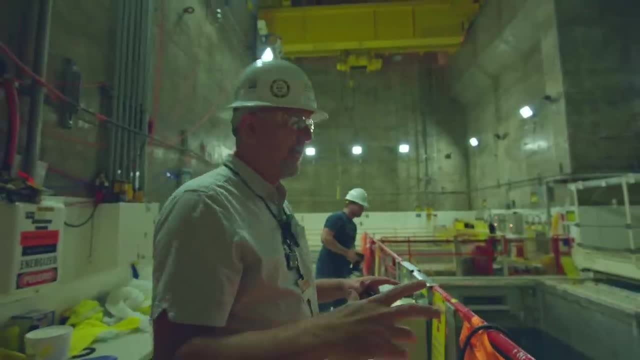 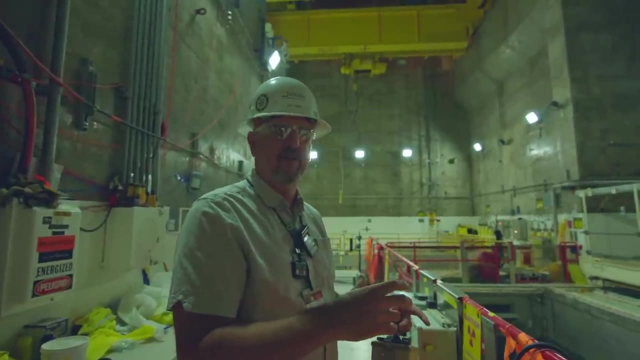 booth where we have all the stuff. like we had an old piece of fiesta wear, we had a smoke detector and we had an old um, not a, not a- radium dial watch. like you pull out of an old world war ii airplane or something like that, but an older, older clock that still had some minor radium in it and you 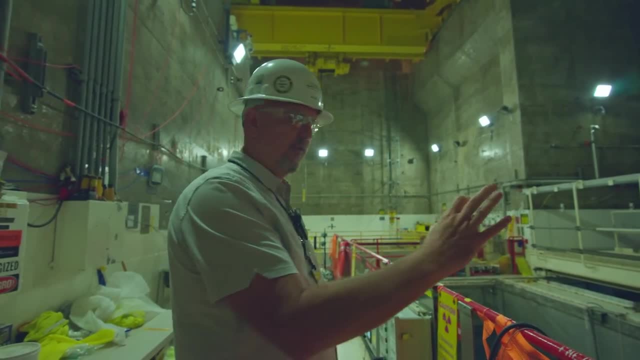 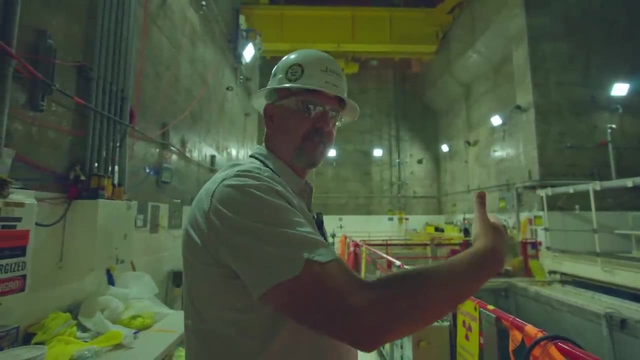 know you can take a frisker which has the same detector as what you have in your rat eye and you put it on there, you can definitely see some activity. you can put it on there, you can definitely see some activity and so it's good demonstration for you know radioactive. 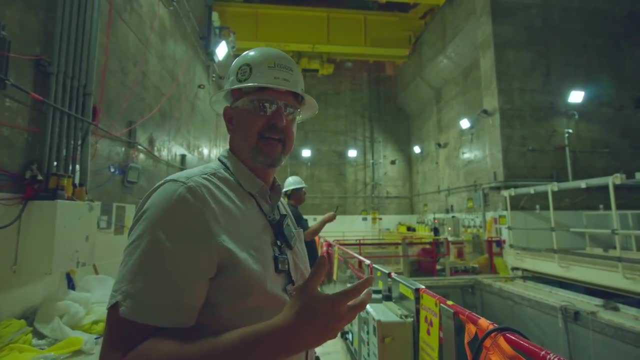 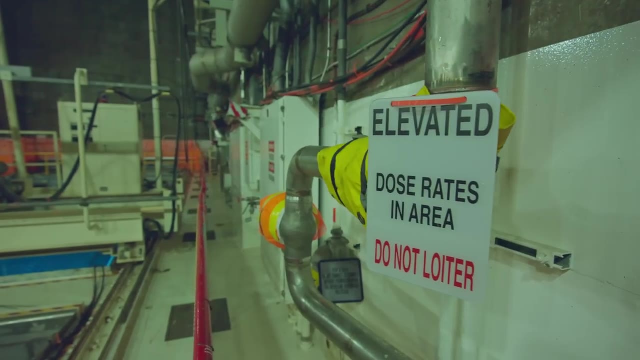 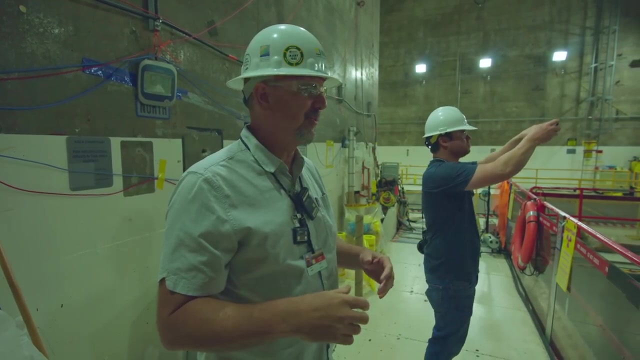 components that were out there in normal living space. let me fix this sign real quick. this is where we stored all the fuel. usually, you see, like on the simpsons, you'll see something green glowing and something falling all over the floor and goo going everywhere. it's really 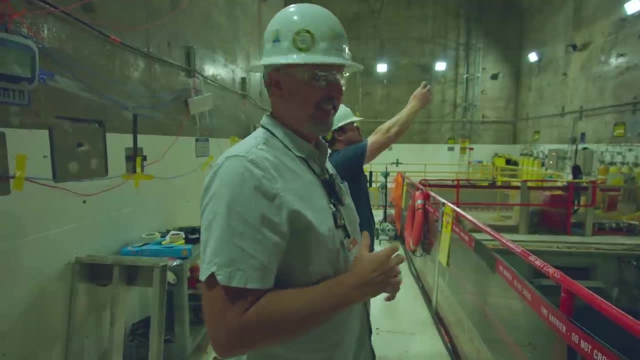 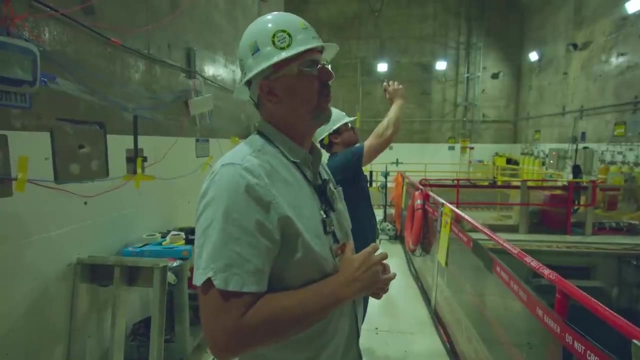 totally not what happens in a nuclear plant. it's all a solid, yeah, because it's like solid ceramic pellets, exactly like in a zirconium, right? is that what it is? it's um zircaloy, um some special metal, uh, zircaloy pins that are basically hollow and you. 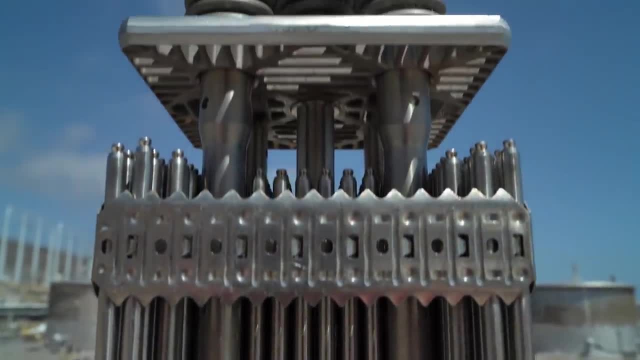 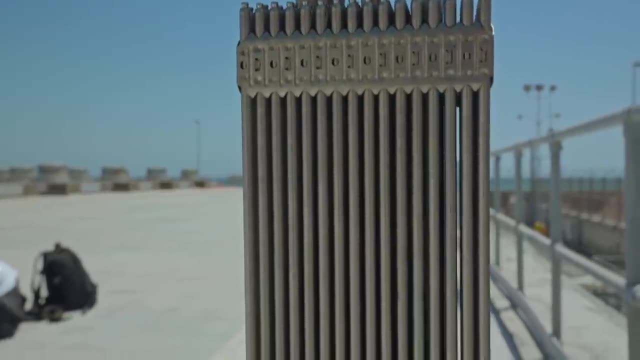 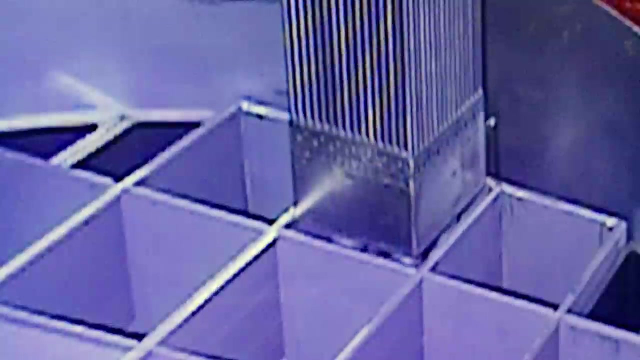 feed fuel pellets in. they're spring loaded so that they're they compress. and then there's a whole collection of made fuel. assemblies are just a collection of those pins, a large collection of pins in a specific square size so that they fit down in those slots. and we had several hundred in there stored just from the life of the plant and so 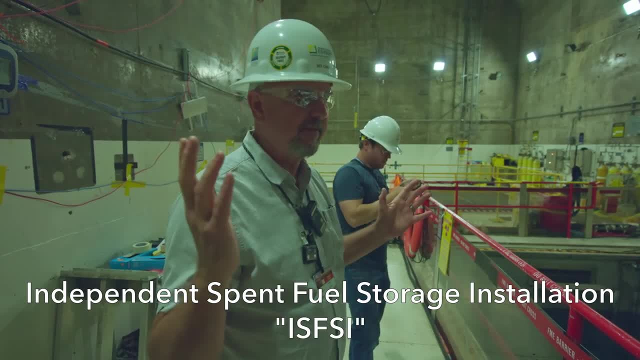 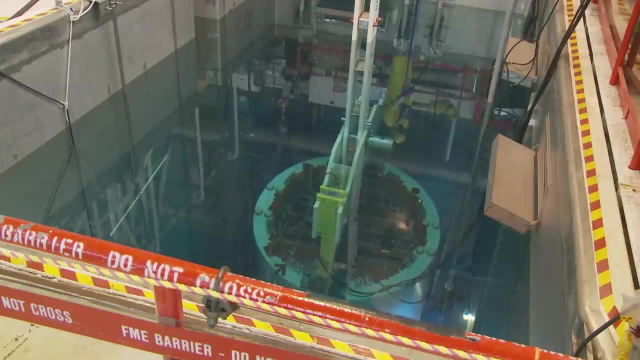 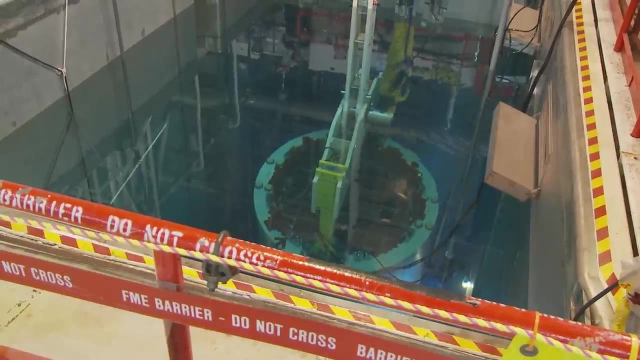 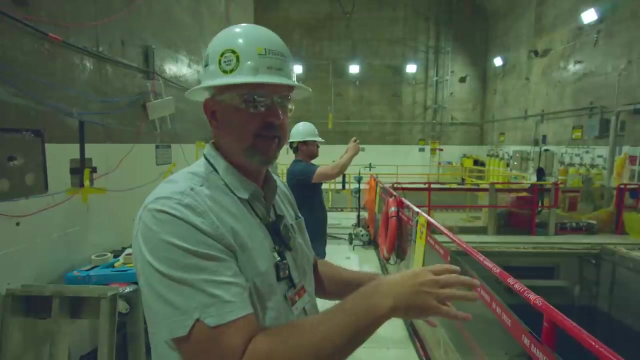 over on our independent spin fuel storage installation- we call it isfacy. we unloaded all those fuel assemblies into individual canisters which had a bunch of design, shielding and like a its own rack inside, and loaded it up with fuel, took it out after we cleaned it, decontaminated it, shielded it, vacuumed all the water out through a vacuum drying. 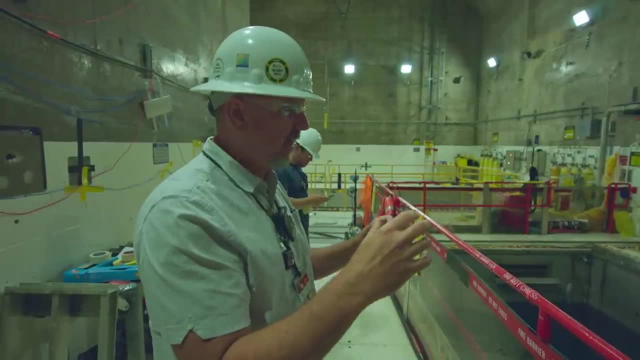 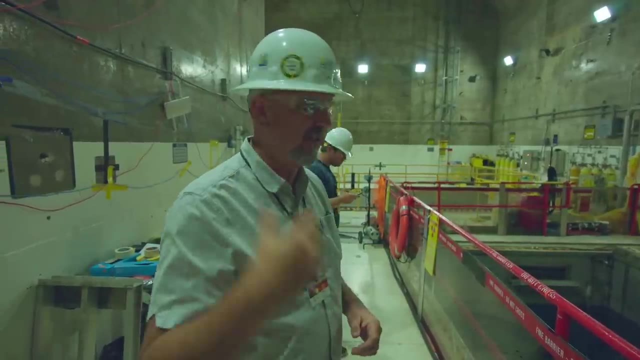 process, fill it with helium gas for continual internal cooling and drying and then shift it over to the pad where it's stored in the modules over there that we'll see later- right after it came out of the core and was being transferred in here, and especially if the lights were dimmer. 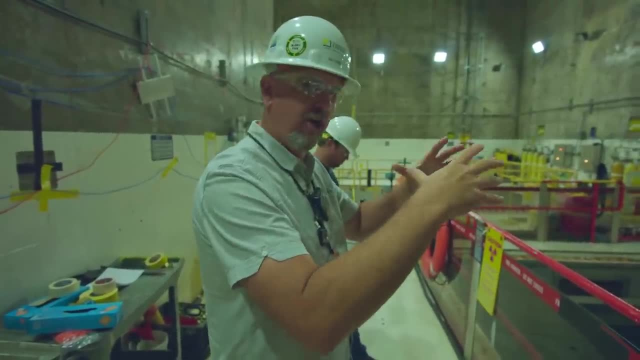 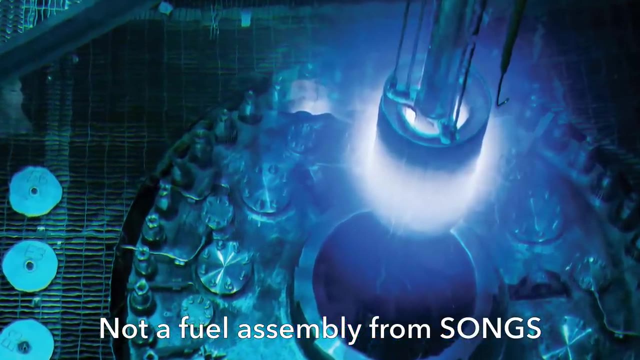 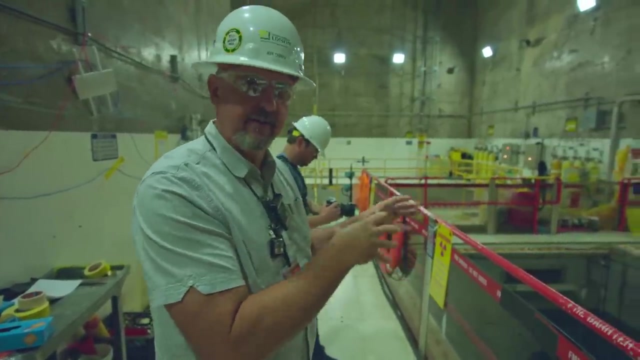 you would see a blue of a blue glow all around the beach fuel assembly and that's sherik off radiation, that's, you know, a lot of high energy betas and stuff coming off of the uh, the fuel assembly, being refracted through elements in the water, isotopes and uh and and. 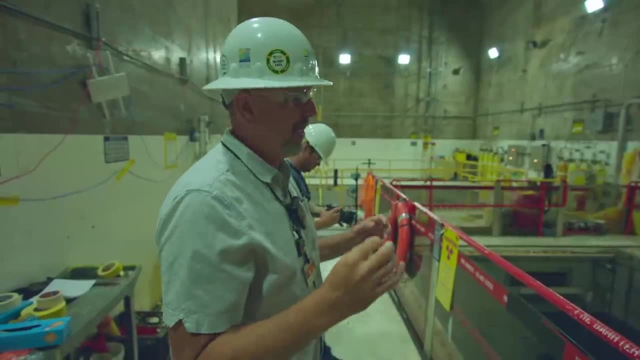 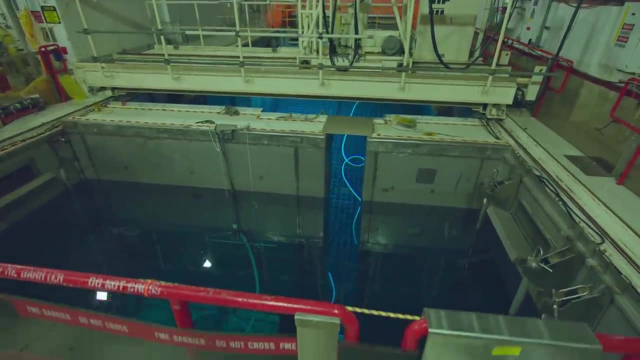 basically, it creates the blue glow that you see. that blue glow, which is, um, i guess, akin to this a little bit, is all you see as far as a, a color element associated with radiation, that's, and that's the only place you would see. it would be around, uh, a full volume of the building in here. 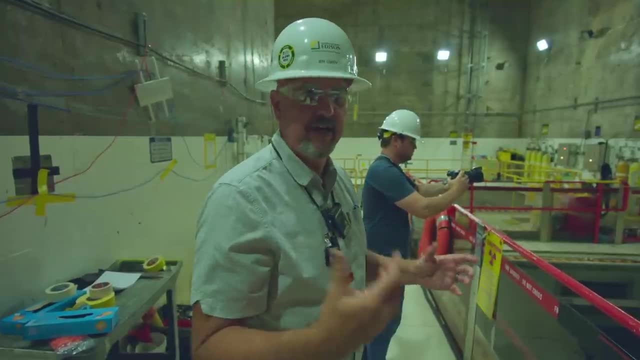 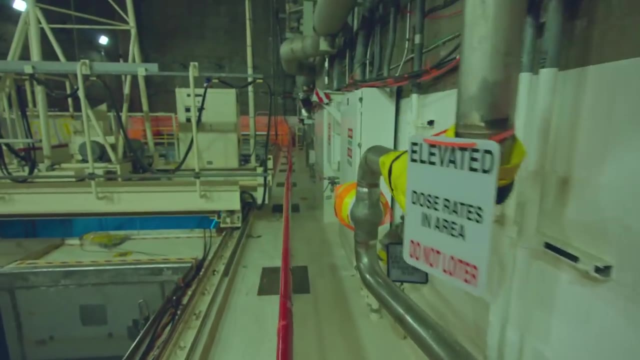 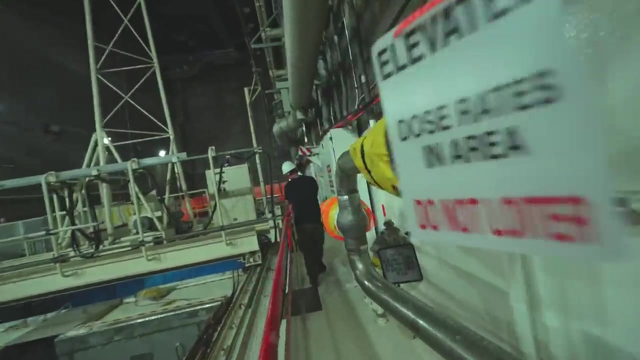 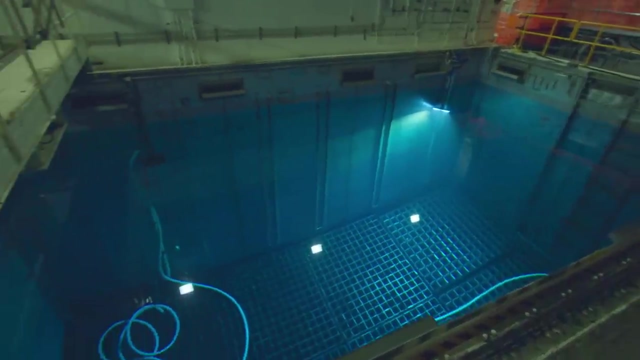 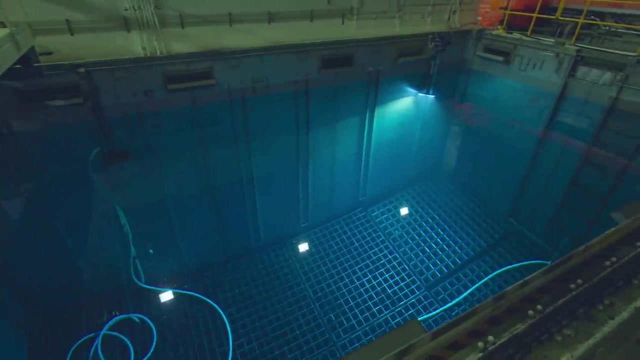 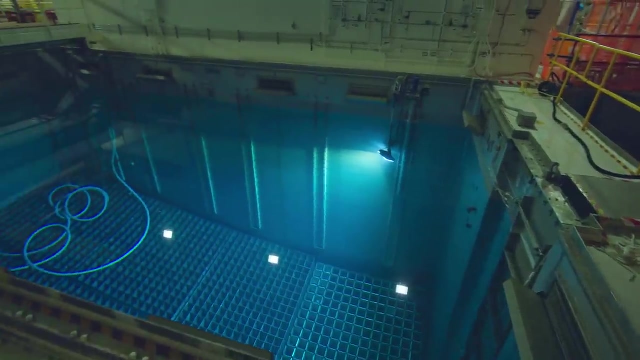 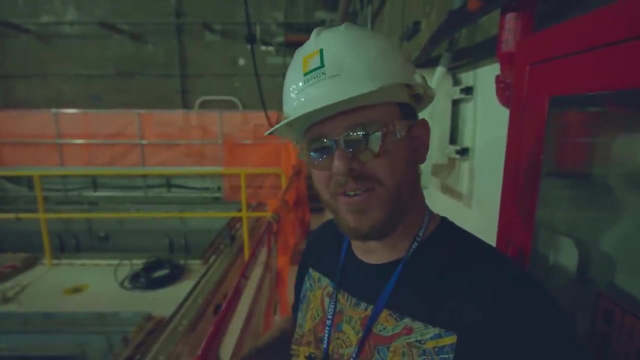 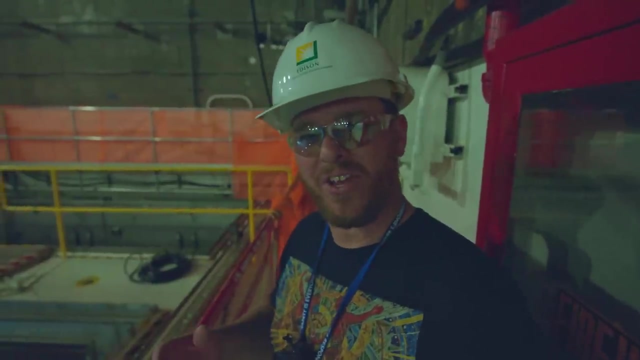 freshly recovered fuel assembly that was recovered from the core right after a cycle of operation. So this is the spent fuel pool, where the spent nuclear fuel would have sat and cooled down over a course of about three to five years. It's very cool. Unfortunately, there's no fuel in here today because all of it has been moved to where they're doing the dry cast of, where they're storing the fuel on site. 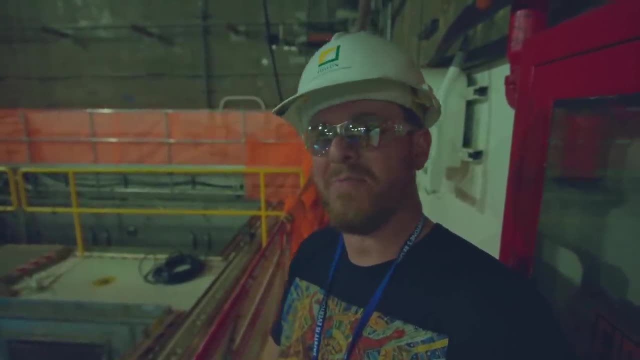 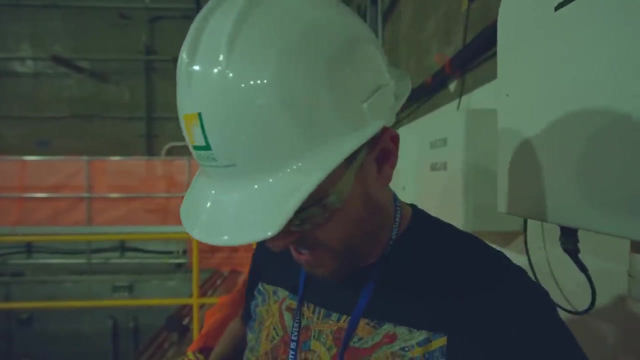 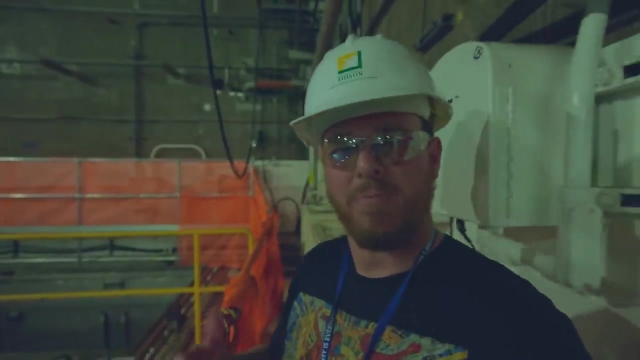 And so it no longer needs to be in this pool Any longer. So this is very cool. So while we're in here, too, we're also fitted with personal dosimeters here to check our radiation level while we're inside of the fuel pool storage area. 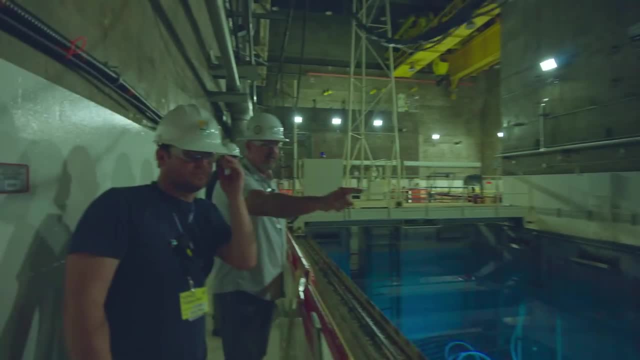 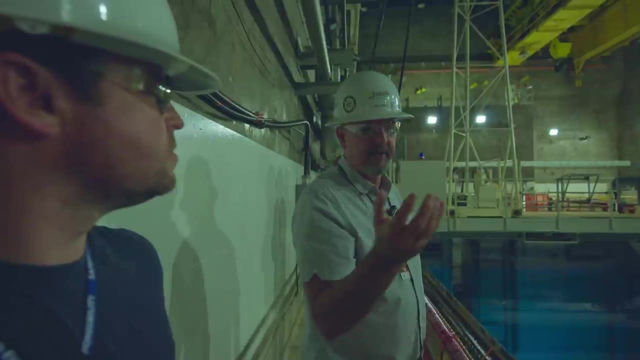 It's a very interesting place. to be for sure, There was our upender pit, And what it's called an upender pit for is because down at the bottom of the pit there's actually an upender. Basically, there's a tube. 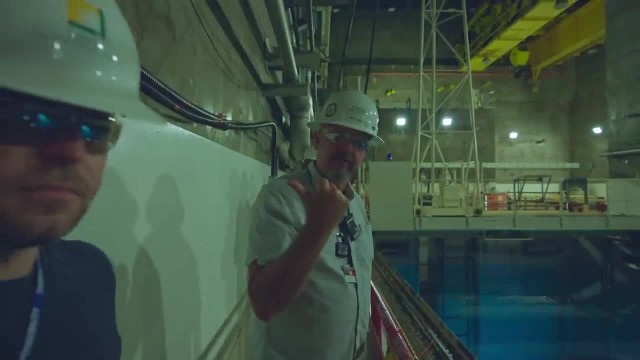 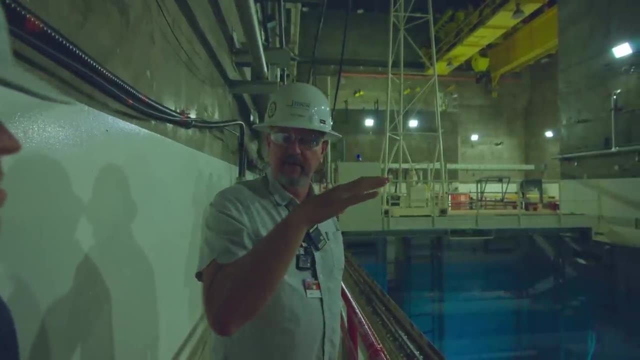 There's a tube at the bottom of the pit that connects to the refueling cavity over in containment next door. So whenever they would do a refueling, they would remove the reactor head after they flooded, as they flooded up the cavity with pool water similar to this. 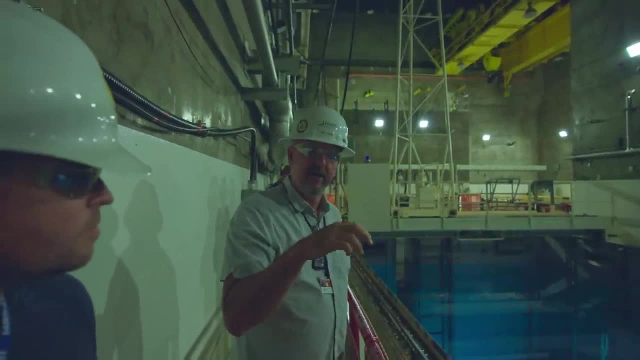 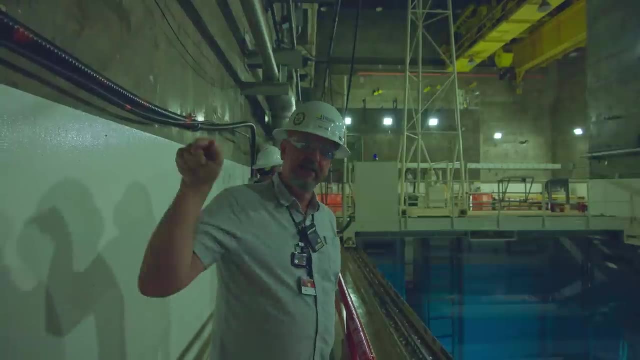 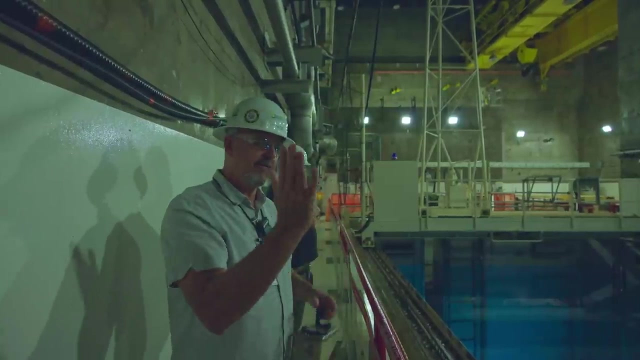 And then all of the fuel, one stick at a time, one control assembly at a time, would be removed from the reactor cavity, put in an upender over there which is basically just a hydraulically operated cell, Put the assembly in and then it gets down, ended and then it goes through a conveyor type mechanism over to this side. 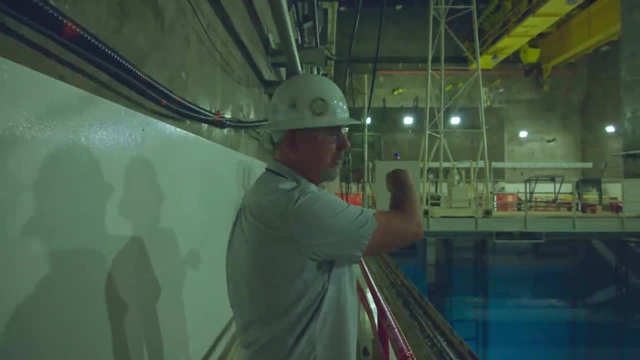 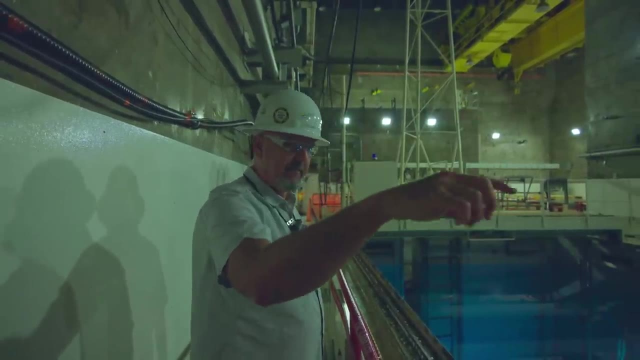 And then it would be upended where it could be grappled with this machine. This is the spin fuel handling machine: Be grappled with a tool and then removed from the upender. It would travel through this weir gate. Of course, everything would be flooded. 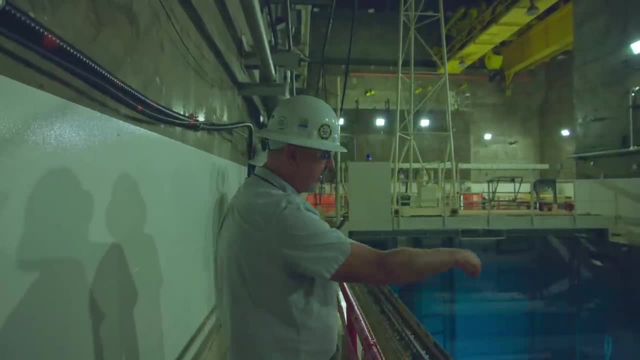 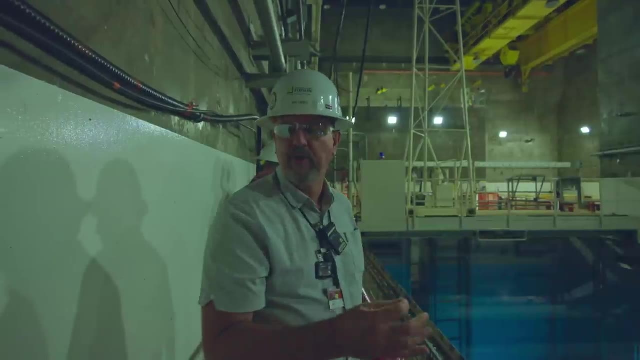 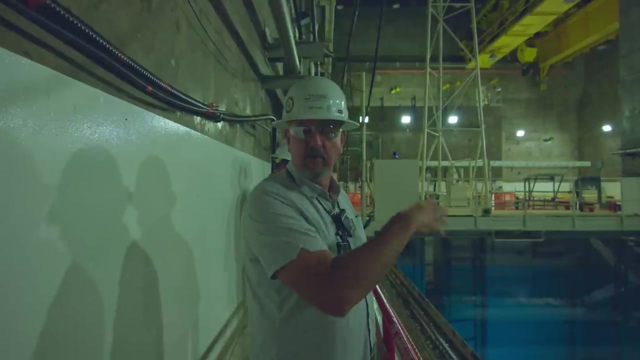 It's empty now, but it would be flooded, just like this pool is, And it would go to a designated location in one of these Racks- designated location in a rack here in the pool- And then we would keep inventory on what fuel assembly from what cycle of the outage went into what location, so that we would have a record of that. 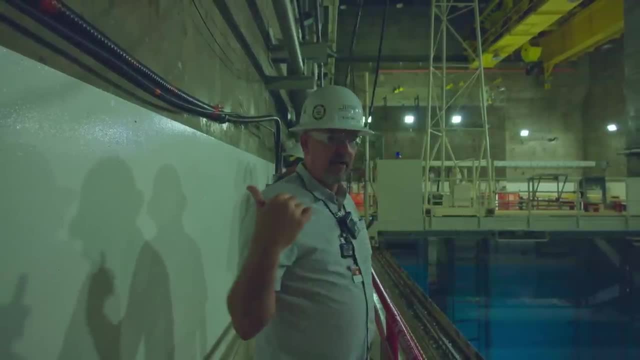 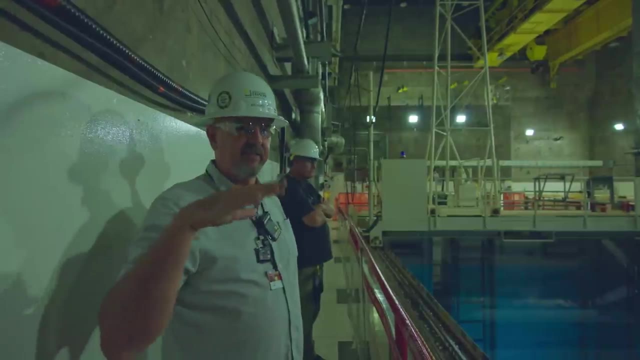 And so right now it's drained down as part of our process. The cavity is flooded over there, But once they're done with all of the cut up activities, then they'll be removing that water as well, And then all of this will be hard to decompose. 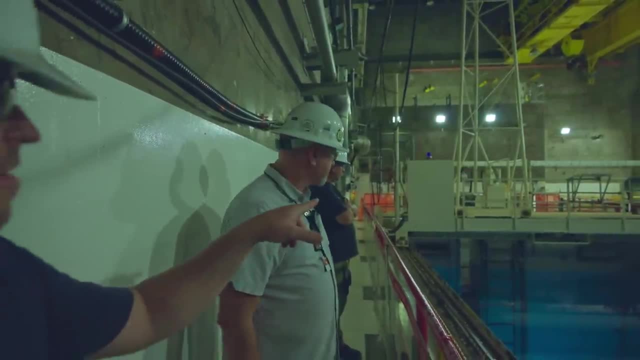 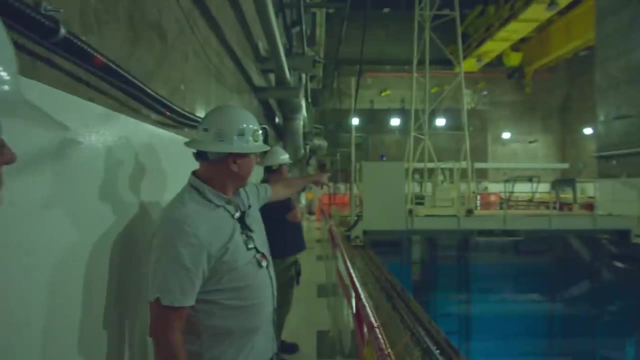 And that's part of our missioning process. Now, that crane right there. essentially, that's what it is, right, It's in tournament. Where did they operate that from? Right on the bridge there, That little white box. if you were to look on the other side, you'd see a console. 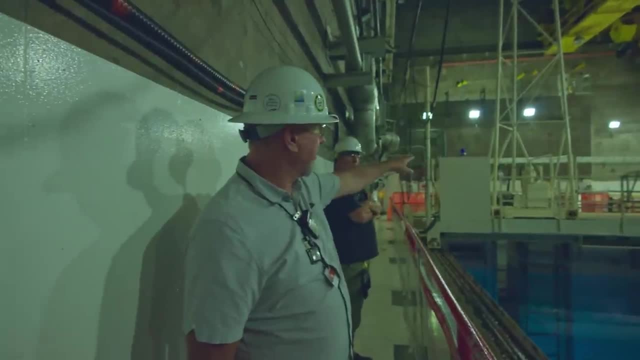 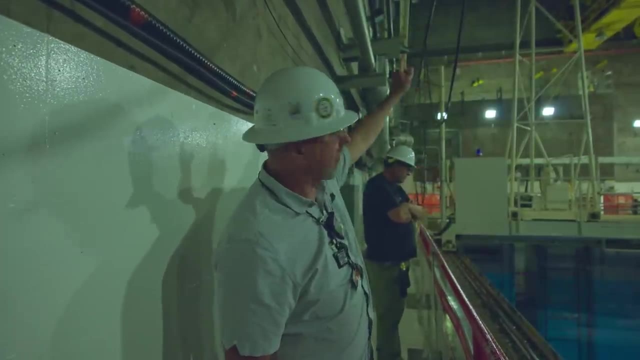 There's like a little chair. that's there. Basically, the bridge operator would sit there and he would. he would operate the hoist, hook up there from that console. It was lower raised- drive the bridge down this way, the trolley that way and back and forth. 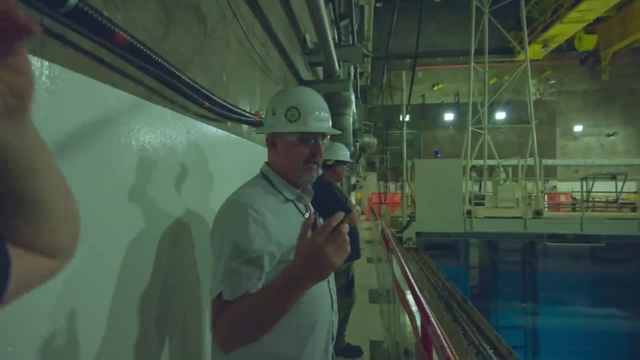 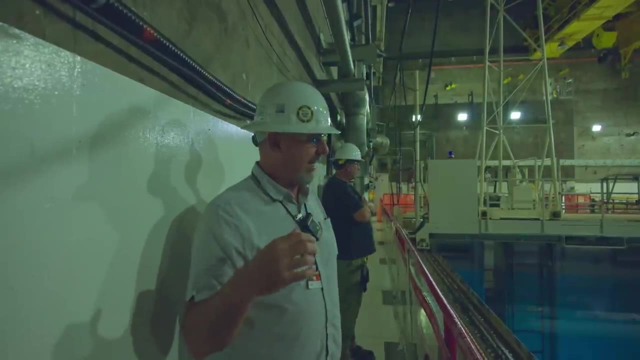 So that you know we have a coordinate system. So the coordinate where they're going to move a certain fuel assembly that they pulled out of the floor during refuel outage might be J72 or something. I don't know. It's probably not 72.. 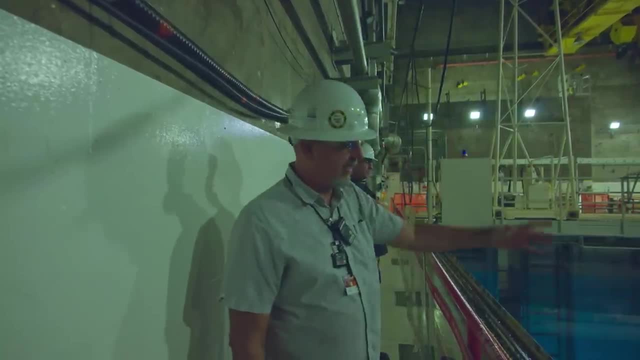 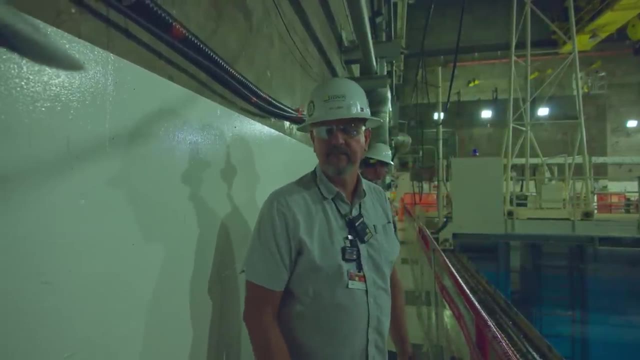 But anyways they would. they would use a coordinate system to go to that location and record that the fuel assembly went to that location and that's it. But is he manually driving it to J72 or is that like they just type it in and it goes there, kind of like a? 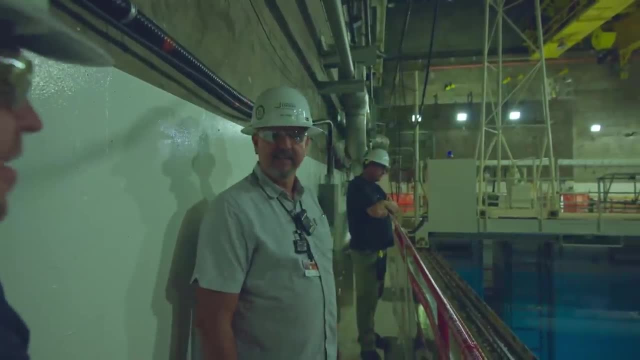 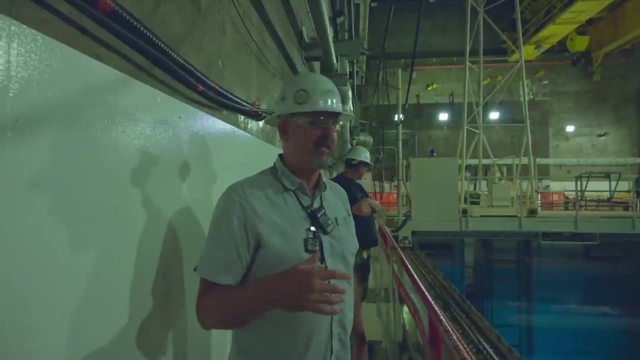 No, He manually drives there. That would be a high stress job right there. no, Yeah, We usually. we have in the industry a contractor group that specializes in operating the fuel handling systems at all the different power plants. Wow, We usually contract with them. 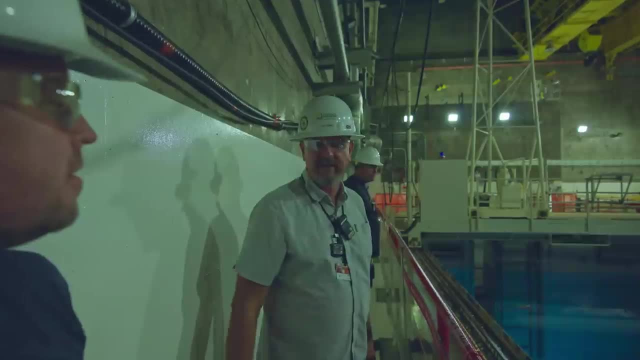 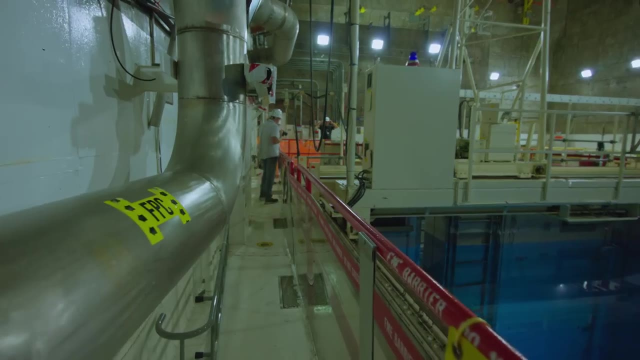 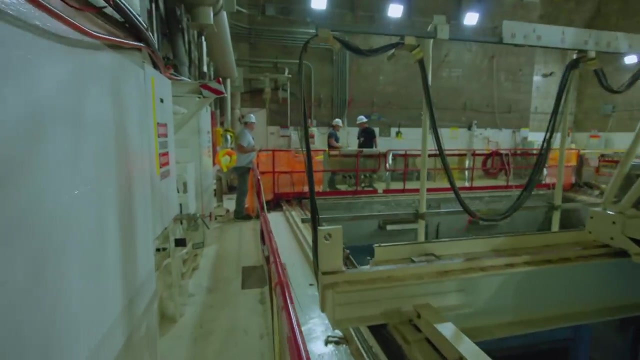 Those guys. they go from power plant to power plant all year long and there's a team of them. They rotate in and out and go around and they're fuel handlers. That's cool, And everybody else is just based on the sales itself. 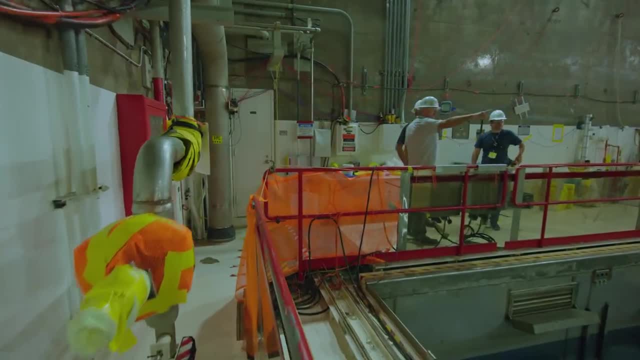 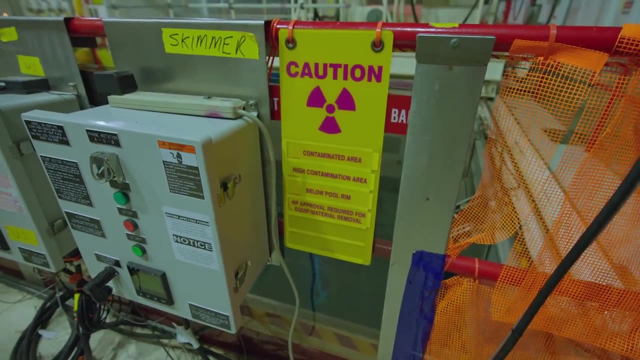 And they go. this guy's gonna fly for four hours to the moon, for a week or even in a few days to the moon. That's cool. You can see from here that they control every HY He will and basically our refueling outages are our cycles of that energy. 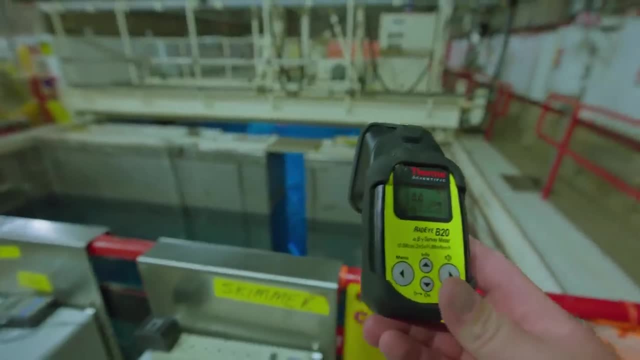 So we have to keep them going. So if you want to keep it a year, that's a huge step, Yeah. But what I mean is, if you have a lot of actual work that you're in, you're not really sure how you're gonna do it. 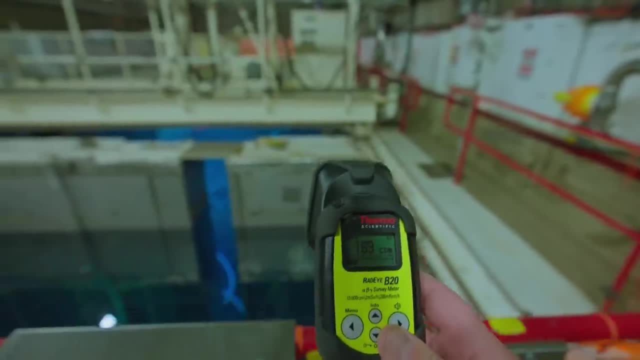 That's true. That's where your five-year period will end up. You know you're gonna have to have a real good first unit with your three years of work. ALF, Have a good time, Be well, Take care, Take care. 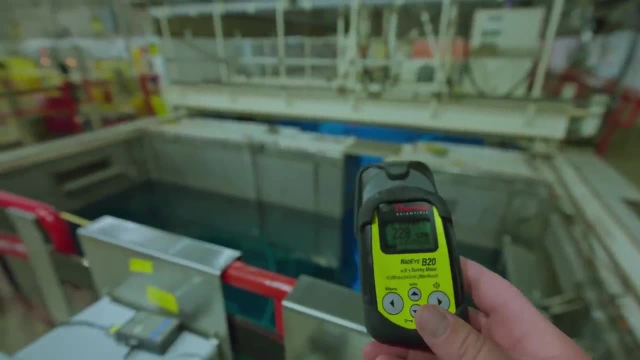 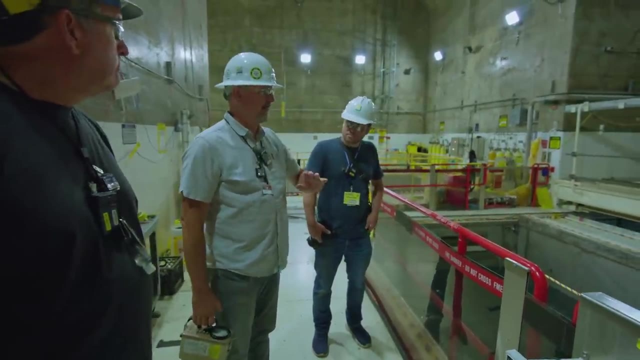 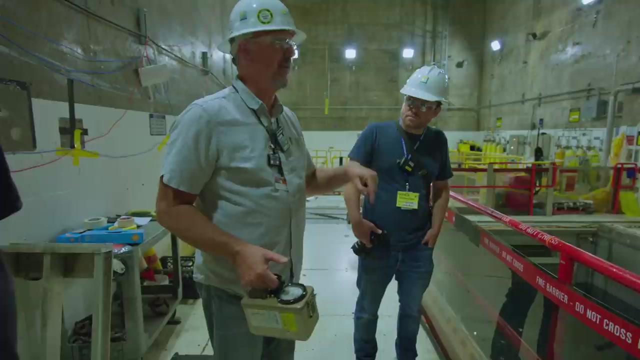 I'll tell you this too. someone might actually ask the question: yeah, but if this pool was loaded with fuel, what would the radiation levels be there? and I can tell you. I've worked here since January of 1990. I spent a lot of my life in this building and the adjacent one and the rad levels. 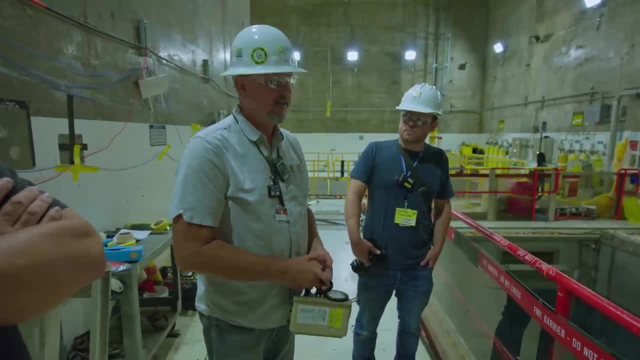 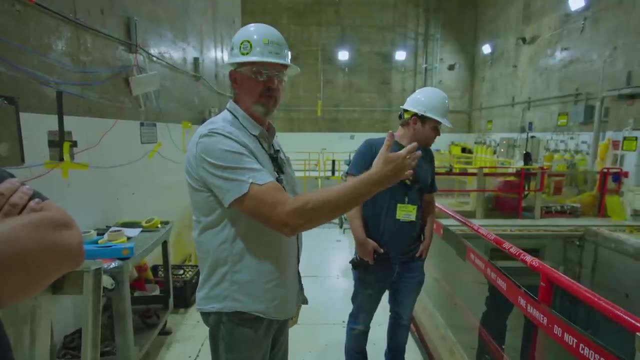 are very similar now to what they were when this thing was loaded up, and the reason is because you have a fantastic layer of shielding right here by design. it not only does the water keep the fuel pool as when it was stored here, but it also provides a fantastic layer of shielding. why is 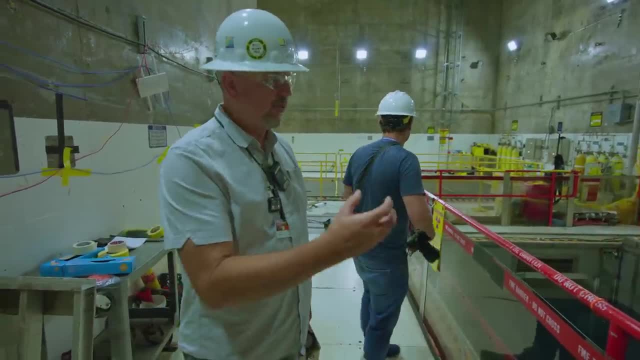 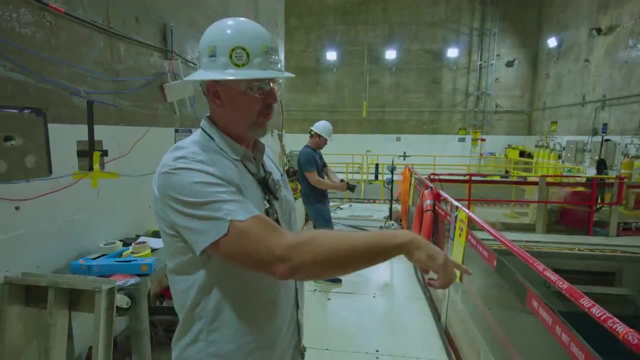 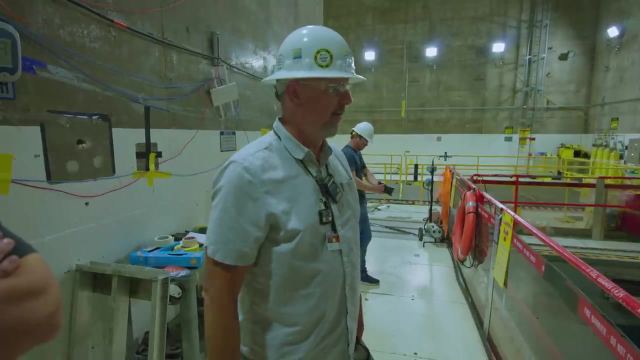 water such a fantastic well it it absorbs neutrons, it absorbs gamma, it deflects. it's a good attenuator. plus, there's such a level here. so basically the top of the racks are roughly 33 foot elevation. we have about 27 or so feet of water, so there's a lot of. 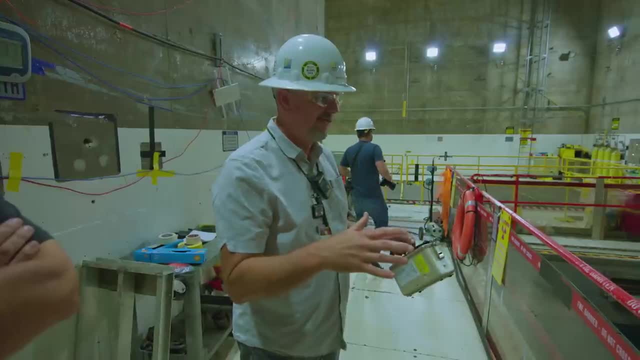 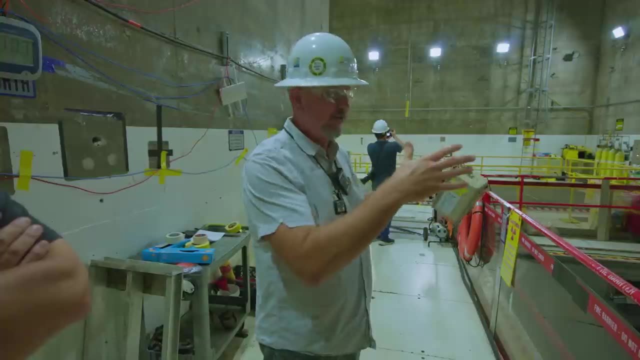 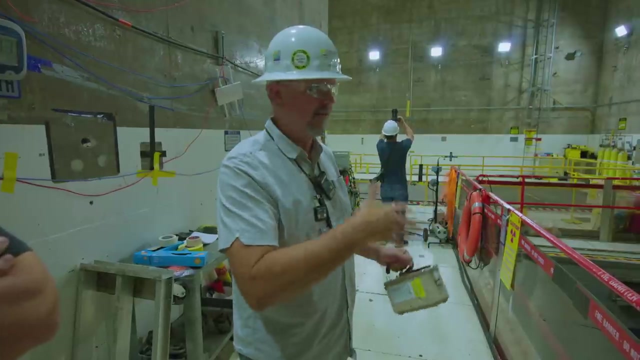 shielding. there there's some thumb rule equations that we use for half value, 10th value layer, in other words, how much shielding it would take to reduce a radiation level down to half of its original value or a tenth of its original value. normally that when it comes to water, that's a few. 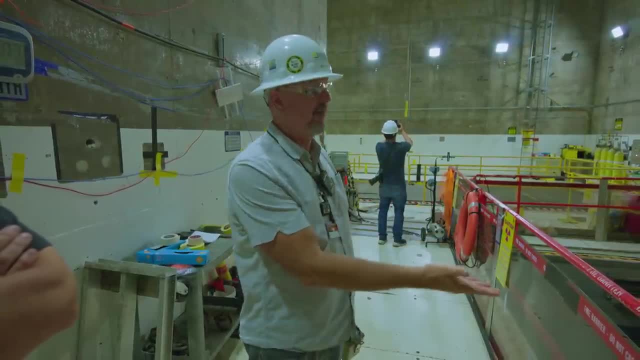 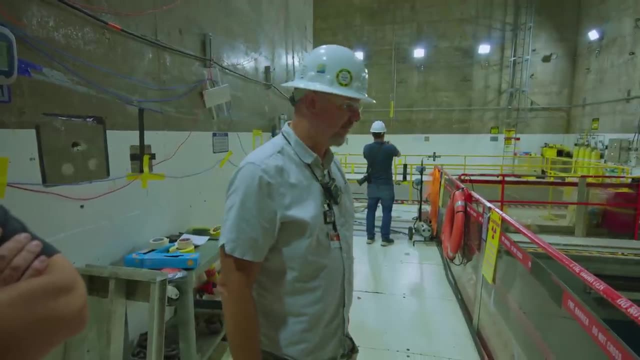 feet. so we're talking 27 feet from the top of the rack to the top of the water. so there's a lot of shielding here to knock those high rat levels down from the fuel assembly. all the clothing that they change out of that's just like that's what they actually consider really low level. 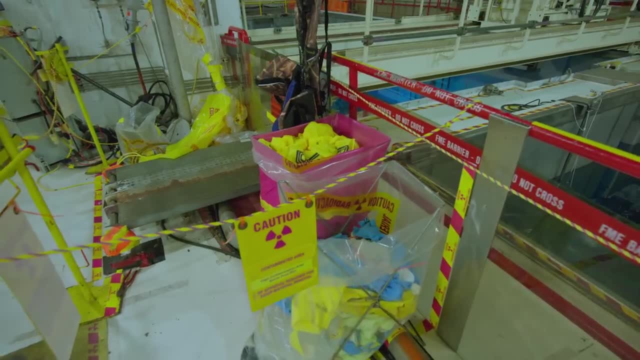 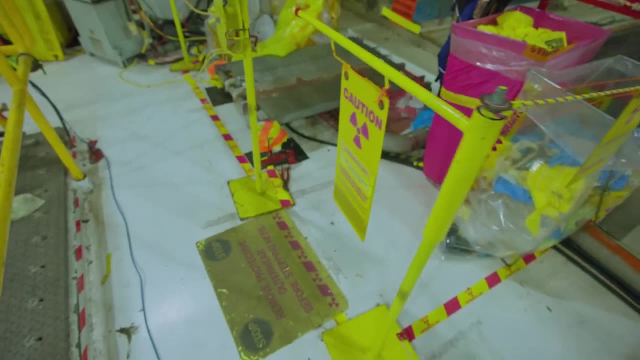 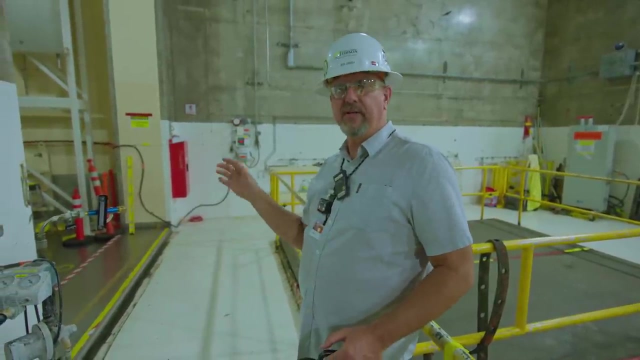 radioactive waste? well, not waste necessarily. there's a if it. if the protective clothing reaches a certain level of contamination on. usually the laundry company that we contract with will monitor all the clothes that we send them that have been used. if it hits a certain contamination level, they'll throw that away. if not, then they'll launder. 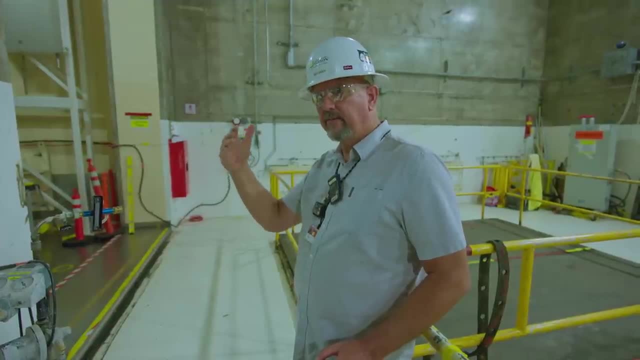 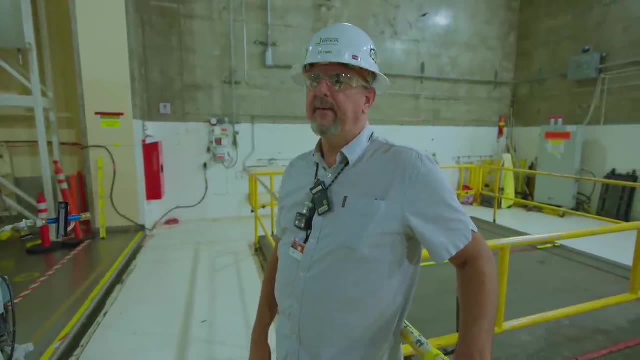 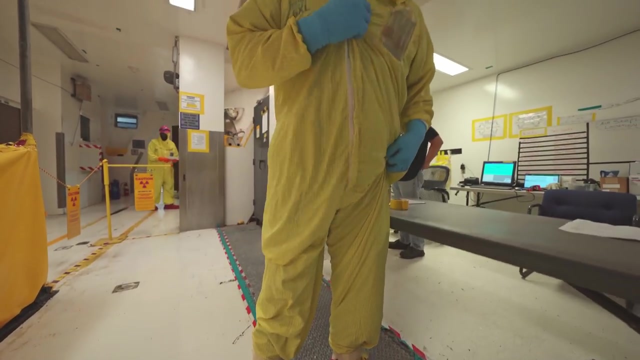 it and resurvey it, and if the if the protective clothing is at a low level- clean level, if you will- then they'll send that back for reuse. the type of clothing that we use is a cloth material that has a Tyvek impregnated in it which is like a rubberized material, so it's, by nature, the fabric. 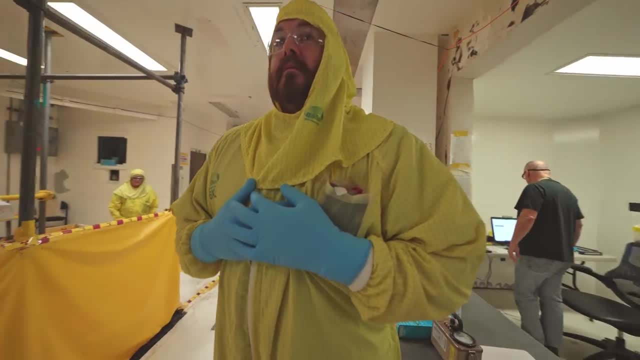 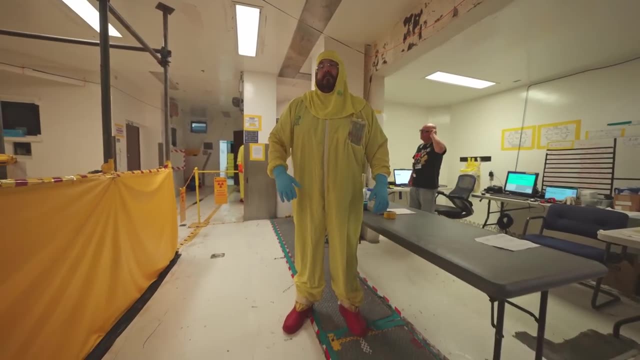 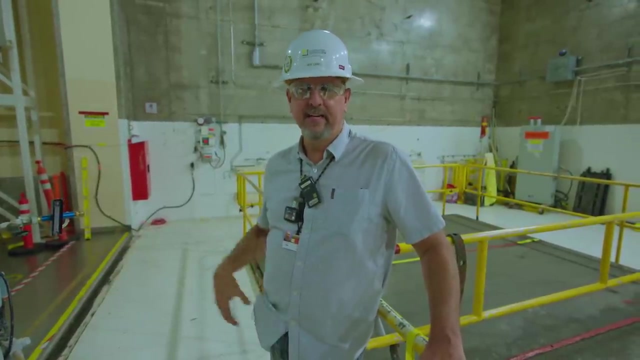 it does breathe, but with the rubberizing agent it also gives it a more, more resistance to contamination. basically particulate matter, so but yeah, it could be that a worker is putting on something that has some very low levels of fixed contamination on them. that's again why we would monitor them when. 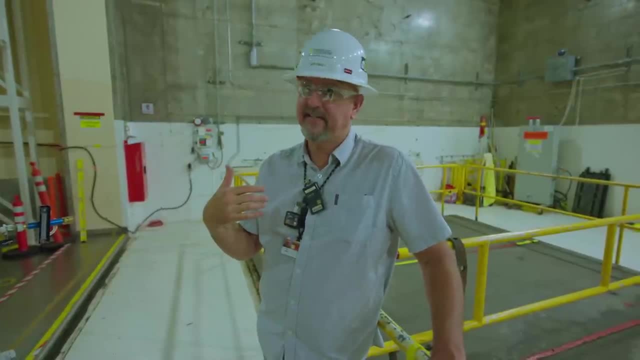 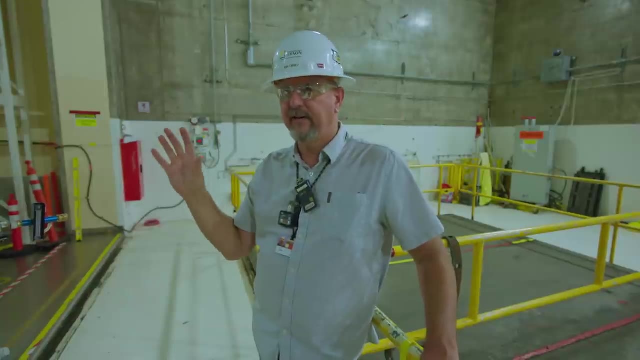 they when they come out of the area to make sure they didn't get contaminated. it could be that they got contaminated from the protective clothing, although it's not usually unlikely. anytime that we send stuff out, like I said, it's monitored before it's sent back and then, as part of our process, we'll do a 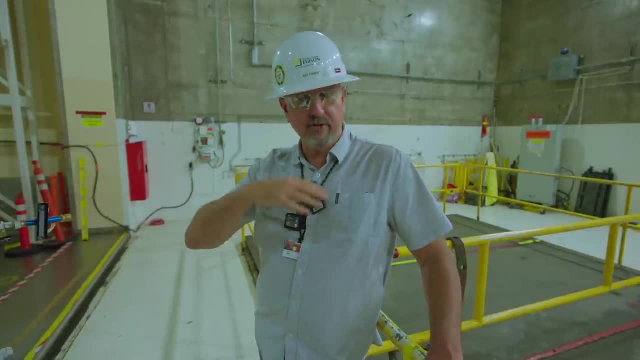 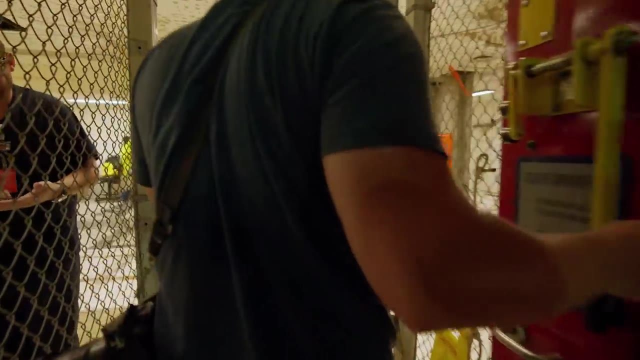 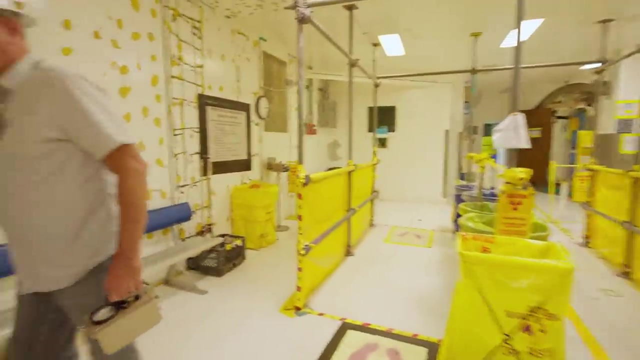 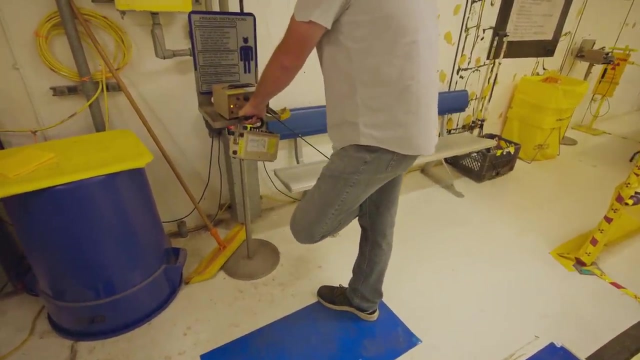 contamination survey on everything that comes back, to make sure there's no loose contamination. so there's no transference. as we left the fuel pool containment building, we had to check our hands and feet to see if we picked up any additional contamination. so the rule here is: 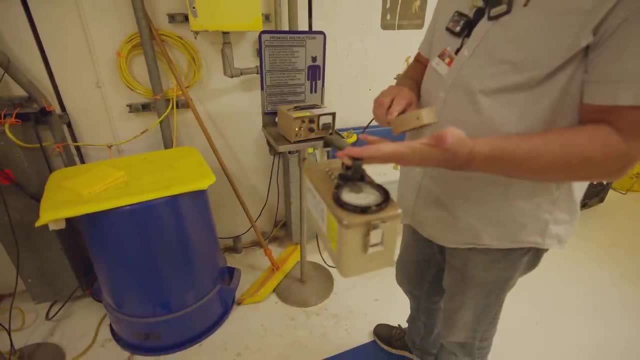 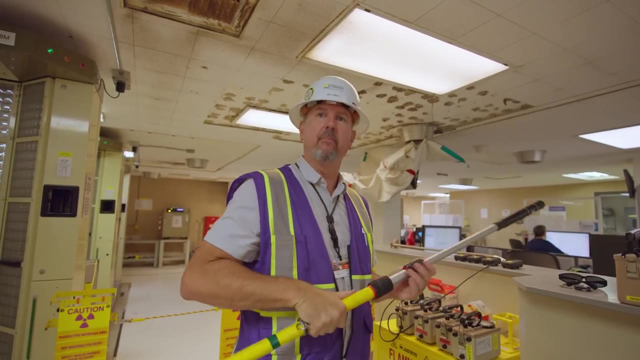 is a half inch away from the surface of the fuel pool and that's where the contamination comes from the surface. no more than two inches per second. but if we need to get a dose rate on something and we just can't reach, like maybe we're going to pull something out of the pool that we were just in. 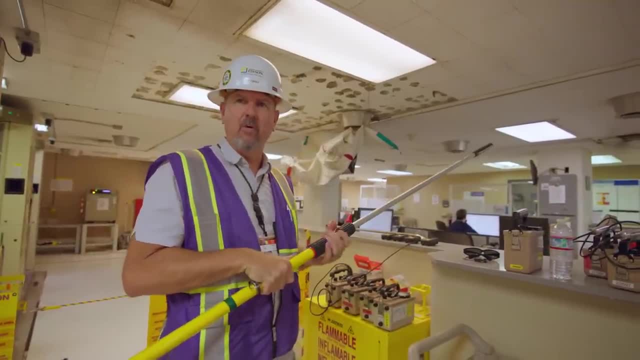 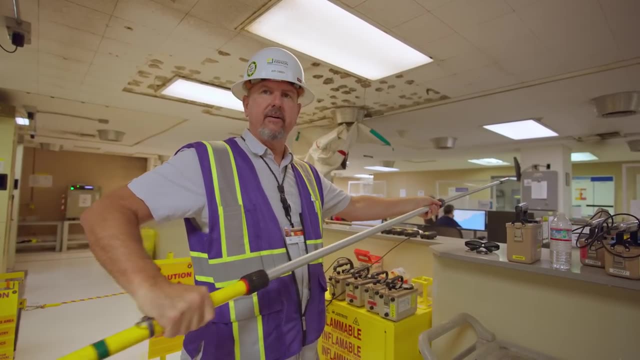 and um, but we can't really reach out there. but we want to check it as it comes out of the water, because it may be hot and if it comes out of the water before we get a good dose rate on it it may, you know, increase the area radiation levels. so we want to be able to check that thing before. 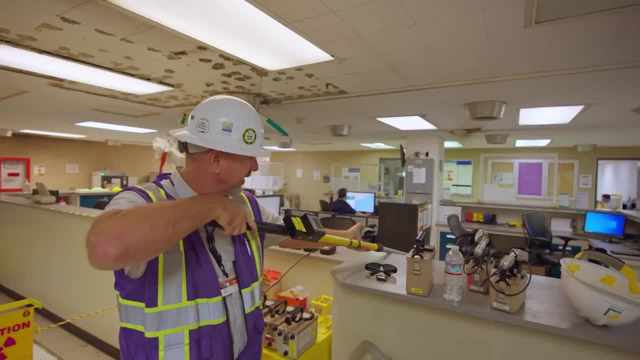 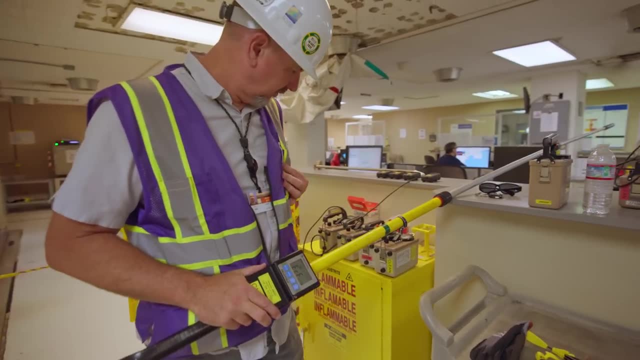 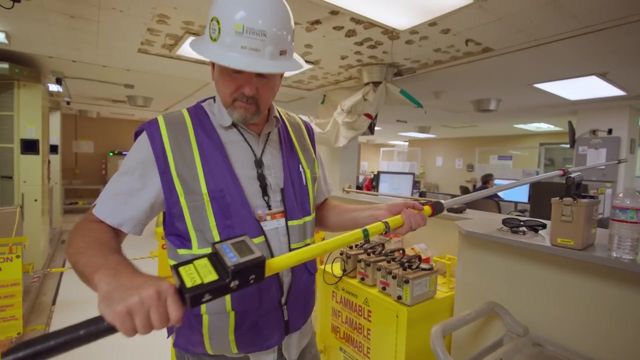 it gets close to us. so use this, because it telescopes way out so we can check those rates, maybe way up in the overhead or someplace far away. so you know what kind of like detectors on the end of there? GM probe, GM probe, yeah, 0.00, 0.01, yeah, but yeah, so what is this? all right, so this is a. 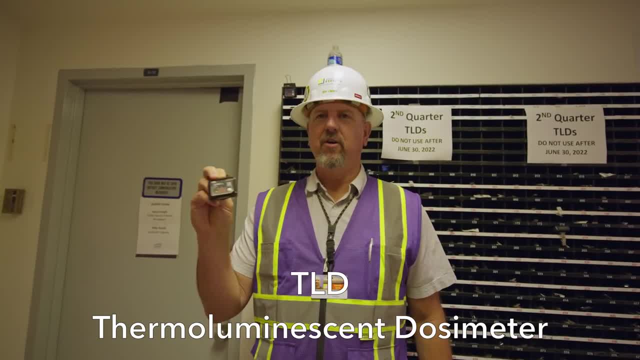 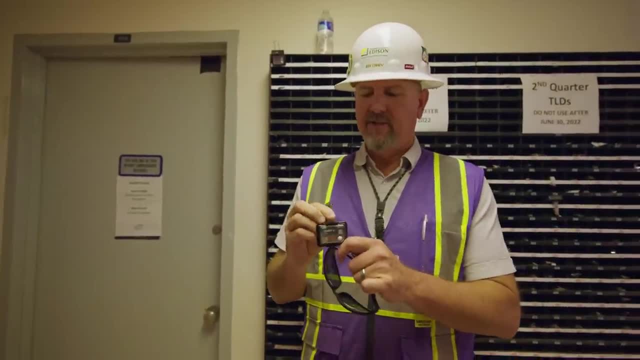 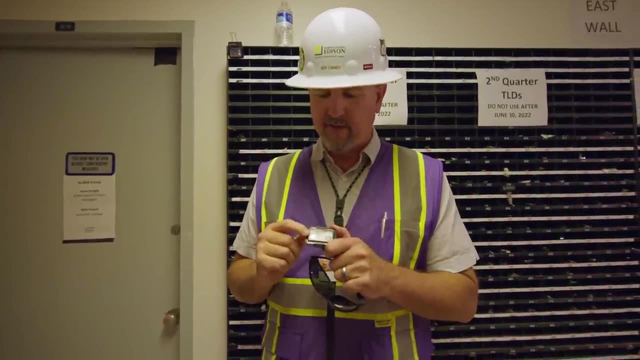 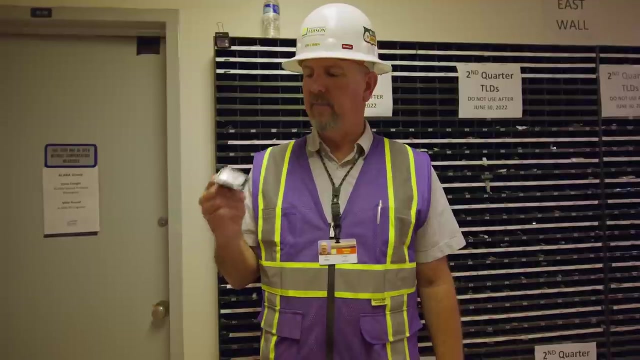 TLD. everyone on site has one of these. every nuclear worker in our, our nuclear infrastructure for the whole country- is issued one of these, and this is our method of determining permanent record of dose, and so basically, this thing measures gammas and also has a window here for betas. these can also be used for neutron as well, if need be, but this is. 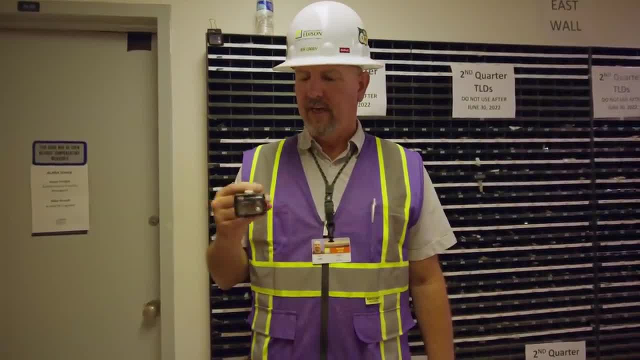 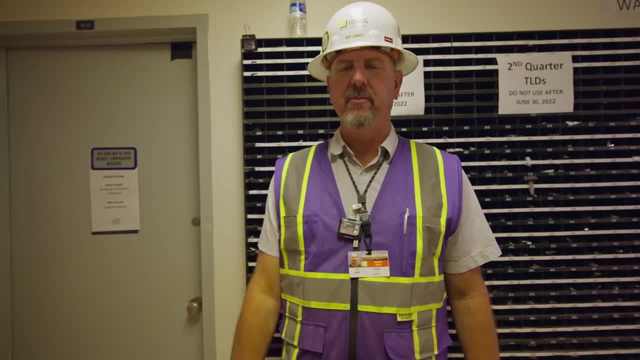 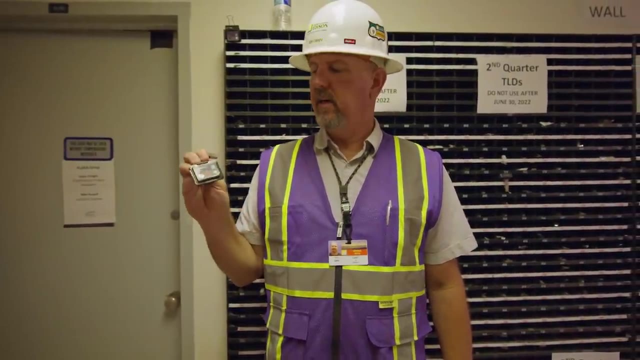 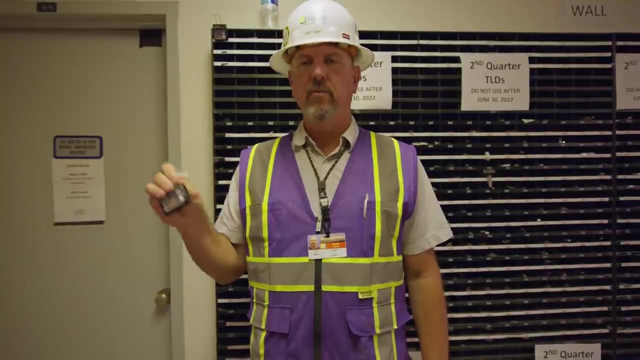 a device that simply measures radiation exposure. every nuclear worker has to have one of these is required per regulation, just to wear it on your chest along with that electronic dosimeter we were talking about earlier. and basically these things get sent off once a quarter, they get read at a lab and that becomes their cumulative dose record. we record all the all of. 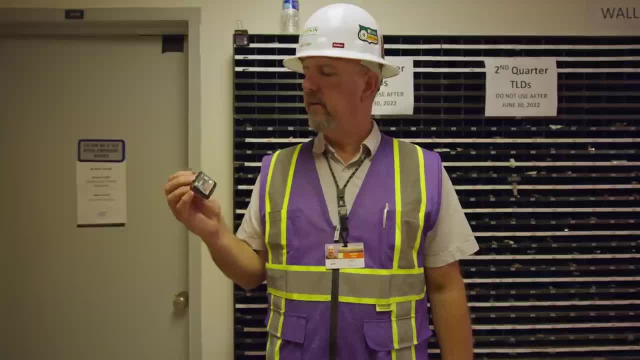 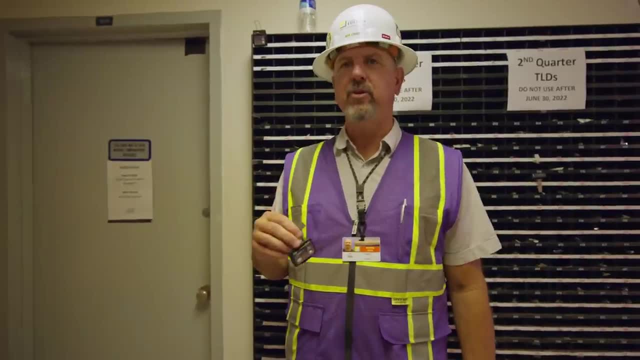 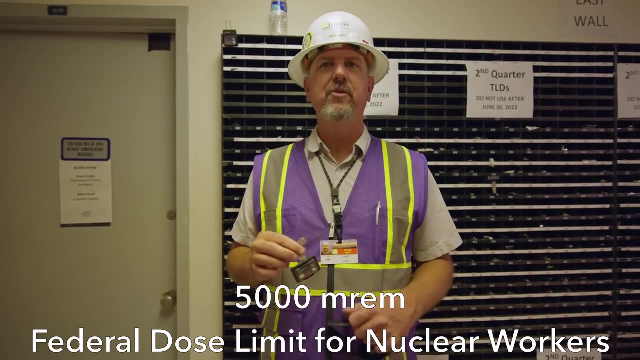 the readings for every worker that's on site, that's being monitored and that record is updated every quarter. so we have an annual total. that annual total goes against a regulatory limit which is five thousand millerim. all the utilities usually use a thousand. they're concerned. 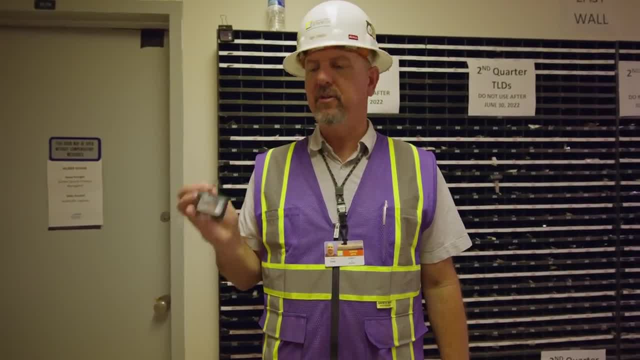 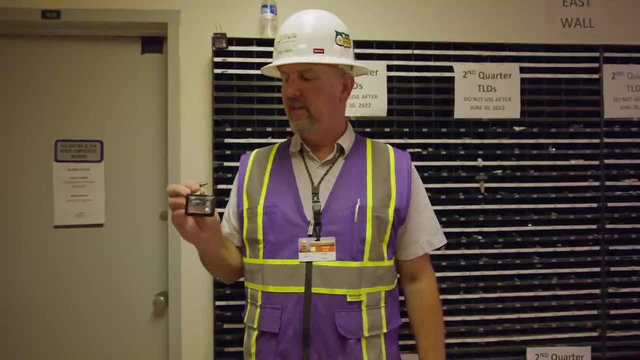 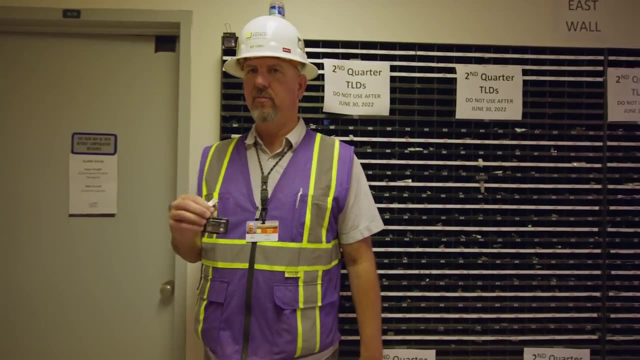 conservative um of uh cumulative exposure and um, it's a rare thing that anyone in the nuclear industry crosses a thousand. there are some examples, but um, but what happens to someone if they cross that? well, it's just more of an administrative thing. there's not like a biological problem. yeah, 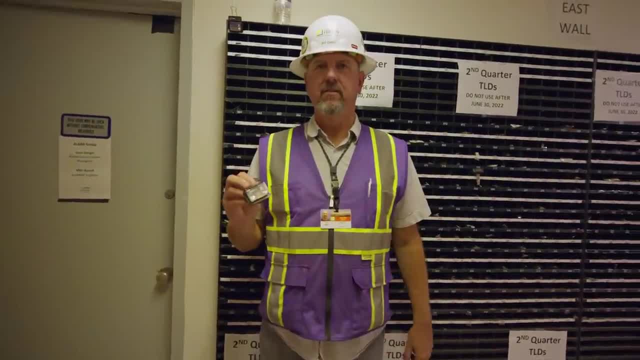 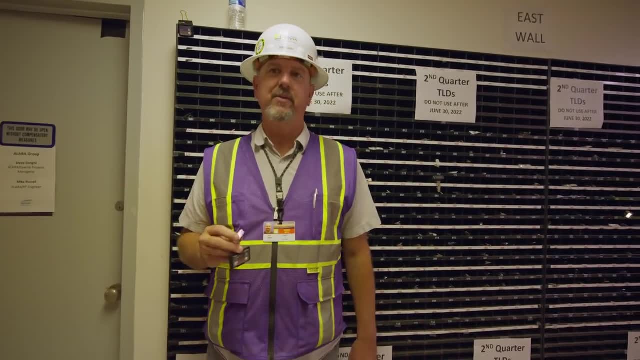 I was just wondering, like, do they just like kind of sit out like until, like, they deem them to be back down? usually what we'll do is we'll give someone an extension if they got a thousand. if they got close to a thousand, we can give them an extension. 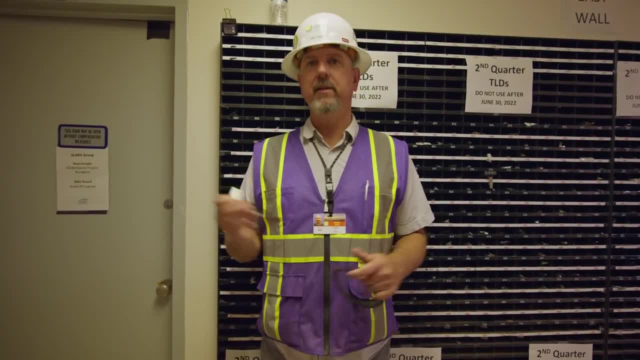 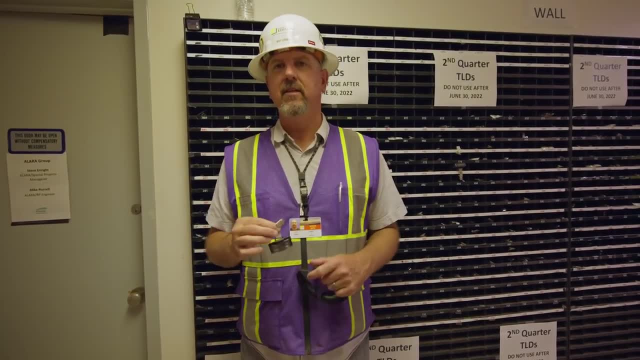 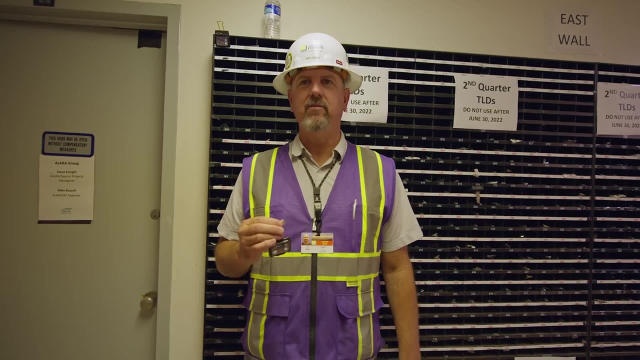 up to maybe 2 000 or 1500 millerim, depending on the site. um, basically, uh, like I said, the government allowances 5 000 miller, so there's a lot of buffer. it's just most, uh plants administratively, they want to control it to a very manageable low level and try to, you know, spread the dose out it. 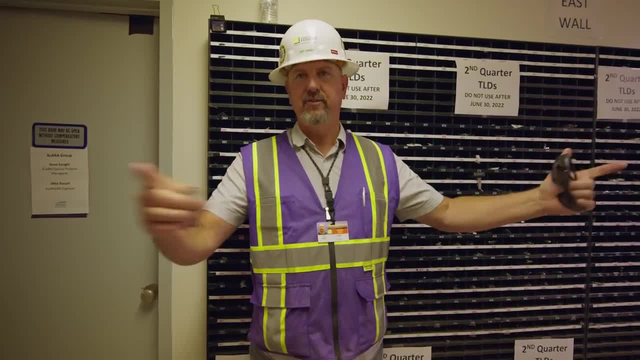 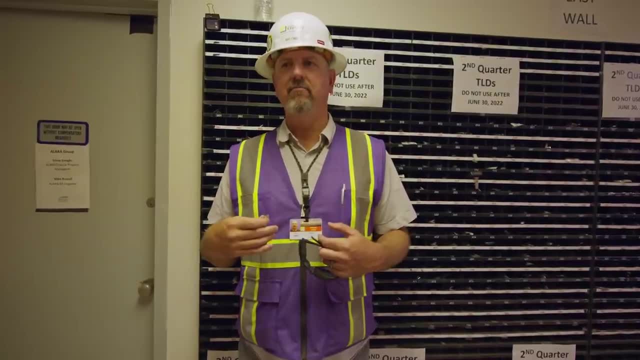 goes along with the lower concept. I shouldn't get all the dose it should be, you know, actually distributed amongst you know several people so that you know one guy isn't, you know, taking in all the the risk. if you will, it's not taking it all for the tuning right. yeah, team's working for him too. 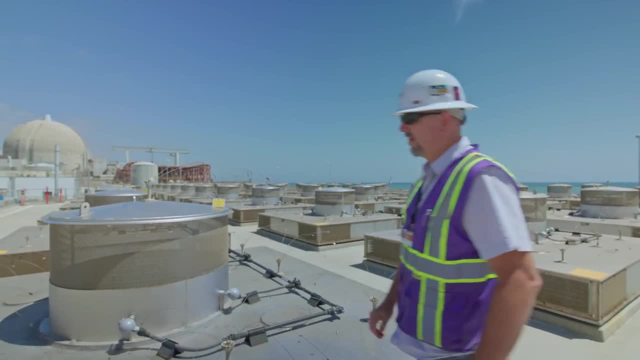 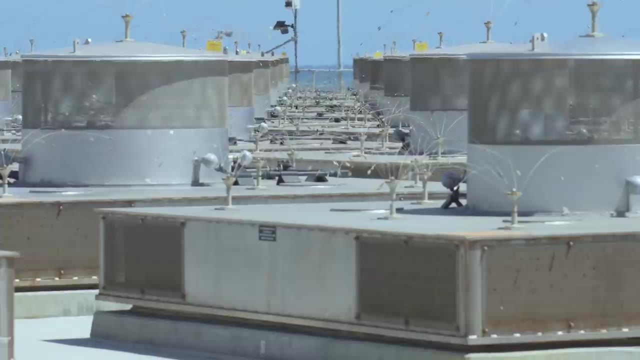 the fuel is sitting six feet down below this level right through a lot of shielding. yeah, so we have a very hot canister, dose rate wise, temperature wise too, as you can see from all the fumes, that lids 35 000 pounds of steel and concrete and rebar and 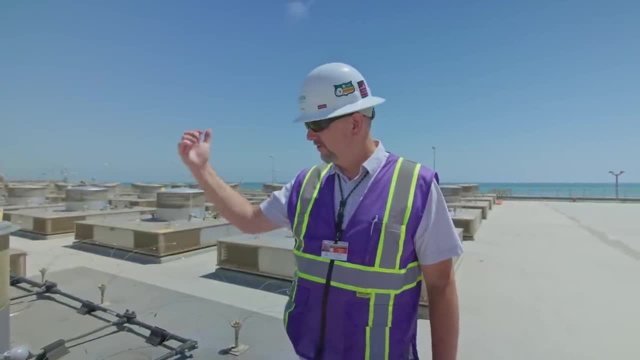 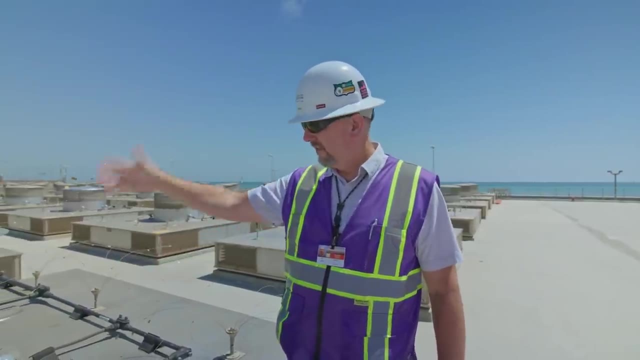 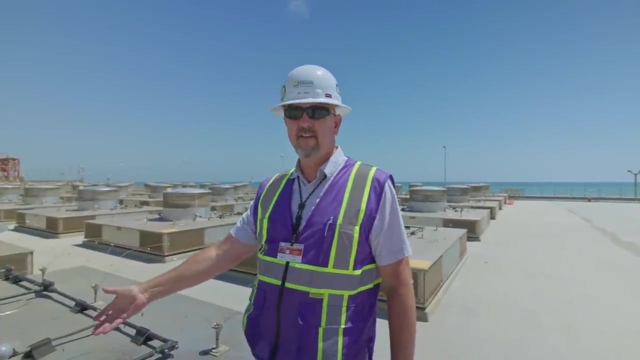 this really is just a convective heat styled exhaust port, and so there's a torturous path that any kind of heat would have to come up through to, to exit the module itself, and so the shielding is pretty robust: the canister itself that the fuel is sitting. 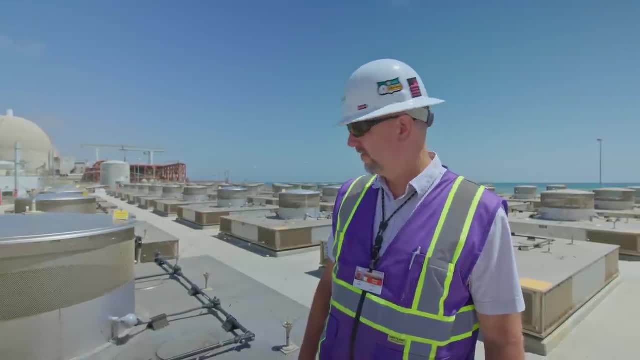 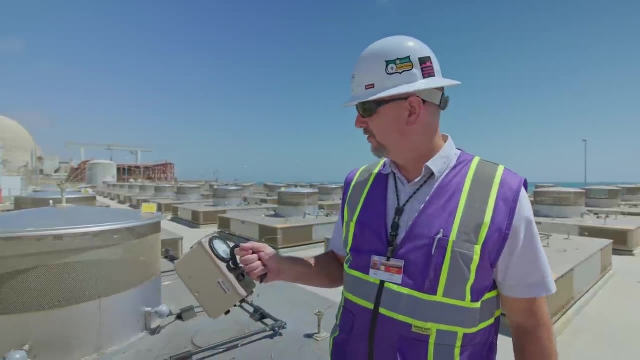 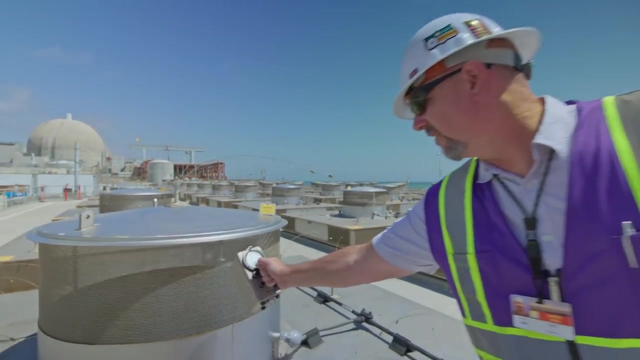 in is very robust, provides a lot of shielding through concrete and steel, and the dose rates are really low. as you saw, our dose rate over here was negligible. less than 0.2 is barely more than that here, right on contact with the module itself, and all the modules are essentially the same dose rate. 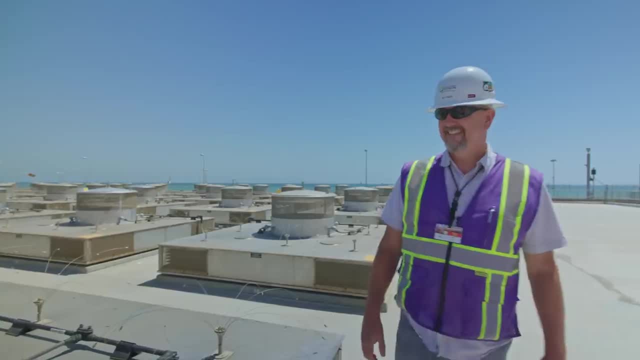 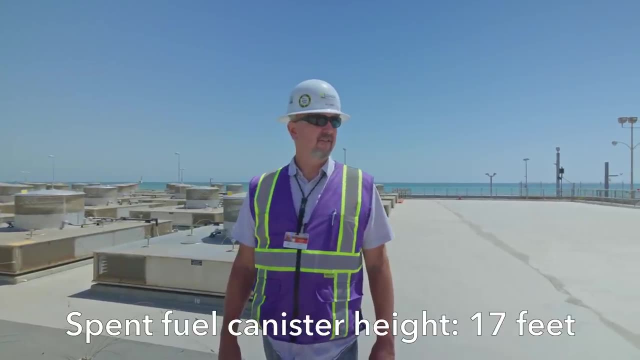 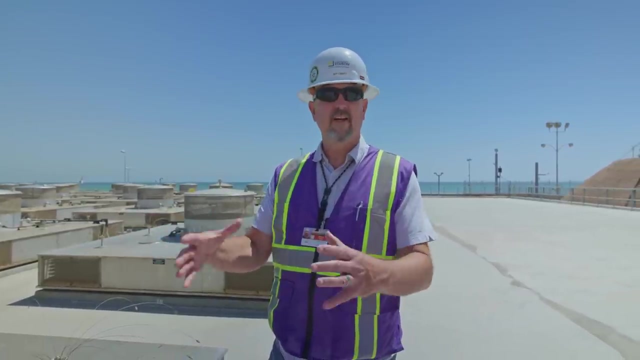 this is a pretty low. be curious to see what you get with your instrument. uh, so now, how tall are these like when they're out, when the the canisters? their canister is 17 feet tall, or 18.. something like that. so you're talking about a structure. that, uh, is a structure within a structure with. 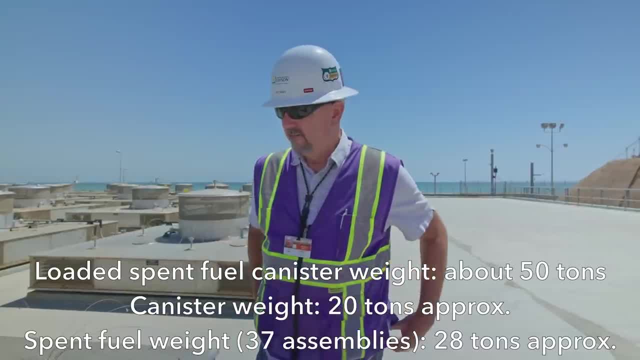 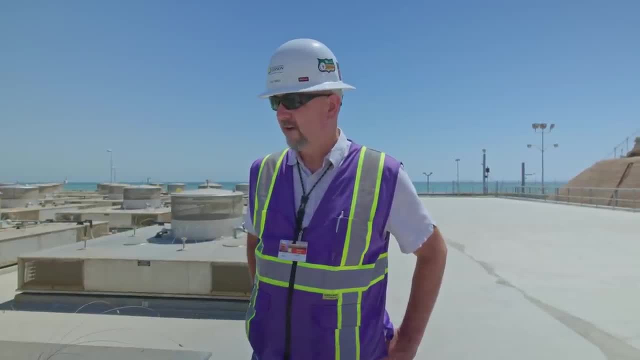 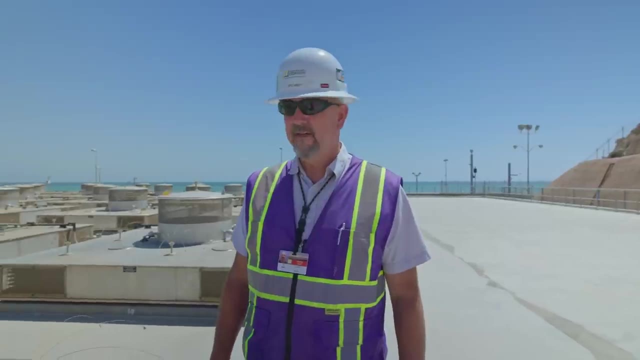 a basket that contains fuel assemblies and and um, so there's a lot of material that goes into the construction of the, the uh storage canister itself. so a lot of built-in shielding for radiation have to pass through before it even gets to the structure of the uh, of the VVM here and the 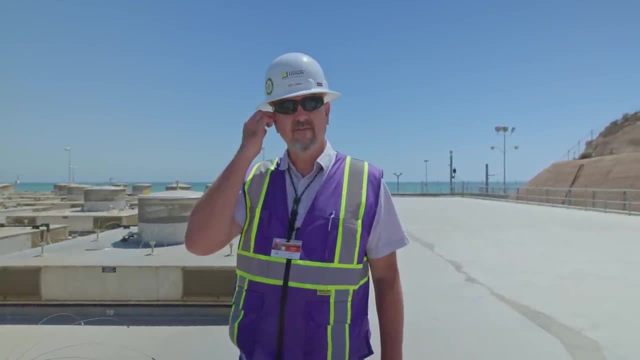 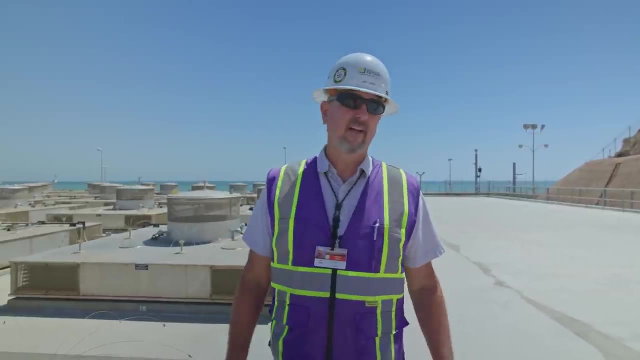 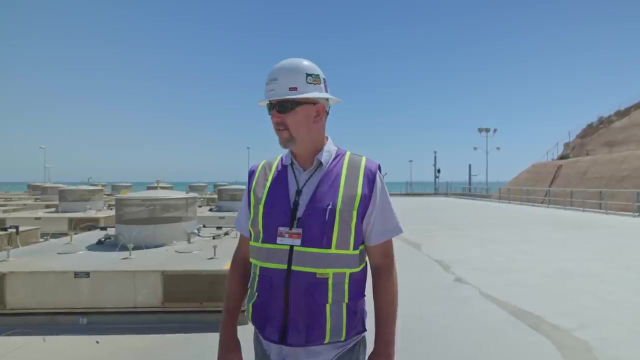 lid and so forth. so there's a lot of shielding that goes into the construction of these things and it's all about, you know, protecting the health and safety of the public, health and safety of the workers from a radiological perspective. those doses down, keep that alarm principle in play. and what's Laura? Laura is an acronym that. 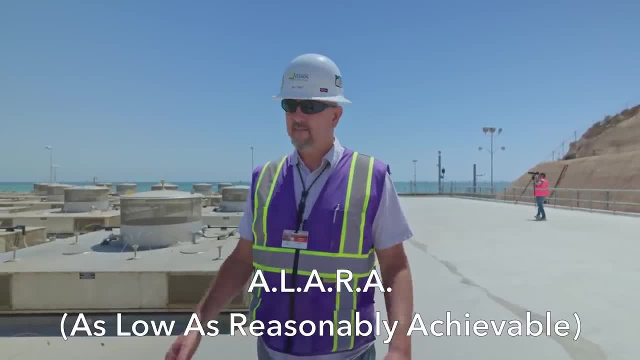 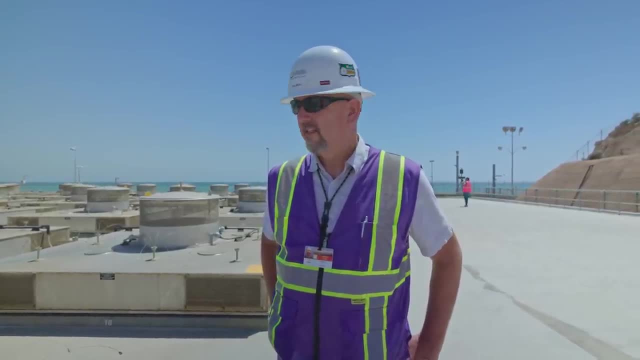 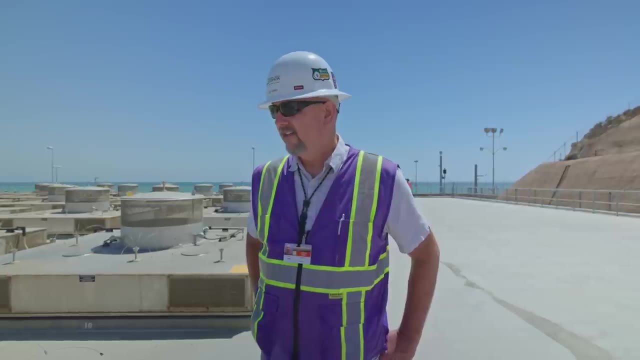 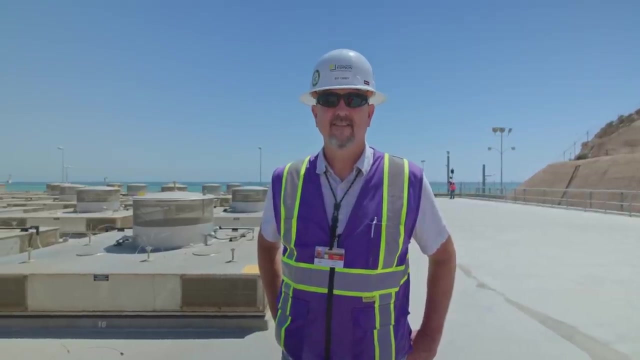 stands for as low as reasonably achievable, and it's all about managing uh occupational exposure using time distance shielding to manage everyone's exposure to the lowest level possible, and that's really. this is uh quintessential to that concept. so now, what would happen if there was a tsunami and water came over this? well, I think the first thought would be that okay, all. 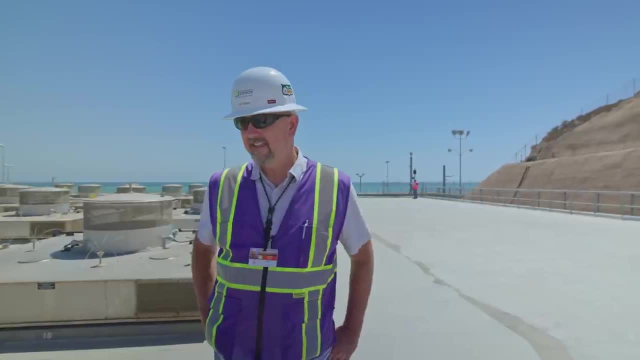 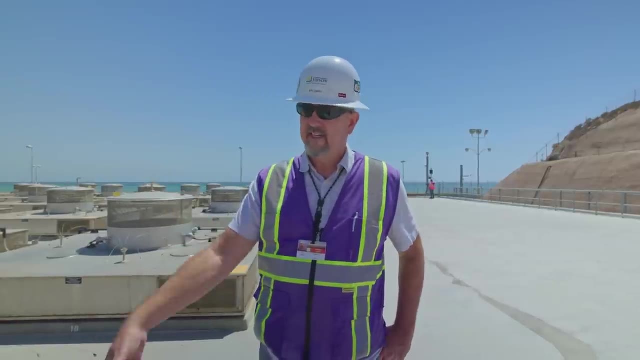 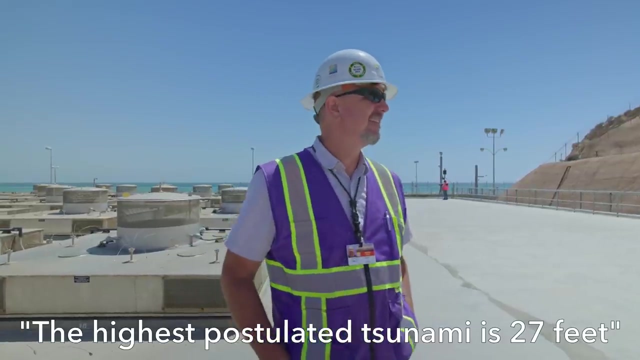 that cold seawater would probably cool everything down. ideally, this thing is is designed to have all air passages free, so that air is free to go in and that convective heat discharge process would would work. it's just postulated. Tsunami is, I think, 27 feet and we're sitting at 32 feet right here, so 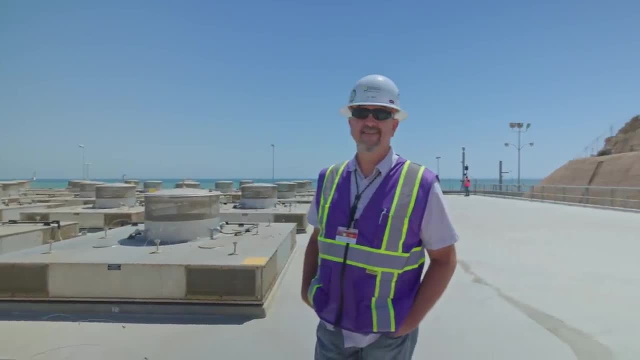 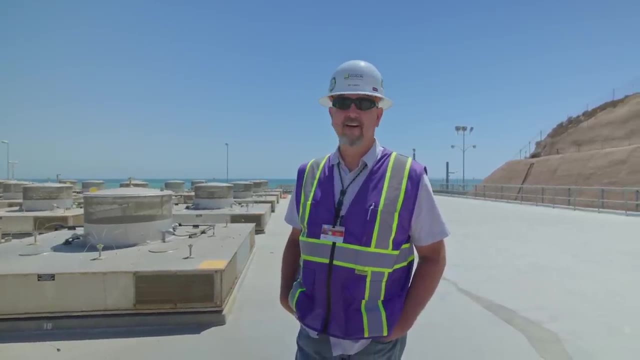 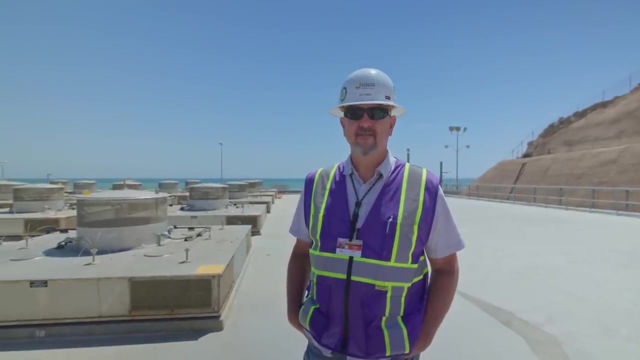 okay, yeah, sounds, sounds like it's all covered. then, well, it's designed, uh, you know, with with the maximum safety factors you know in mind, really. so now there was a thing that, uh, LA Times read about, where they're saying that this was going to be the new Chernobyl, and blah, blah, blah and all. 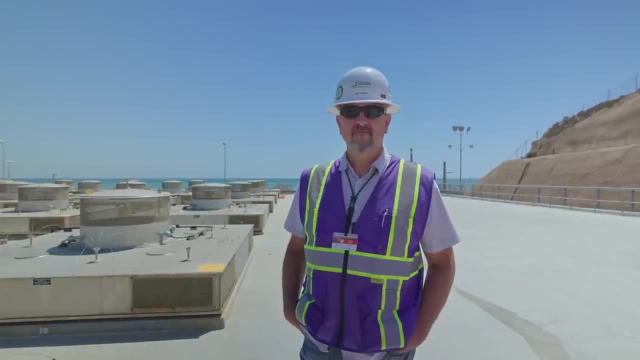 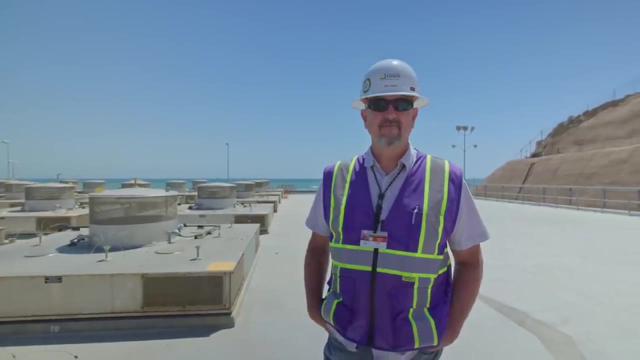 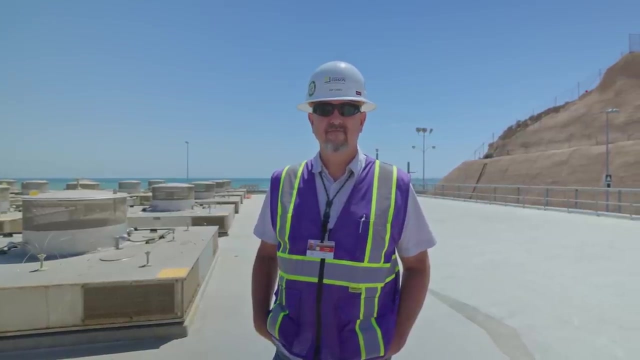 this other stuff and they're talking about, I think, when one of the canisters were being moved in here, they like got hung up on something and you know they're saying that if that would have fallen and you know the very unrealistic, uh hypothetical of it cracking open would have actually done anything. 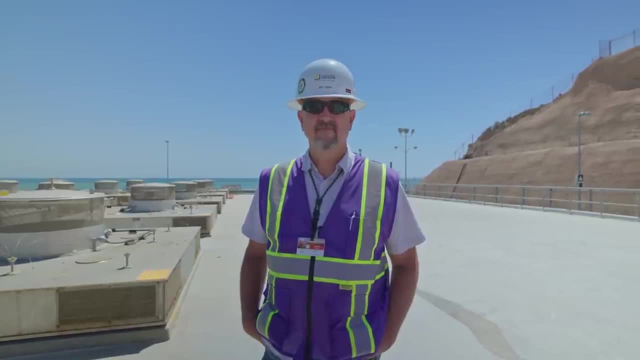 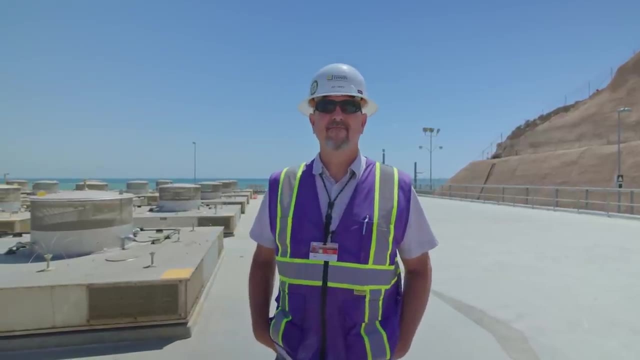 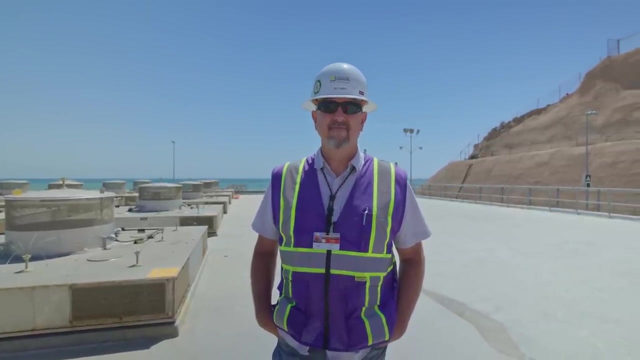 it's like they were saying that that would have evacuated the whole coastline of California doing that and it's like that would have been a local problem. it would have been contained to this pad and to clean up it wouldn't have been something to where it's like all of a sudden it explodes. 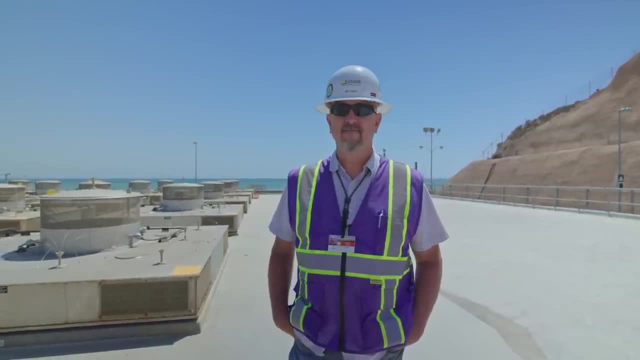 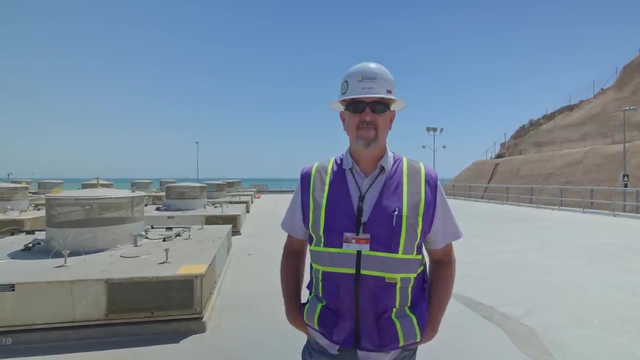 right, you know, it's like that's what they made it seem like they made it sound like that were to happen. it was like blow up and blow. it'd be like a little mini Chernobyl and blow material all over the place, and it's like that's not how it works, that's not how that operates. yeah, 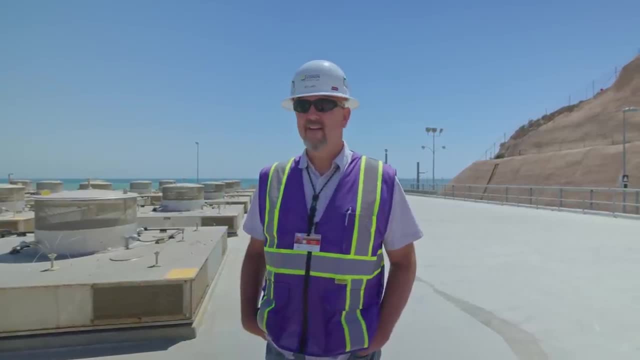 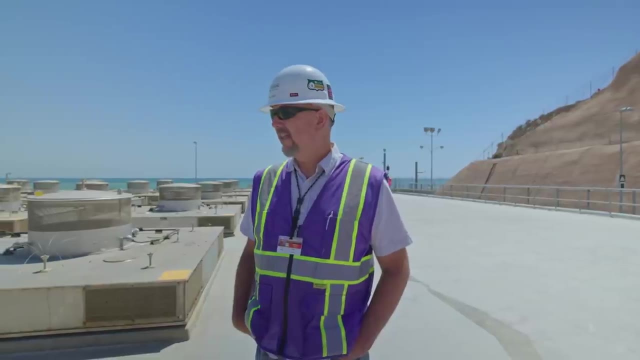 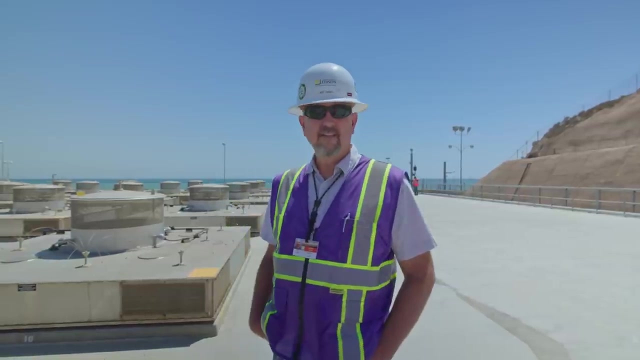 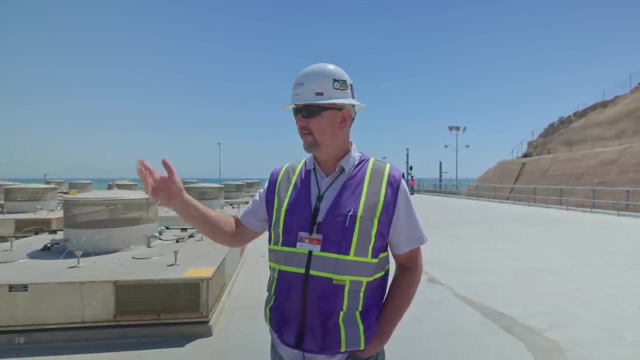 we have procedures and processes in place that are specifically designed and written to uh guide us in addressing a situation like that. in reality, that the canisters are are built so so strongly welded um lids and everything that it's been likely that it would have split apart. if it would have, we would have had things in place, though. 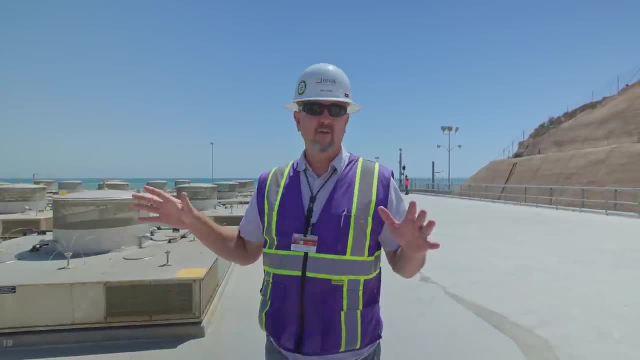 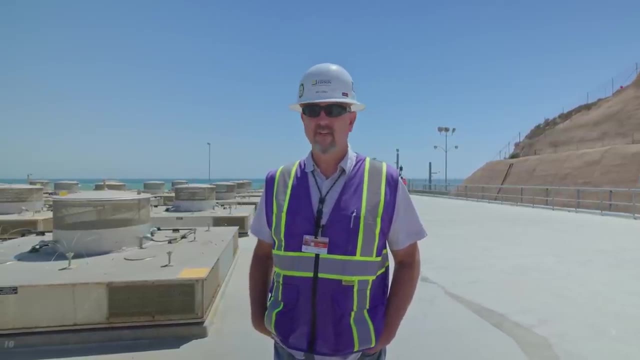 to mitigate a release. I think that at worst, it would have been a local issue where we would have controlled the release of rad material. we would have entered our e-plan, we would have made notifications, we would have put actions in place right away to deal with the event. as far as dose, 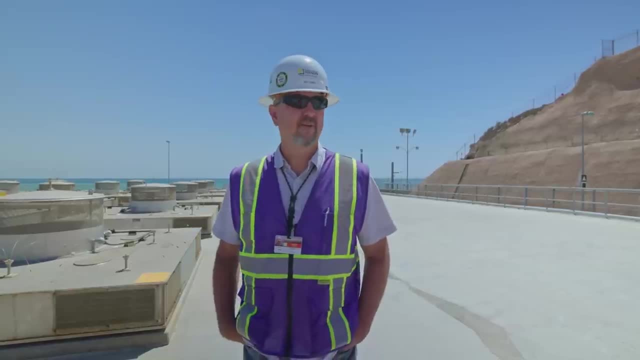 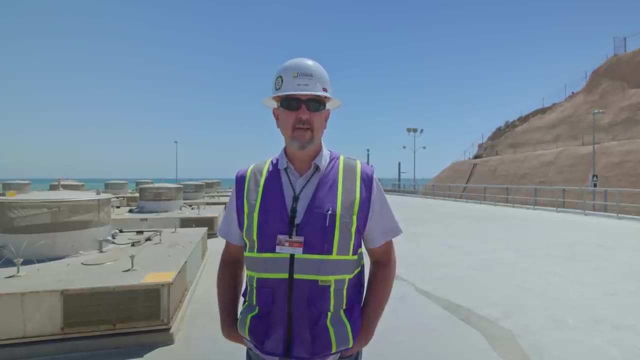 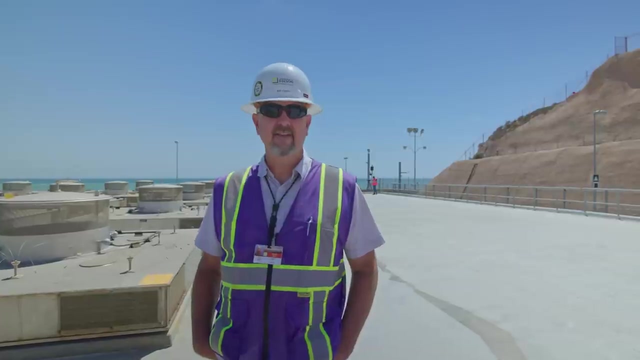 to the public. primary method we'd use would be limiting access. no one would be allowed in here except for mitigation teams, which would then probably be, you know, mostly our own on-site people. and then the second thing that we'd be concerned about would be any sort of an off-site release of a particular or primarily gas from the. 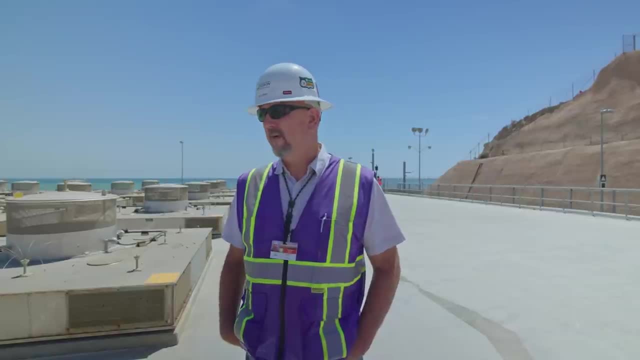 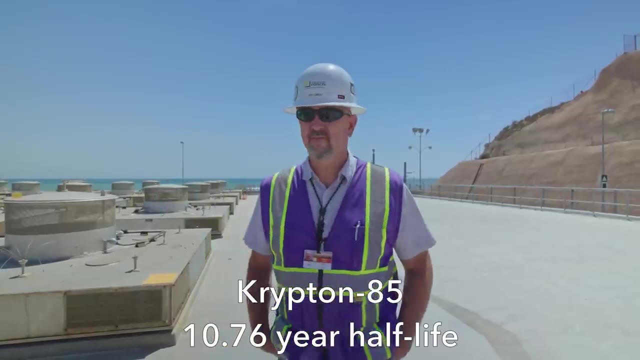 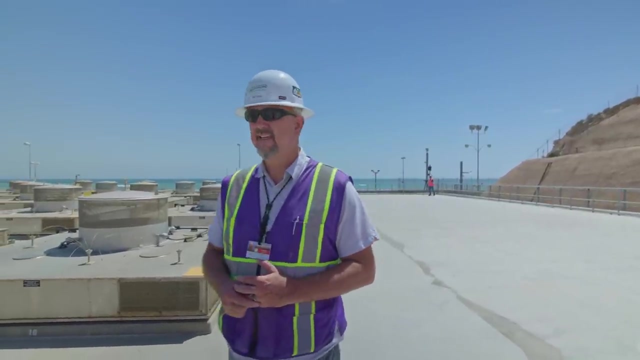 release of the can, if it would even um broke open, but like xenon gas or something, yeah, something like that or some sort of a Krypton gas, you know would be probably the big one. but regardless of that, you know, there's a dilution factor that would, you know, be in play um. 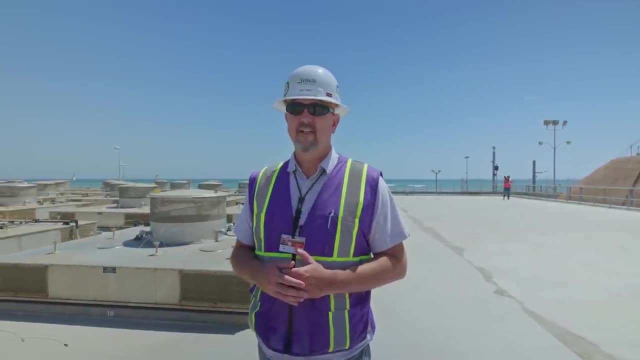 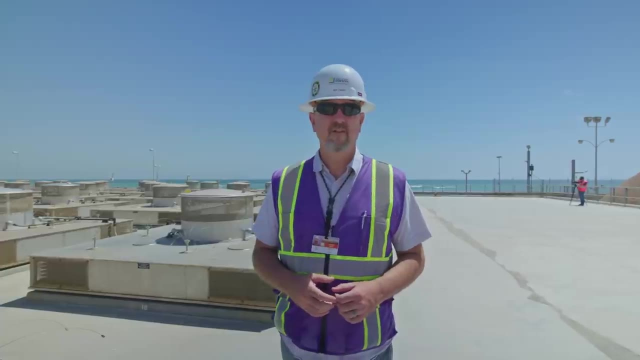 um, wind direction. there's a lot of things that would you know have to be, you know, just right for that worst case scenario to happen, and fortunately we're bordered on one side by the ocean, so there'd be limited concern there. we have, uh, on the other side we're on the the Marine Corps base, so there's. 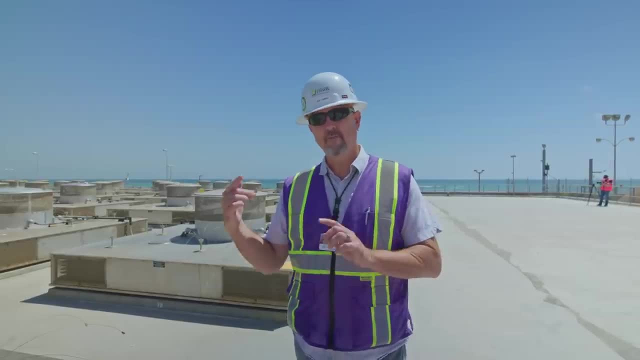 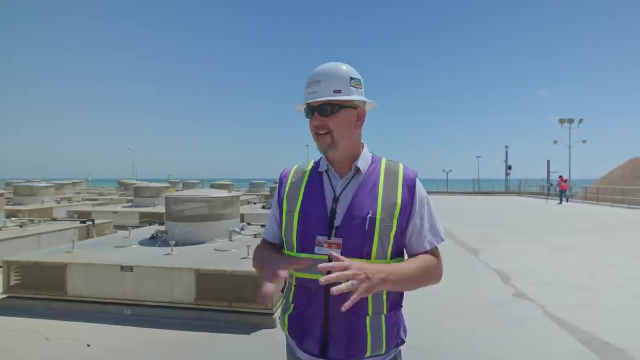 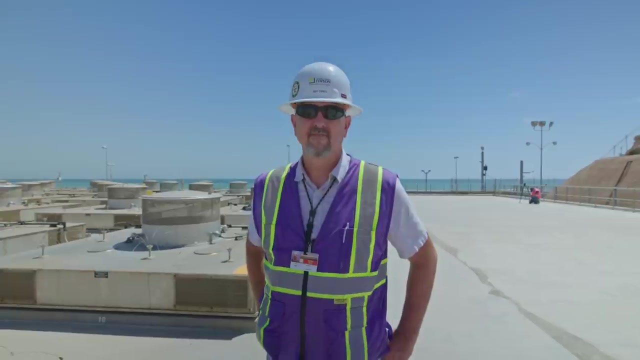 not a big population Zone, it would have to be something where the wind was blowing directly North and you know, um, but you know I I don't think that that would have even been a problem because you know we would have been dealing with locally with our own mitigation efforts. I was just curious on. 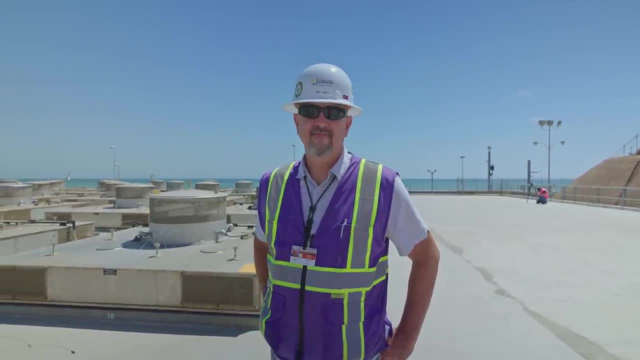 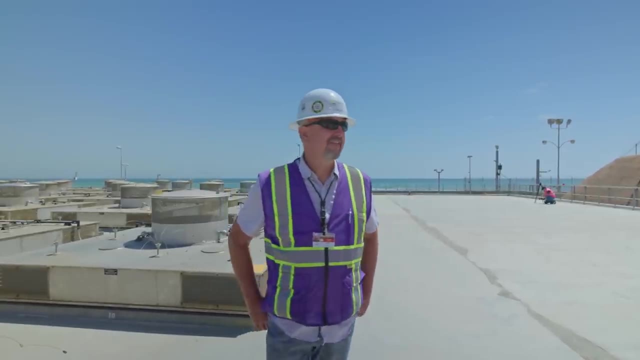 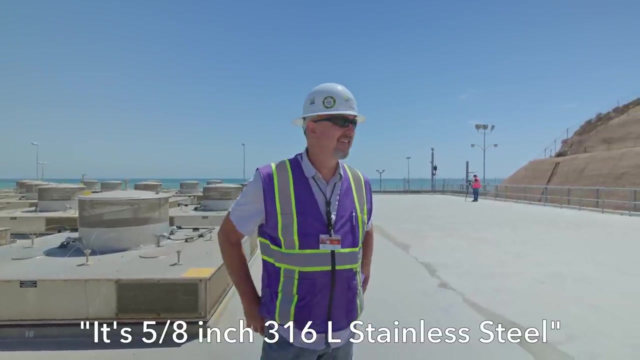 what your take was with. you know about it, because I already had my opinion about it and because it all seemed very far-fetched and what they're trying to sell people. yeah, that I think if you, uh, if you saw the design of the can, it's unlikely, it's super unlikely. I mean it's five eighths inch. 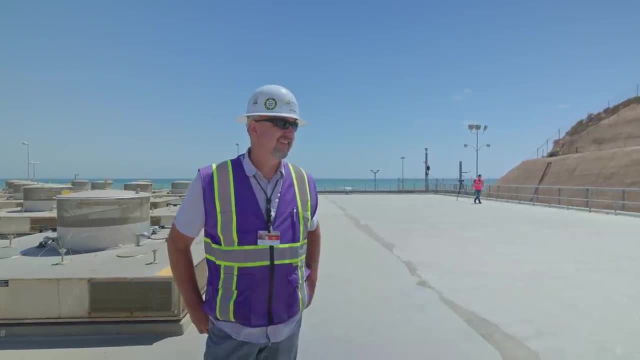 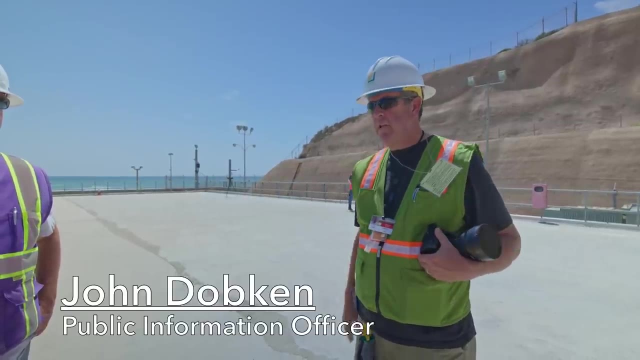 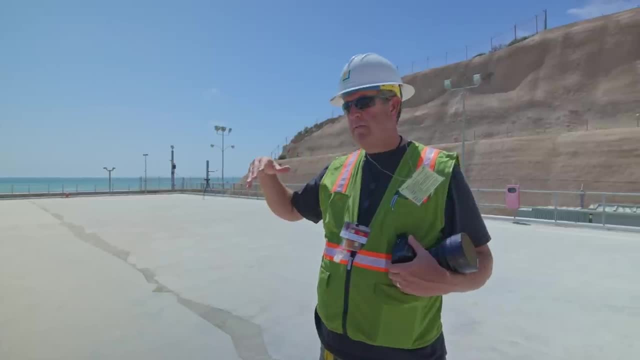 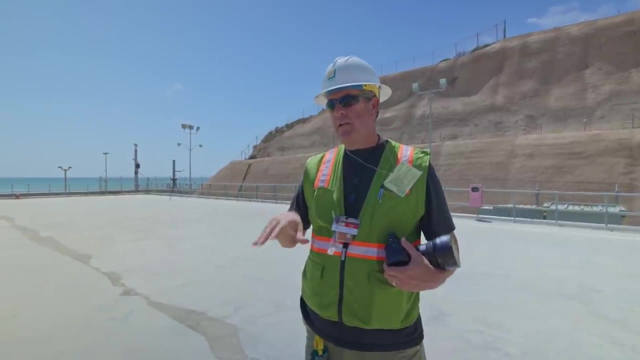 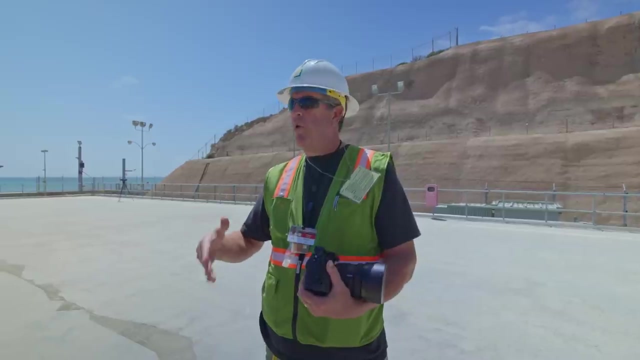 that and and found that, you know, even if it had, uh, you know, could have fallen from from 25 feet and not breached, so you know, obviously you would have had to, you know, um, deal with any damage to the fuel assemblies inside. but yeah, it would have been a very hyper local event. um, we have 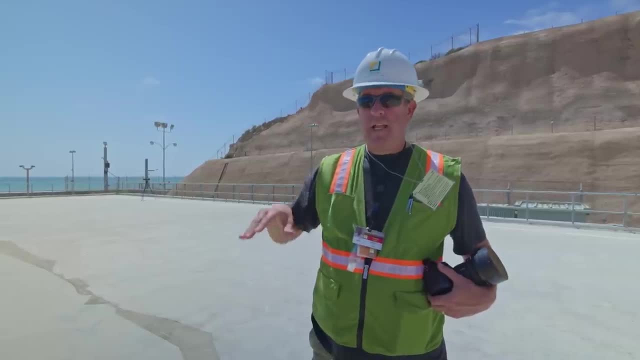 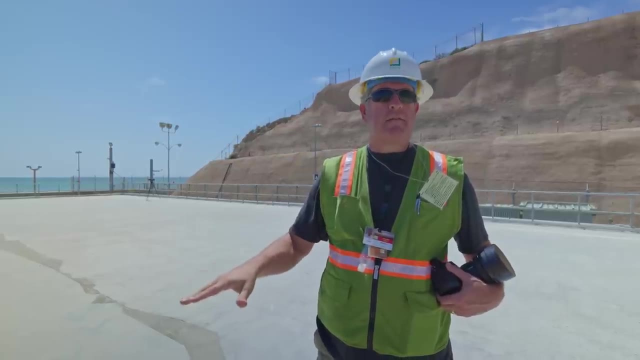 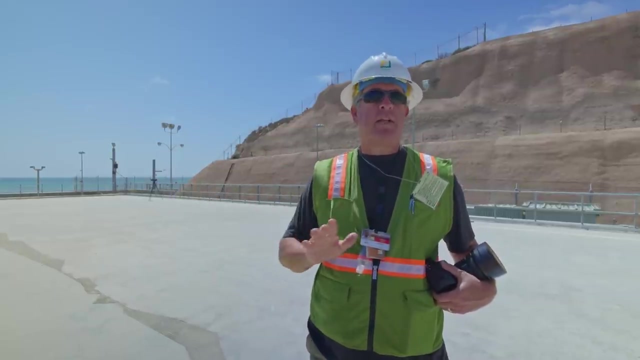 three emergency action levels currently. we had 82 when we were operating and we're down to three now, and none of them involve radiological material leaving the site. so you know, that's why we don't have sirens anymore throughout the community. we don't have a 10-mile emergency planning. 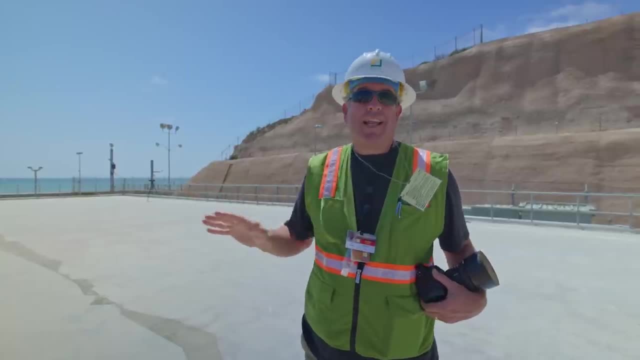 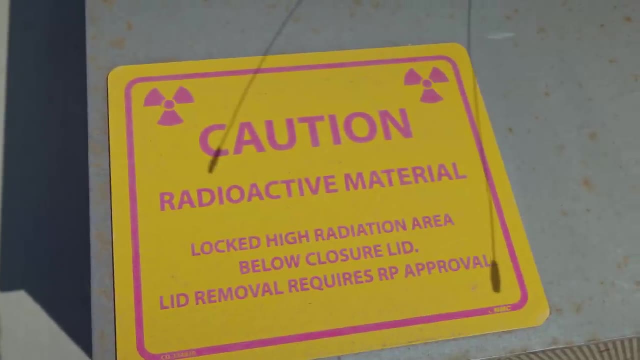 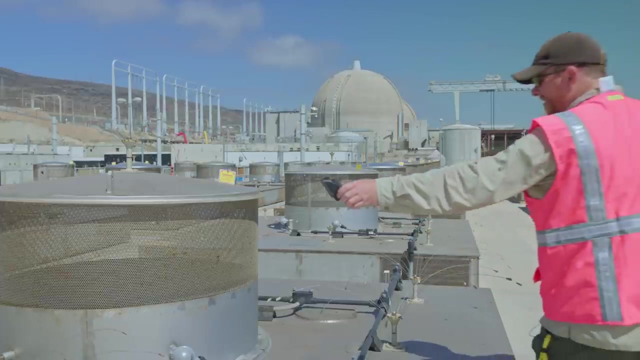 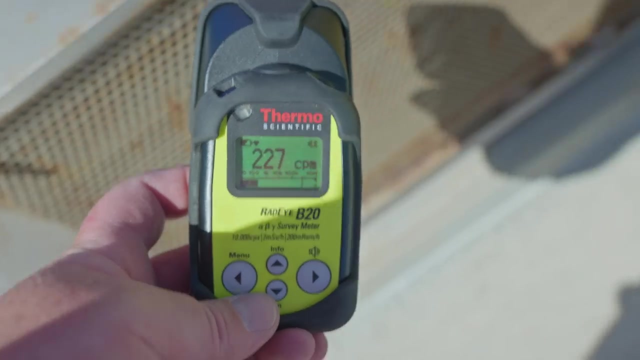 Zone. we don't have any of those things because they're just, they just can't happen. so you know, okay, the level of safety has gone way up, yeah, so now I wanted to walk around and check out the radiation levels myself using my radai. the levels I found were extremely low, especially considering how radioactive 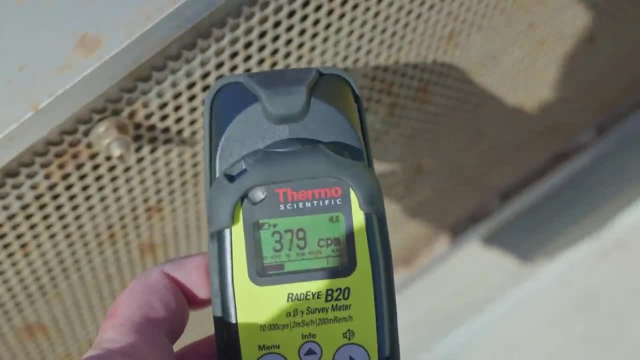 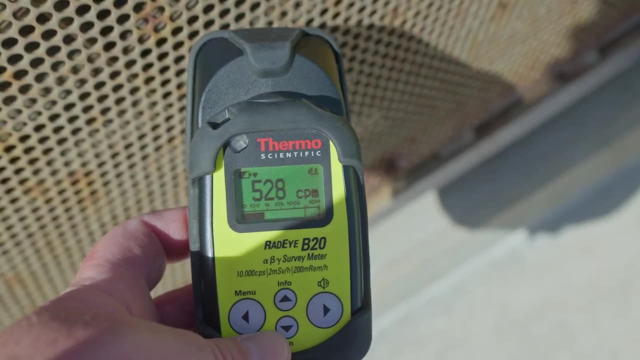 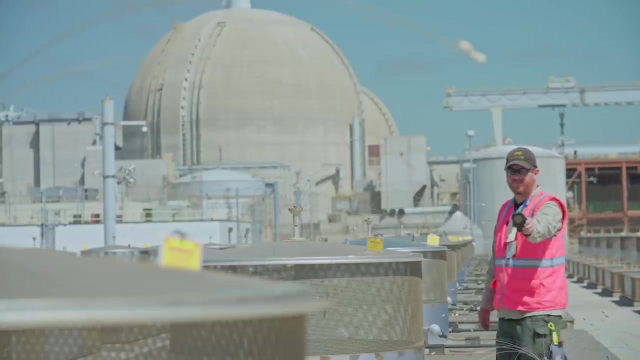 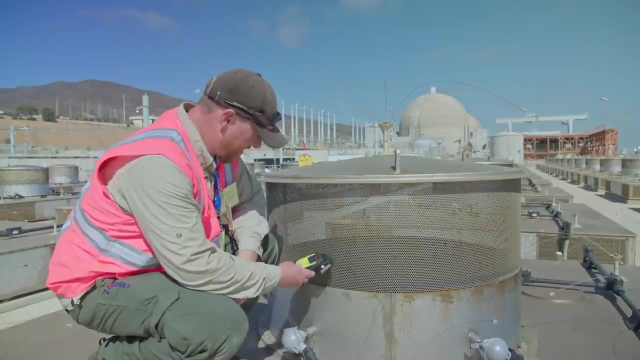 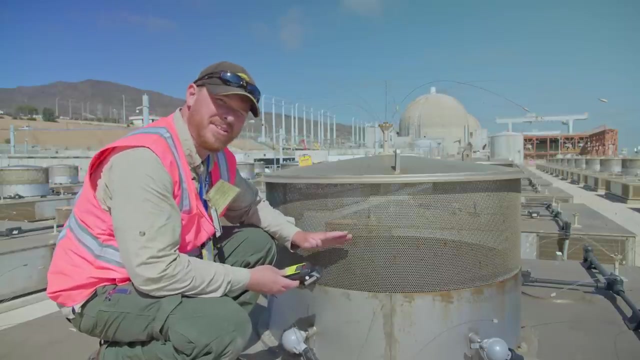 the fuel assemblies are six feet below me. I did see the readings shoot past 500 counts per minute, but that is also extremely low. this is the highest reading I got while checking out the dry fuel storage in this area. us drive fuel actually produces a decent amount of heat coming out of here. it's around 120 degrees. 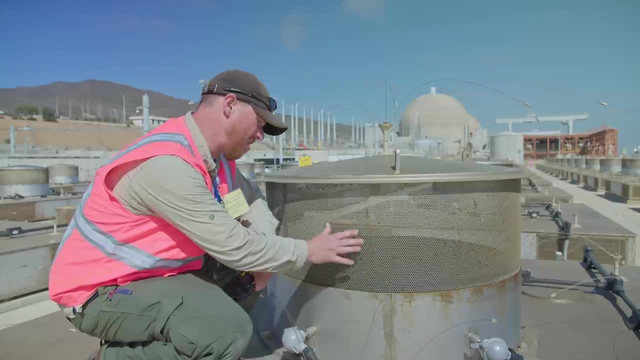 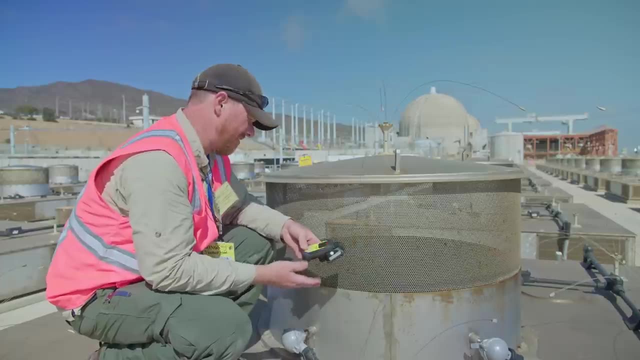 Fahrenheit, the air coming out of here, so it feels pretty warm when you put your hand up in here, when it actually the air comes and is pushed out of here and it feels pretty warm. so I'm going to set it at a out. but it's not the air that's radioactive that's coming out of here. the air is completely. 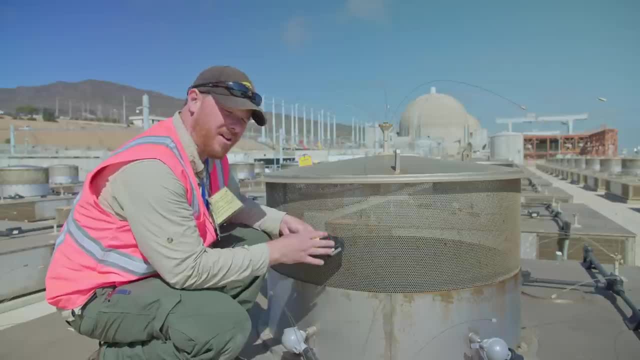 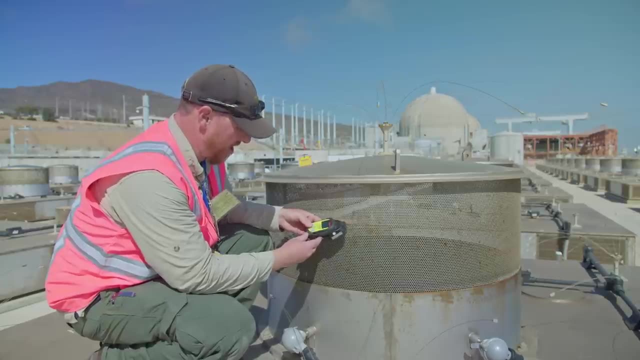 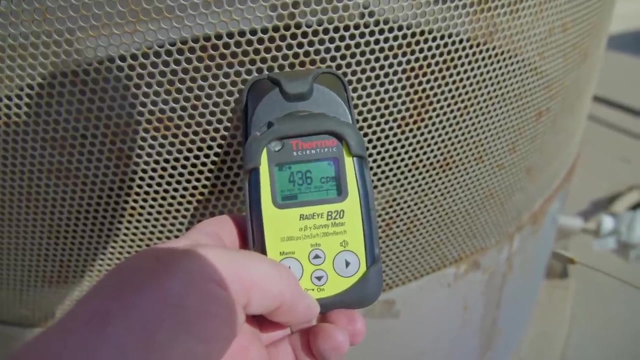 uncontaminated. it's actually the radiation i'm picking up on is from the fuel in the dry storage down here, and so i'm getting around like 350 counts per minute. i've seen it go as high as 400 and still that is extremely low and, uh, that's pretty reassuring that this storage system can. 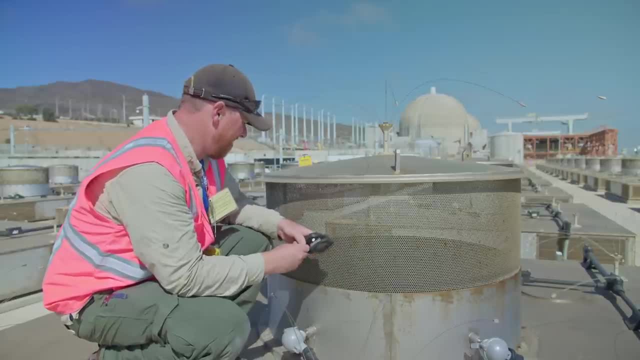 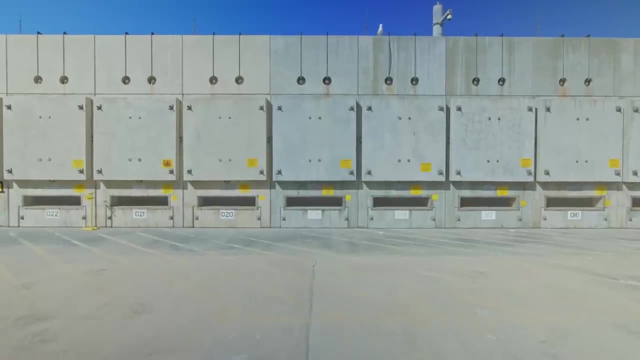 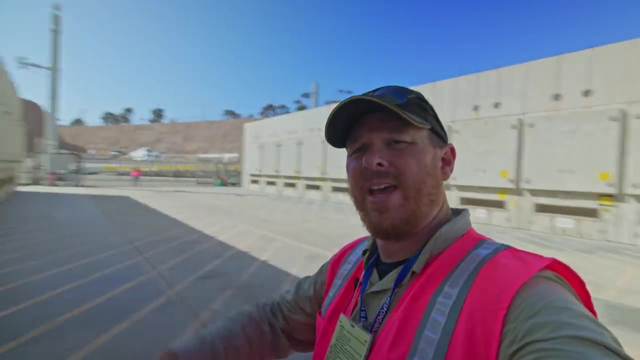 actually keep this radiation under control like this, because, uh, i find stuff way hotter than this. not at a nuclear facility, all right. so this is the other dry fuel storage that's out here. these are from units one, two and three, but it's of an older design of dry fuel storage, and so 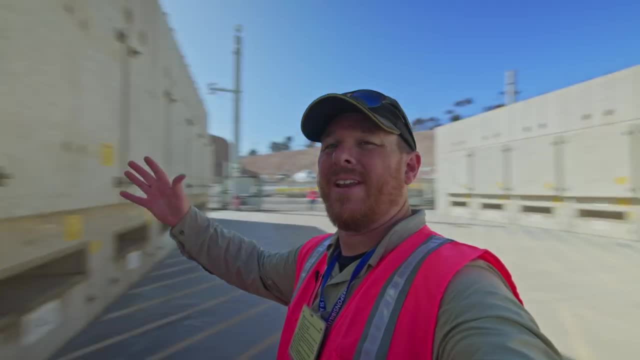 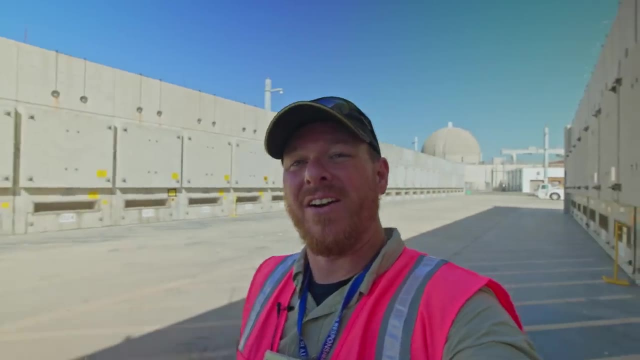 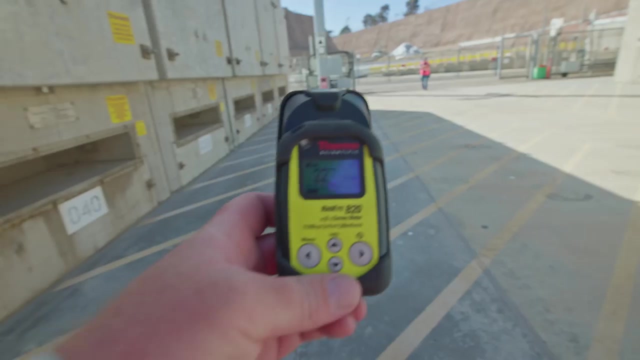 these are really cool. they're like super, super big. i mean you can't tell this is a giant and uh, yeah, they are a little, uh radioactive right here, like down here by these vents right here, and i'll show you that reading here in just a second. 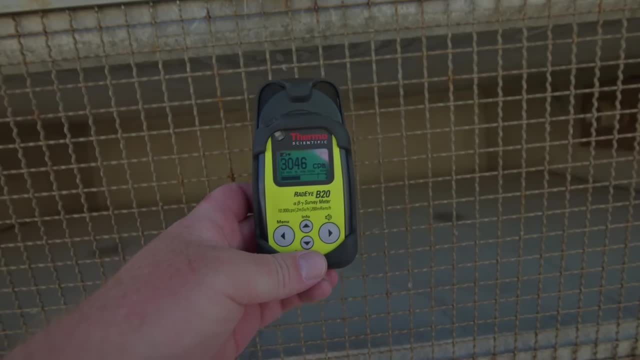 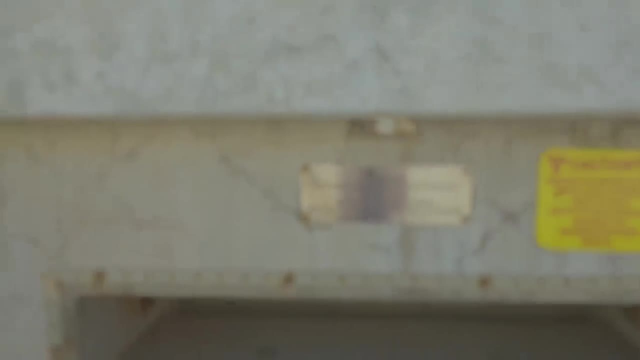 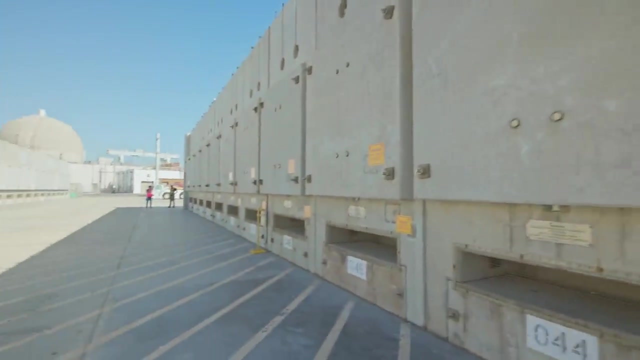 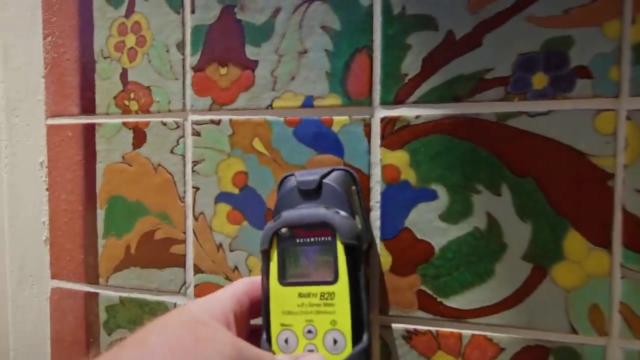 now this may sound like a high level of radiation for the clicks coming off the geiger counter, but this is about a hundred times above background radiation that's being detected out of this vent. but now let's get a little perspective, like we have before. this again is the adams house in malibu, california, and here on this tile i'm getting. 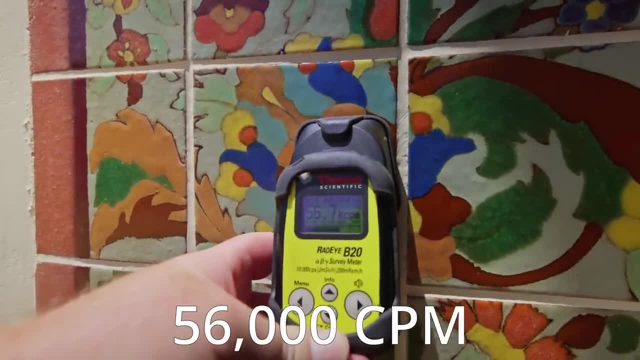 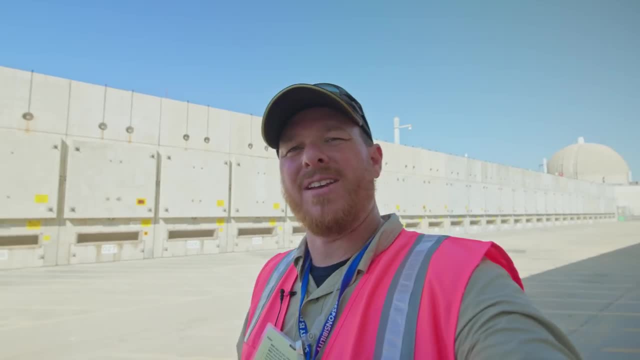 a level that is 17 times above what i was seeing at that san onofre fuel storage. like i keep saying, you know, throughout this video, i can find stuff at uh antique shops that are more radioactive than the stuff i'm finding here, granted a lot of the radiation that's coming. 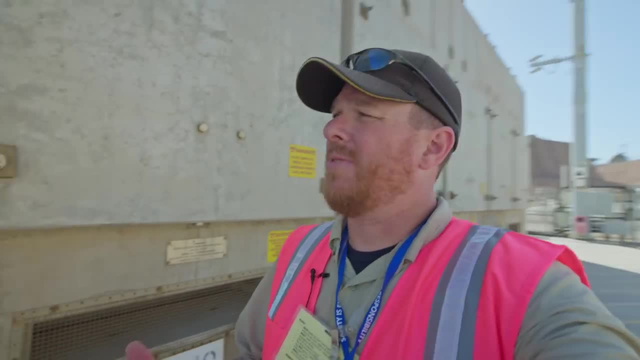 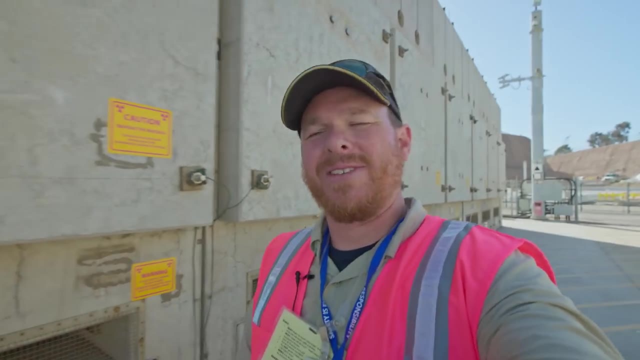 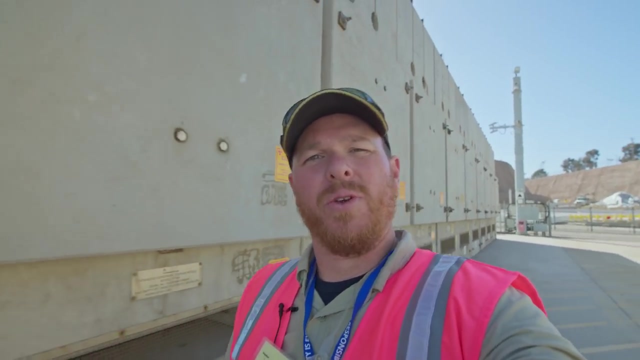 out of this is gamma radiation, which is more penetrating, but i'm not getting anything out of this area. i'm only getting it down by the vent, and so that makes it kind of interesting, like how the radiation exposure works at a place like this and right next to old fuel in dry storage. 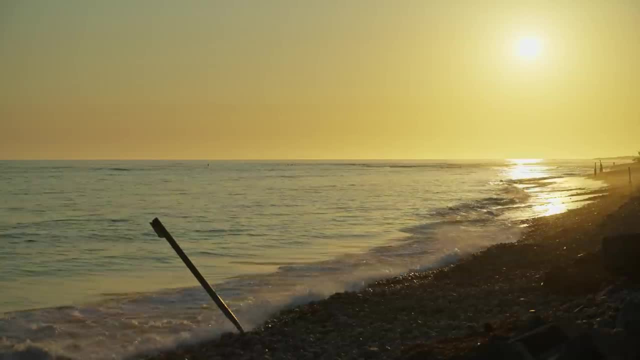 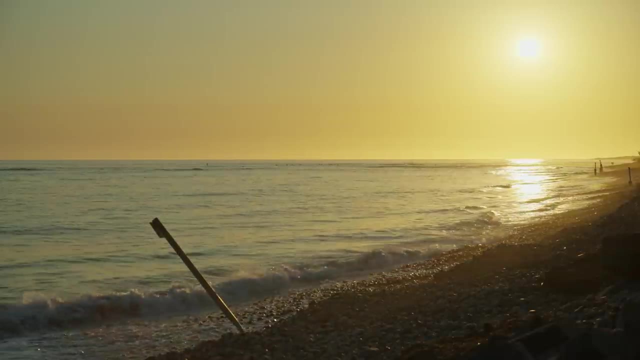 i hope you enjoyed this video about san onofre nuclear generating station and the decommissioning process that's going on there. this is a very interesting video to make, as this was a subject that i've always wanted to know more about, and to actually see this firsthand is quite 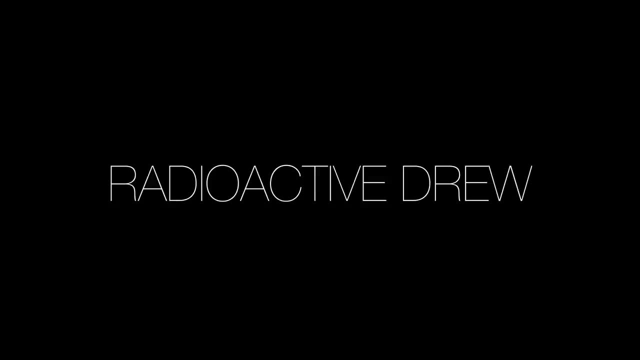 an experience. so if you enjoyed this video, like it, subscribe and i'll see you in the next one. you